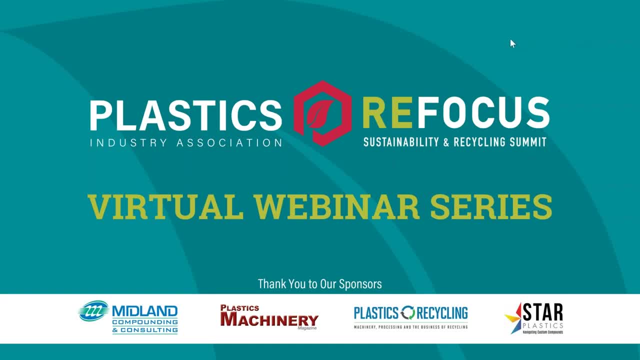 Good morning everyone and welcome to the 2020 Refocus webinar series. My name is Ashley Hood-Morley. I'm the Senior Director of Sustainability and Materials here at the Plastics Industry Association. My role here includes serving as our staff liaison for the Recycling Committee. 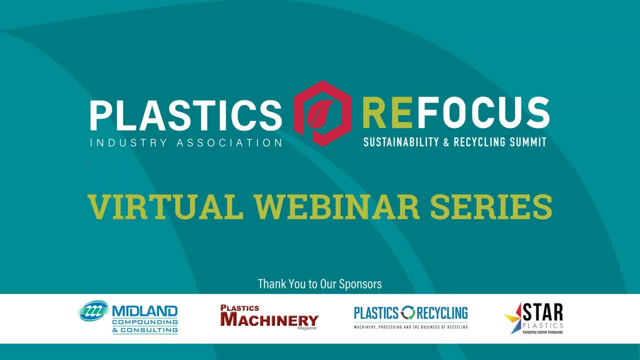 which, through the leadership of the Events and Education Subcommittee, hosts our annual event, the Refocus Sustainability and Recycling Summit. For those of you who joined us here on Episode 1 live stream, you heard me express my disappointment that we could not be together. 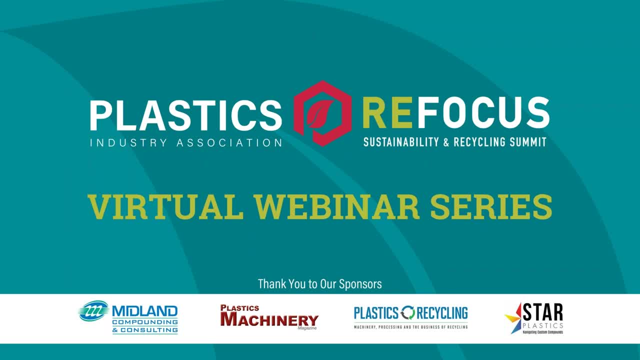 to meet in person this year in May, But kind of what we're doing right now- making lemonade out of the lemons that we've been given. we are excited to be here And to bring you this webinar series that's going to continue to happen monthly throughout. 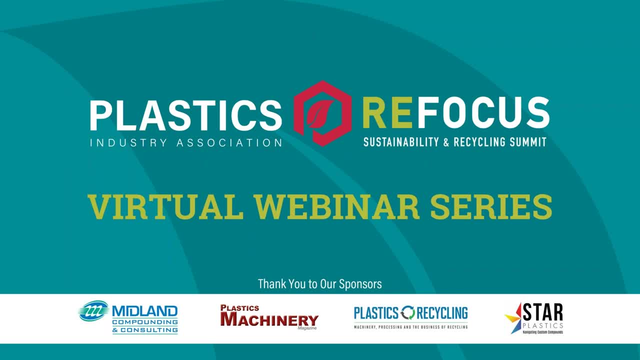 the remainder of 2020.. Today, I'm going to be hosting this program as well as serving as your moderator. I do want to thank Monica Siliol from PolyQuest for preparing to serve as moderator and, unfortunately, unavoidable conflict for her today. so you guys are stuck. 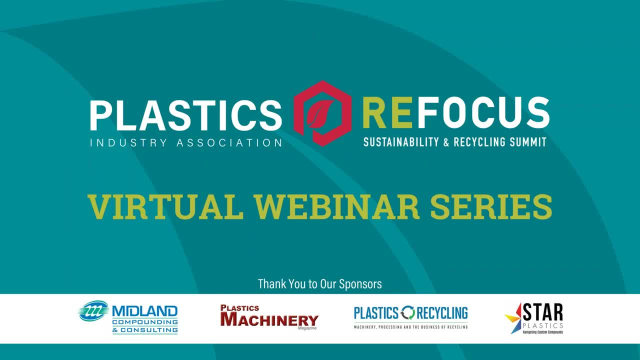 with me, But Monica is a great member of our Recycling Committee. She's the Executive Board and our Events and Education Subcommittee, So I know she's disappointed that she can't be here with me as well, So just wanted to give her credit. 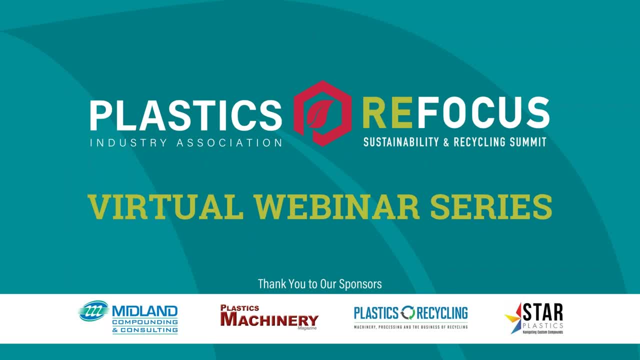 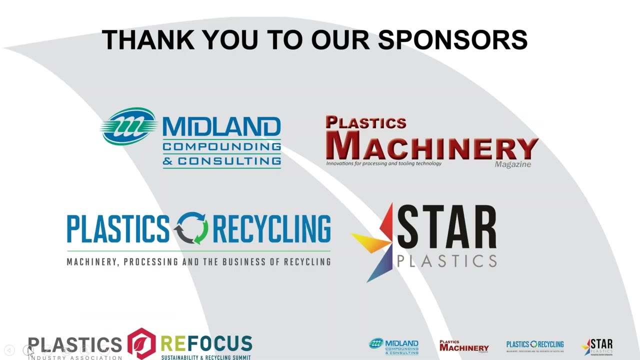 So today we're going to learn all about LCA. So before we dive into that topic, let me just bear with me to cover some background and housekeeping items before I turn it over to our speakers. So first and foremost, as always, we want to give a sincere thank you to our sponsors. 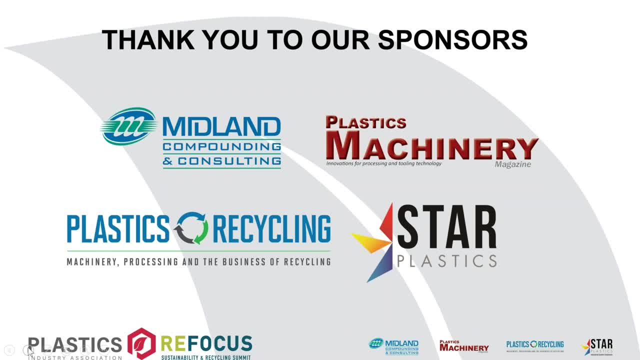 for this webinar series: Midland Compounding and Consulting, Plastics Machinery Magazine, Plastics Recycling Magazine and Star Plastics. Give these folks a virtual round of applause. I know they can't hear you, But thank them for bringing this excellent content to you. 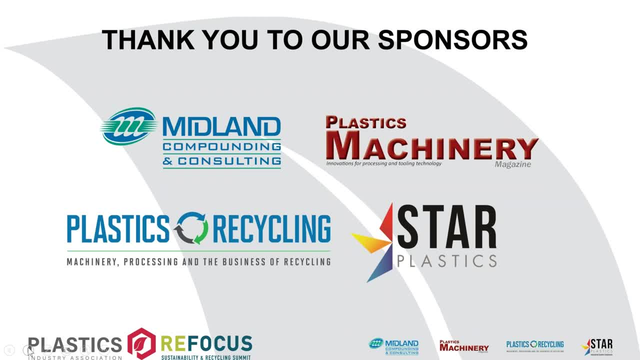 today and for the remainder of the year, At the low, low price that I think we've been talking about. I think you're all willing to pay. meaning, because of these companies, you're able to view this webinar at no charge And based on the number of folks that we have. 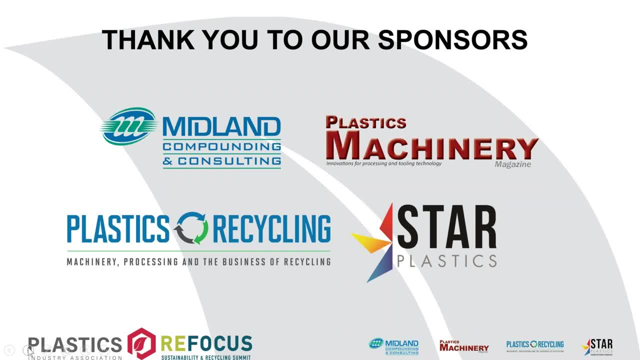 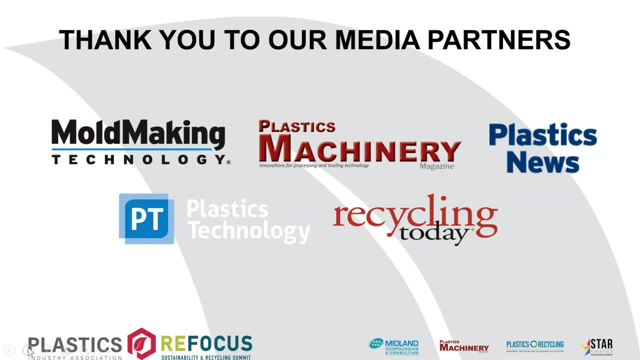 tuning in today. there's a loud, loud, boisterous round of applause going on right now, So thank you to our sponsors. In addition to our sponsors, thank you to our media partners, which include Mold Making Technology, Plastics Machinery Magazine, Plastics News, Plastic Technology and Recycling Today. 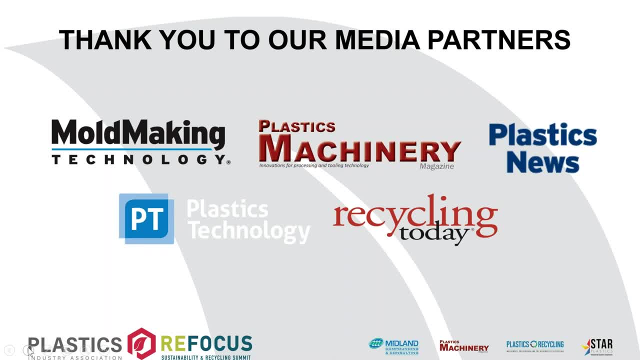 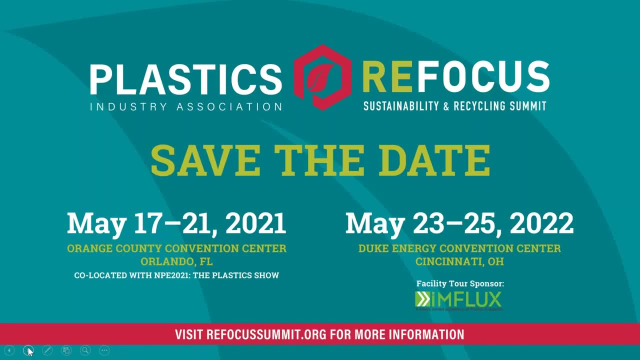 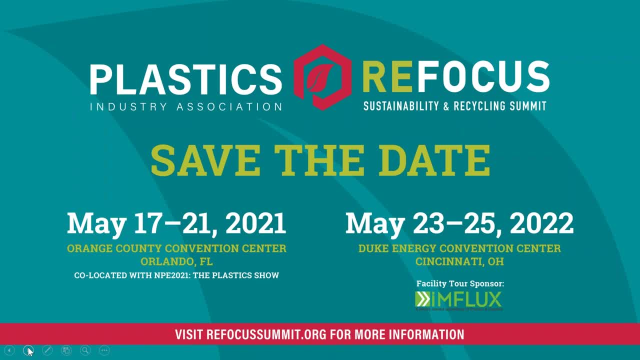 refocus event at, in conjunction with MPE 2021, the Plastic Show. That's going to happen the week of May 17.. And we're targeting May 19 for a refocus sustainability and recycling event. information will be coming out, you know, in the coming months about that And also just as a 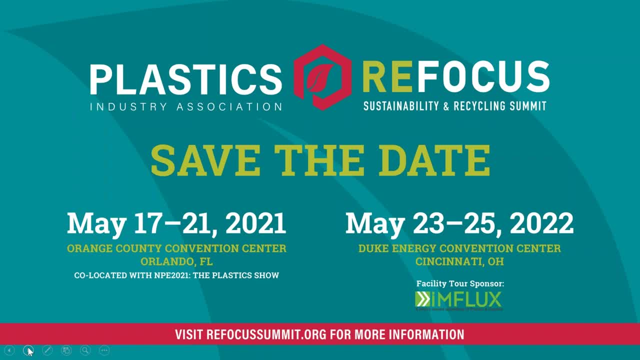 reminder to go ahead and plug dates in on your calendar. Although we were not able to host our event in Cincinnati this year, we are really pleased that we've been able to secure that date and location for 2022. So we've shifted many of our planned events there, including Influx has. 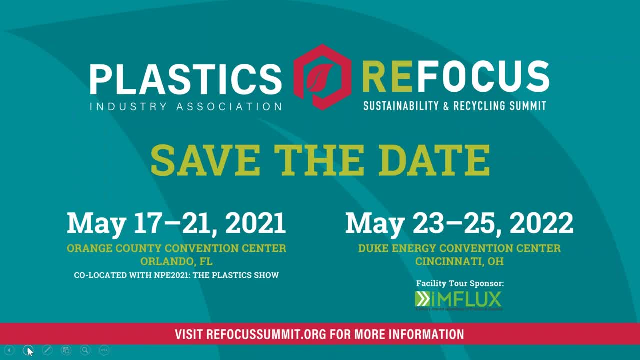 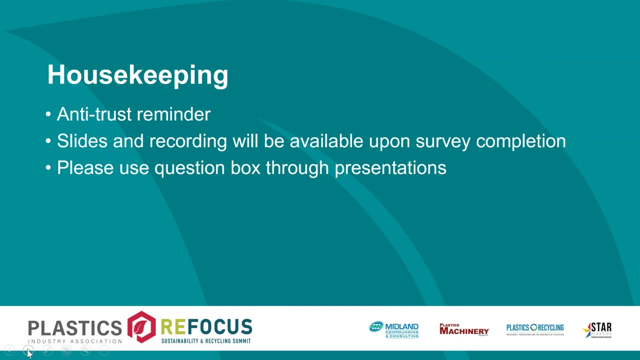 graciously agreed to continue to sponsor our facility tour in 2022. So we already have some really good things lined up for you there. Okay, And then just getting into, finally, just a few housekeeping things before we dive in, Although all of the attendee lines are currently muted. 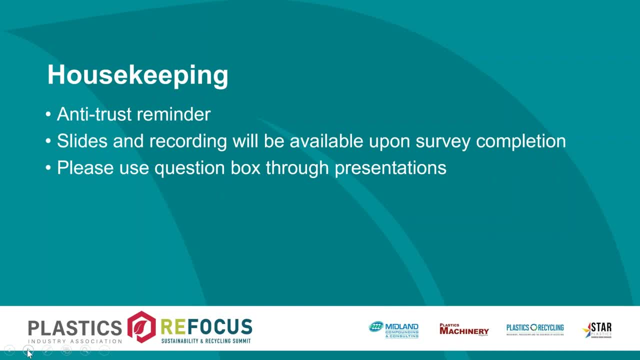 we're certainly going to offer a Q&A session. So, the way that we'll go through this, I'll introduce Both of our speakers for today. both of them will present During those presentations, if you would. if you think of a question that you'd like to ask, please submit that via the question box. 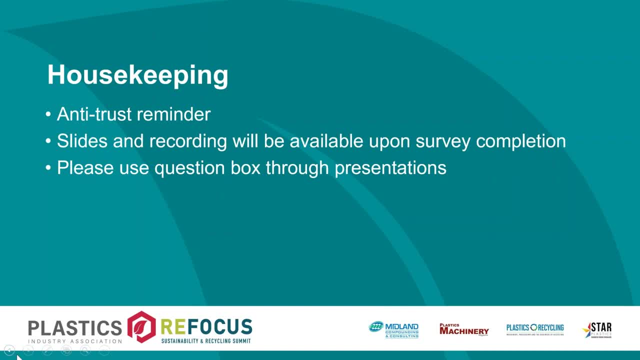 as part of that GoToWebinar panel that you have control of, Submit those questions And after both Bruce and Dennis speak today, we'll do a Q&A session all together with this at the end. So keep in mind during this time: 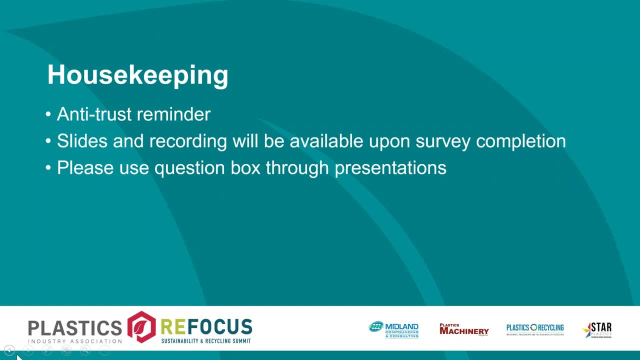 and we'll see you at the end of the session. So keep in mind during this time- and we'll see you at the- because Dunno, Only public medical care detectives personally When you're posing questions- that we will about antitrust rules and refrain from. 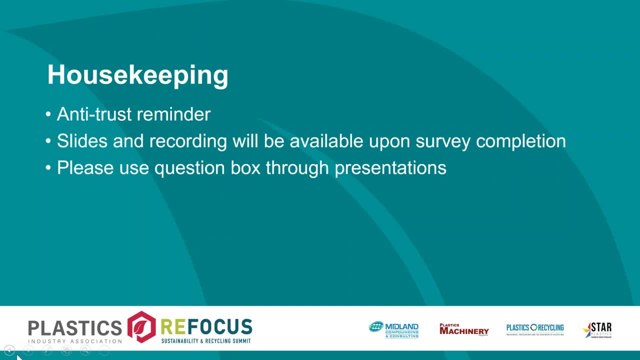 discussing processing, production, marketing strategies, anything that could be construed as market manipulation. we will not not address questions of this nature during the meeting. Lastly, I'd like to notify all attendees that this is a public education session where members and non members and crest may be president. 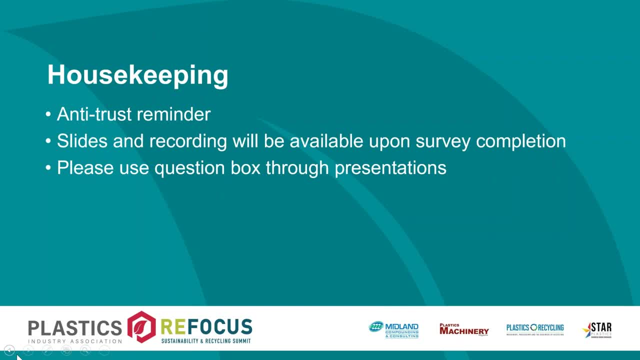 We will not be conducting Any official business And the association to today and this session is being recorded and slides will be made available after this is concluded today. So to access the recording and slides, we'll be sending all registrants a quick. 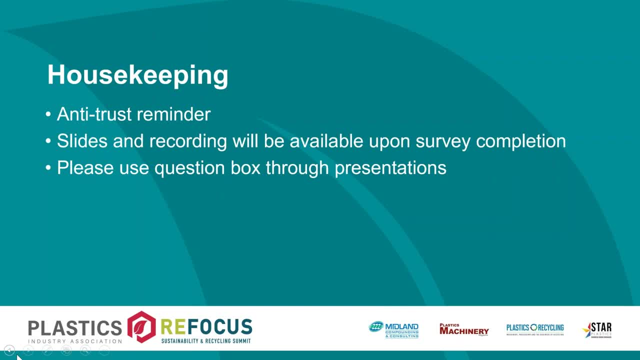 survey via email once this wraps up. When that goes out, if you'll just take three to five minutes to answer some brief questions, at the end of that you'll be presented with a link so that you can re-access this information as you wish. 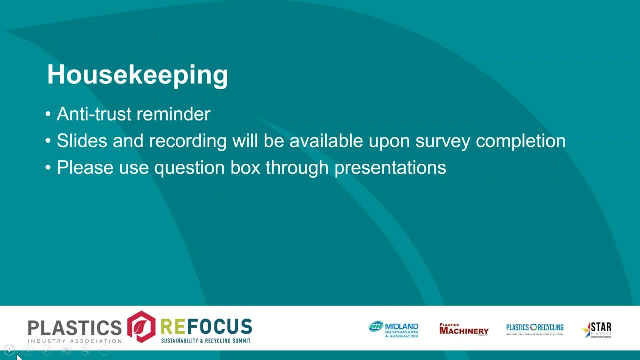 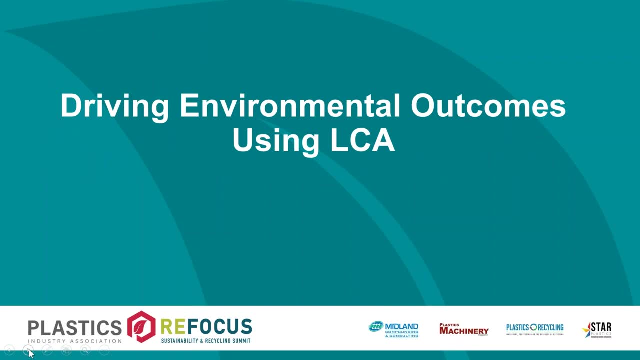 Okay, and I think with that we have completed all of our housekeeping. So now I would like to get us started on our topic. today, Again, we are going to be covering driving environmental outcomes using LCAs. So today we have two speakers with us. We have 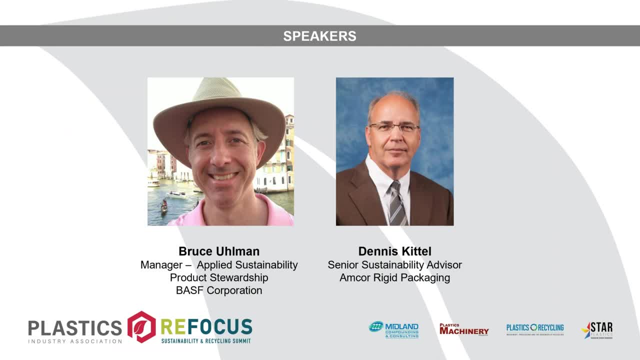 Bruce Ullman and Dennis Kittle from BASF and AMCOR respectively. So first I'd like to introduce both of our speakers before we dive in. So Bruce has been working in the fields of engineering, manufacturing, research and development and sustainability for over 30 years. 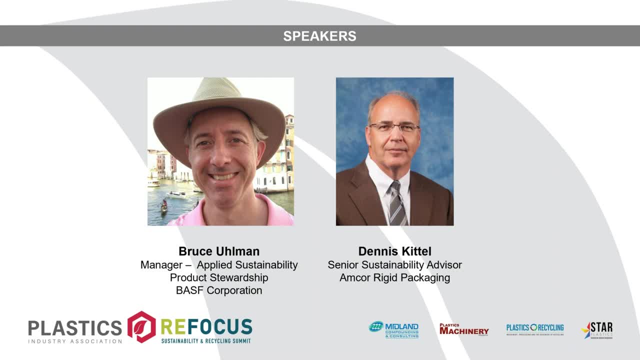 Bruce has several years of international work experience, with specific expertise in the areas of process and project engineering, technology, commercialization and lifecycle assessment. More recently, he's worked in the areas of applied sustainability and has performed lifecycle and eco-efficiency analyses and total cost of ownership studies for a broad range. 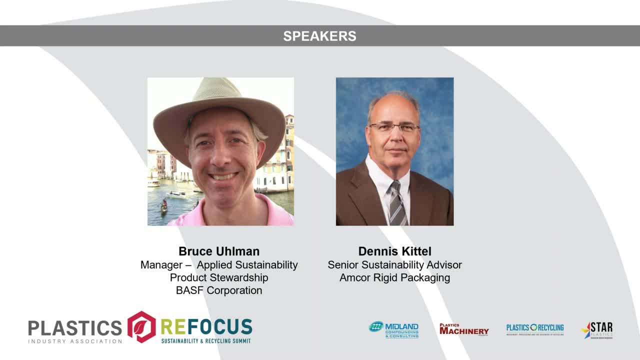 of end consumer products and industrial processes. Bruce partners with BASF many businesses and customers in helping them understand and measure sustainability throughout their value chain and helps them integrate the results of sustainability studies into their strategic decision-making processes and stakeholder communication. He speaks frequently on sustainability and lifecycle assessment and has published 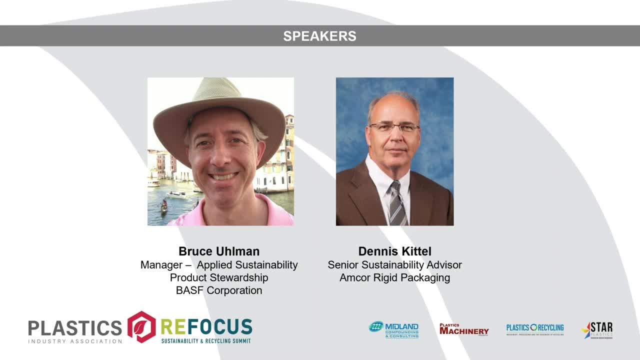 many articles on these topics. Bruce has a BS in chemical engineering from Villanova University, is a member of the American Center for Lifecycle Assessment and is a certified LCA practitioner and certified lifecycle executive. He's also a member of the International Society of 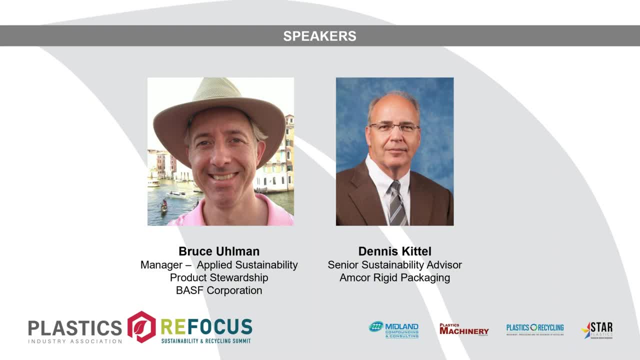 Sustainability Professionals and is a certified sustainability associate. Bruce lives in Northern New Jersey with his wife and two children. Our second speaker, Dennis Kittle, joined AMCOR in 1991 in research and development and has over 35 years total experience in plastic. 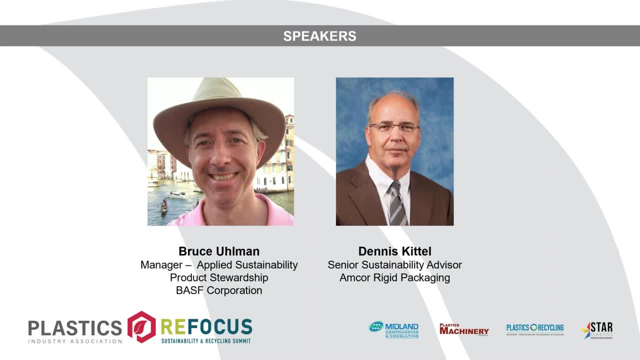 packaging for food applications. Since that time, Dennis has served as the director of cellular manufacturing and R&D technical director for food packaging in both flexible and rigid formats. Over the past few years, Dennis has held the position of global sustainability manager for AMCOR's rigid packaging business group and is currently senior advisor to the sustainability 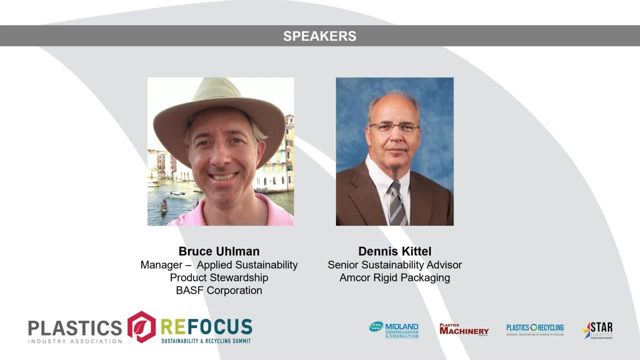 efforts of AMCOR. He's closely worked with Dennis Kittle on the sustainability and lifecycle assessment of food packaging. He has worked with customers, commercial, marketing and technical functions to define and implement more sustainable packaging. Food packaging piques Dennis' interest and it has. 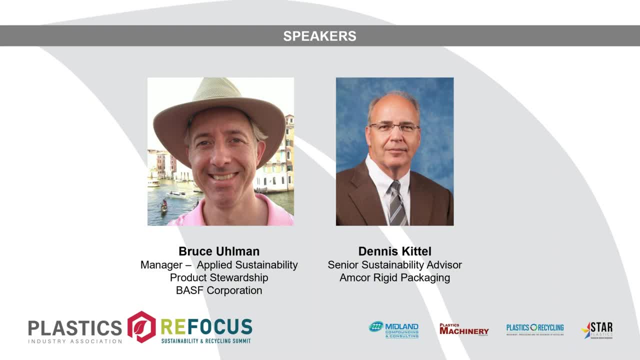 a challenge to be recyclable with many multi-layer structures. Before joining AMCOR, Dennis worked with Ostermeyer Division of Craft Foods. He holds a BS in mechanical engineering and an MS in masters- I'm sorry- manufacturing systems engineering from the University of Wisconsin-Madison. 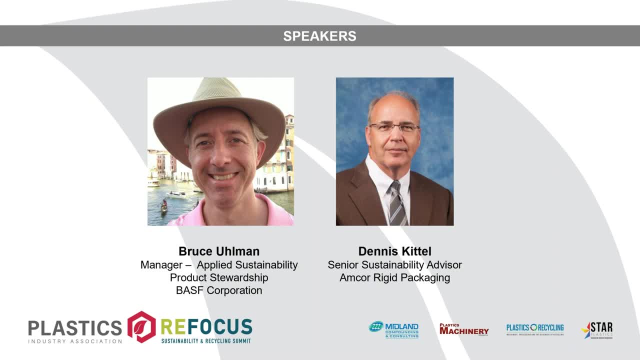 So, as you can see, both of our speakers today that have graciously agreed to be with us have a tremendous amount of knowledge in this space, So I'm happy that they accepted our invitation to be here with us today. I'm as 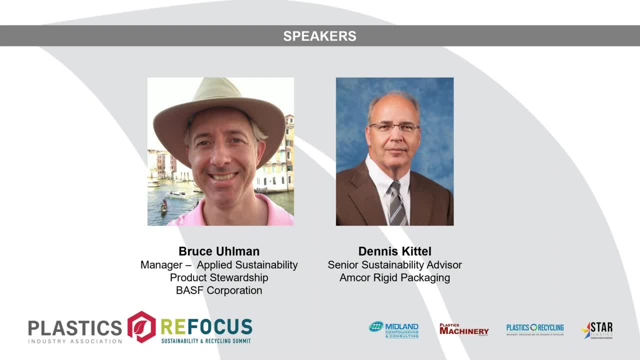 excited as you are to sit back and learn. I have a lot of learning to do in the lifecycle assessment space myself and I've seen their slides and I think you guys are in for for a treat. So with that I am going to advance to. 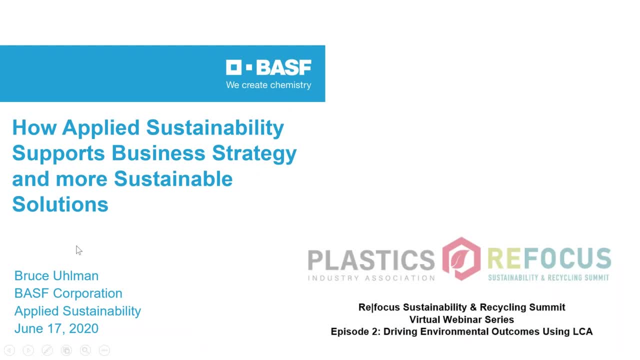 Bruce's slides. I'm going to exit the webcam and sit back and enjoy this with you guys and Bruce. I am going to leave you guys and I'm going to turn the mouse over to you, So you should now have that and be. 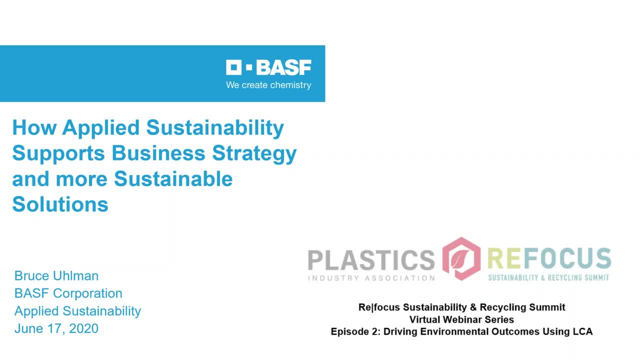 able to take it away and just don't forget to unmute yourself. Okay, great, Can you hear me, Ashley? You are good to go. Thanks, Bruce, All right, yeah, So thank you for the nice introduction. It's a pleasure to be here with you and Dennis and the audience. 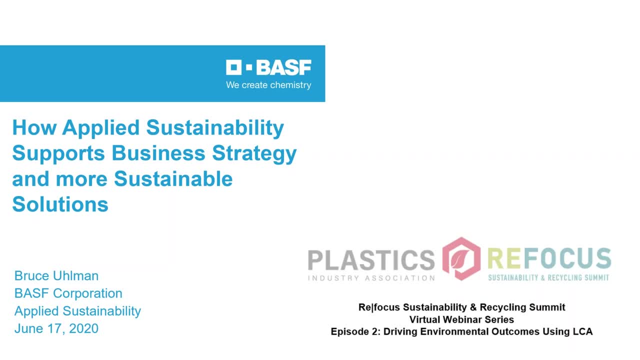 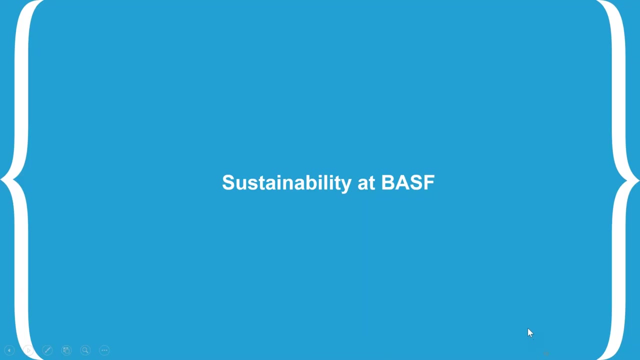 Here to talk about lifecycle assessment and how it really benefits our businesses but overall our customers and society. My talk today is going to be around applied sustainability really- how we're applying lifecycle assessment really to support business strategy and driving more sustainable solutions out there into the marketplace. I went one too many Missed the introduction there. 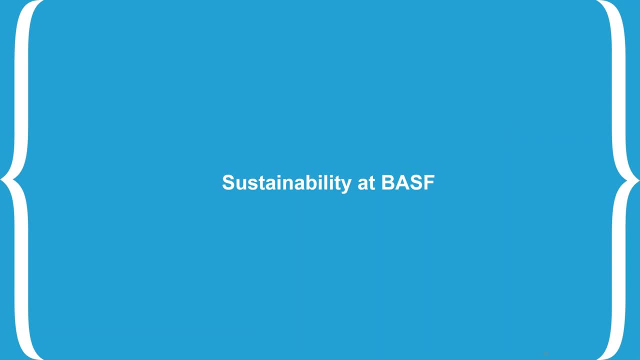 So I'll just go over the agenda for today. I'm going to provide a brief overview of BASF and what sustainability means for us, and then talk about the challenge of sustainability, The challenge that we face for better understanding it, measuring it and really. 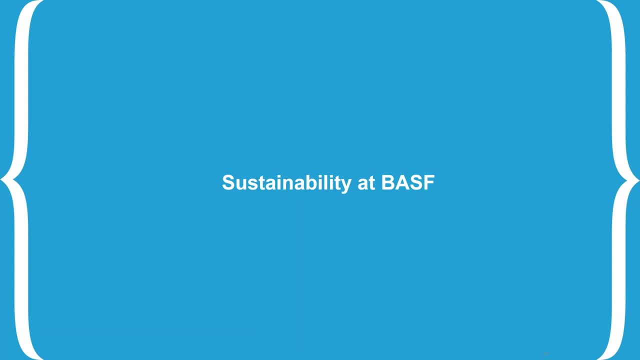 integrating that into our decision-making process. I'll then give a brief overview of LCA. It helps to have a good fundamental knowledge of what this methodology is all about, and then I'll give some case study examples of how BASF is using our applied sustainability toolbox. 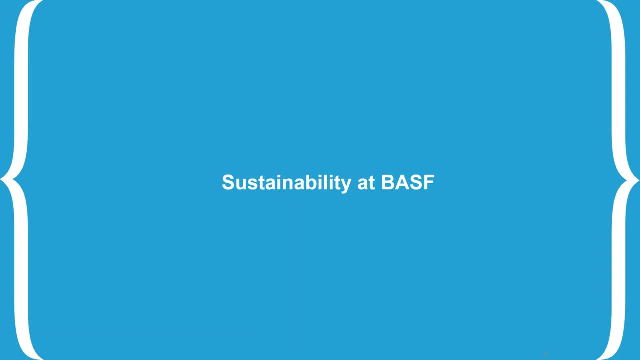 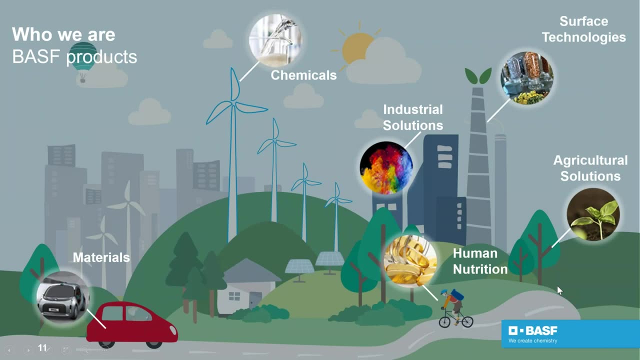 to help us manage sustainability within our value chain, support our customers' needs and create value to society. So for BASF, we are the world's largest and leading chemical company. We produce over 50,000 solutions and with these solutions- solutions- we are impacting mostly everybody. on this call, We touch everybody And because of this, 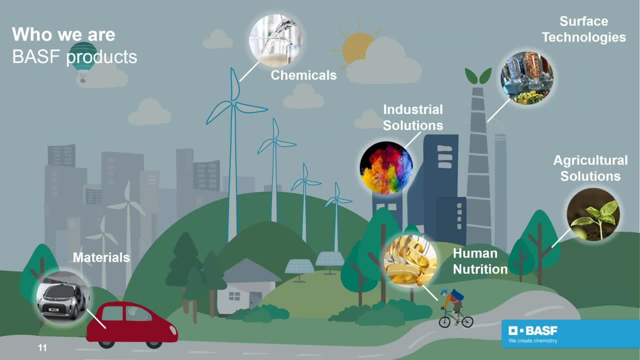 impact that we have on society. we take our role in driving sustainability quite seriously. We want to, as BASF, really have a positive impact on society, not only now but also into the future, And we do this really by creating chemistry for a sustainable future, And we're using science and 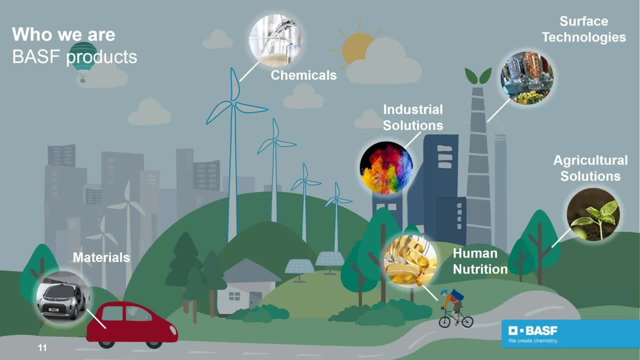 innovation, really supported by lifecycle thinking and lifecycle assessments, to really enable our customers to meet the needs and challenges of their market sector, but also society as a whole. And we really summarize this commitment to sustainability in our purpose, which is that we create chemistry for a sustainable future. 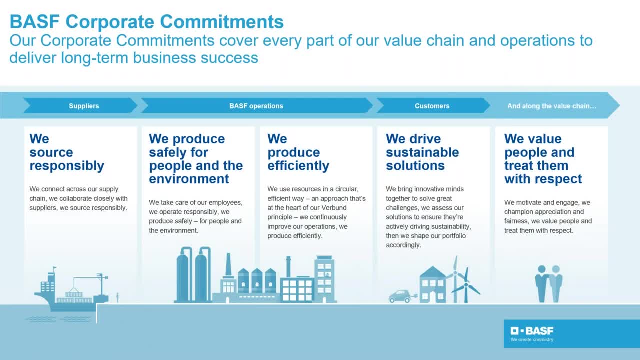 And how do we do that? Well, we do that with our corporate commitments. We source responsibility. We're a global business and we have responsibility not only for our own actions, but the actions of our suppliers. So we want to make sure that our suppliers are sourcing materials. 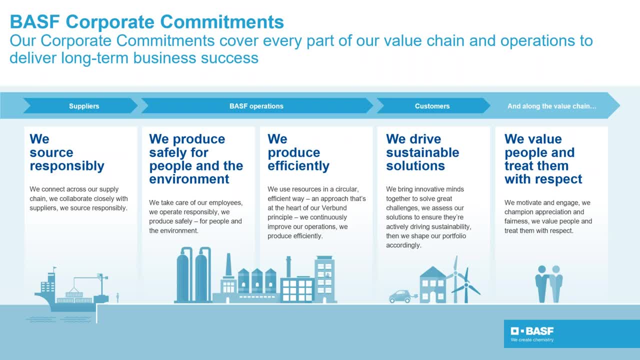 using the highest levels of sustainability and practices that are available. We contribute to organizations like Together for Sustainability and the Roundtable for Sustainable Palm Oil, supporting these sourcing opportunities For us. safety is the number one priority For us, producing safely for our employees, for the people who use our products, but also for the environment. 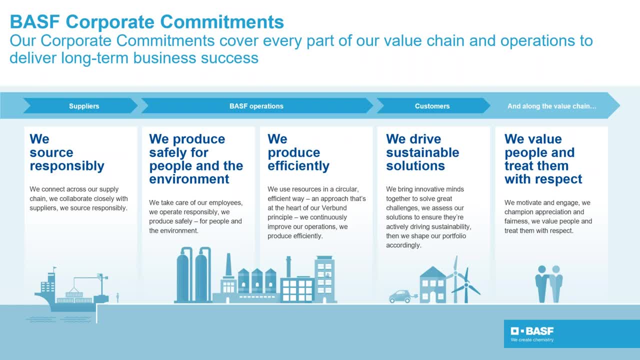 And we also produce efficiently as well. Operational excellence and producing efficiently is a key to our growth and really driving sustainability. We achieve this through our Fibunda manufacturing, but also through our concerted sustainability goals. We have committed this year to keeping our greenhouse gas emissions flat at today's level. 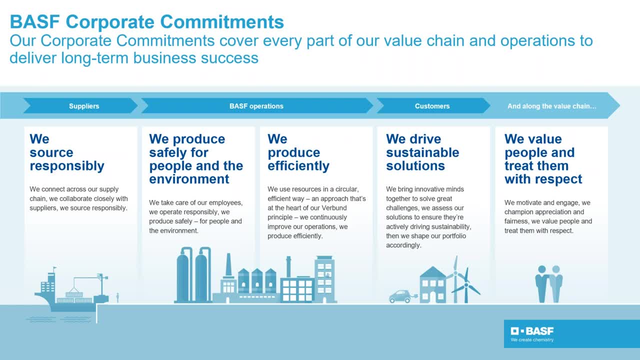 Through 2030.. Thus we are decoupling our organic growth from our greenhouse gas emissions and thus we're really going to set an aggressive target of growing carbon neutrally. We drive sustainable solutions. This is really focused on those solutions that we have are called accelerator solutions that are really adding great sustainability benefit to our value chain. 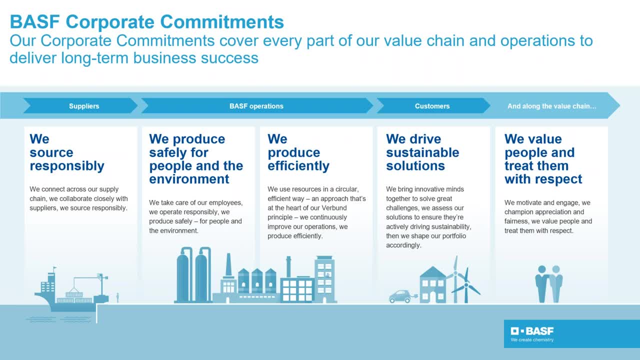 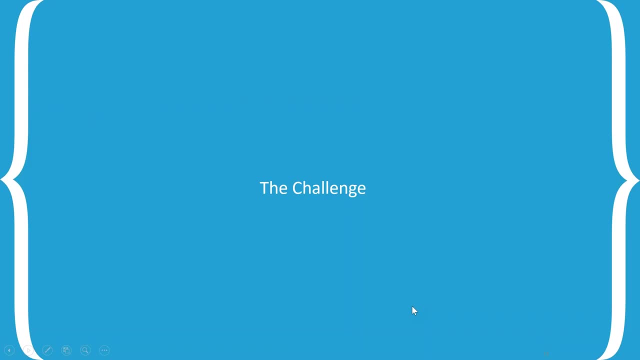 And, of course, on the social side, human rights. We respect human rights. It's the pillar of our social responsibility. We value diversity in the workforce in our supply chain and really know that that's helping us drive sustainability within our own operations but also within our supply and value chain. 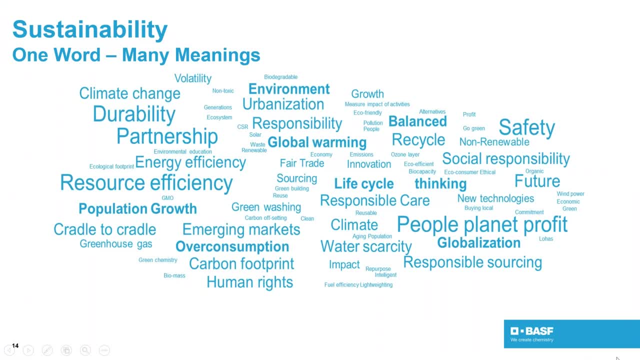 But the challenge that we have- and I think, if we all look at this word chart right here, word cloud- that we can all associate many different meanings to sustainability And that's what makes it so difficult for us to integrate within our businesses, within our customer engagements, and really for us to quantify. 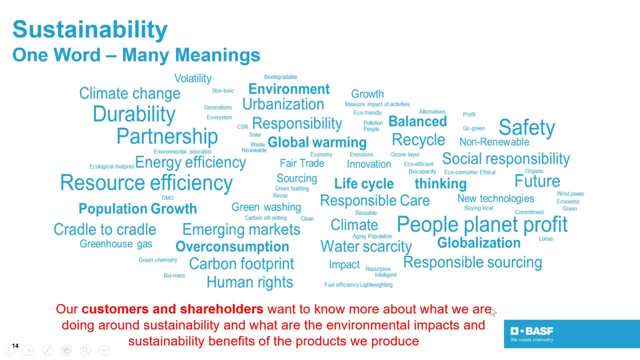 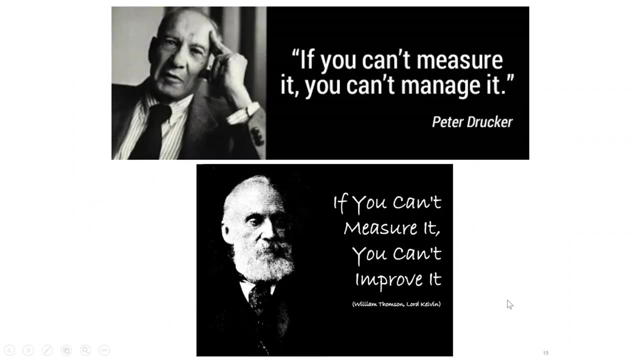 So, with that, we know that our customers are very anxious to know what we are doing around sustainability. How are we supporting them with driving sustainability within their value chains and helping to reduce their environmental impacts? Well, we took to heart these two great quotes here from business strategist Peter Drucker. 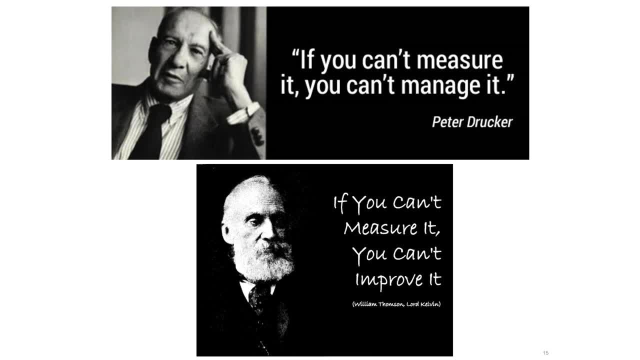 He said: you can't measure what you can't manage, and if you can't measure it, you can't improve it. So with that, BASF knew that the key to sustainability is really around measurement. That's the key and lifecycle assessment is that key tool for us. 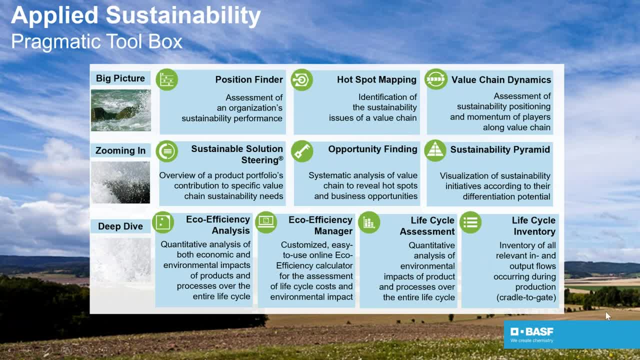 So with that we developed over the last several years a robust toolbox that really enables us to better understand and manage sustainability at various levels of granularity, whether it's looking at the big picture or the small picture, or the big picture or the big picture. 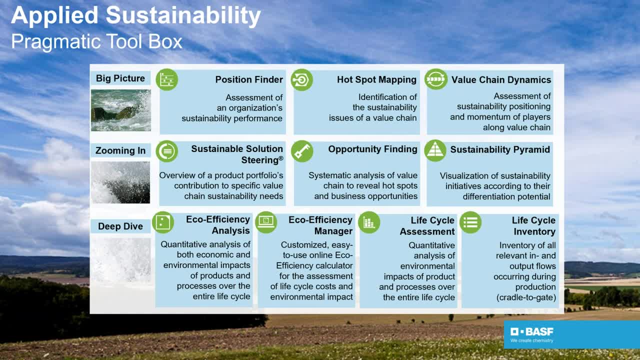 Such as hotspot analysis or assessing your own operations around sustainability with position finder. But it allows us also to do those deep dives through lifecycle assessment tools such as the eco efficiency analysis or traditional LCA. That's really enabling us to address that challenge of quantifying sustainability in really real science-based, pragmatic terms. that enables us to really integrate that into our business decision making. 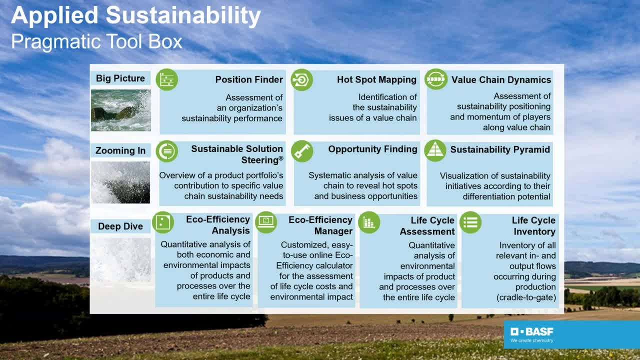 It enables us to understand sustainability trends in the marketplace- where are the hotspots- and thus enables us to understand where our benefits are and to communicate those, but also understand where tradeoffs are and making sure that we're not optimizing in one area at the expense of another area. 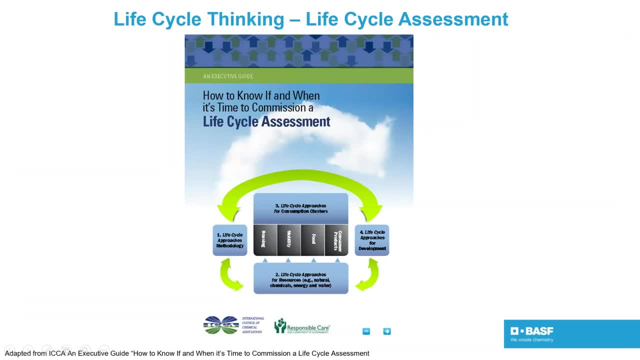 So what is lifecycle assessment? For these next few slides here I pulled information from a very recent study. It's from a very useful guide from the ICCA, the International Council for Chemical Companies, which published a very useful executive guide to basically understand lifecycle assessment, when to use it and what it is. 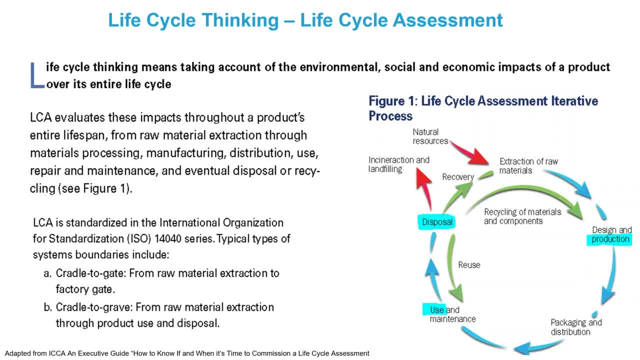 So what is LCA? Well, from the very highest level, it's about lifecycle thinking. It's a systematic and holistic approach that takes into consideration all three pillars of sustainability: The environmental pillar. the environmental pillar and the environmental policy, The social pillar. social pillar as well as the business case, the economics. 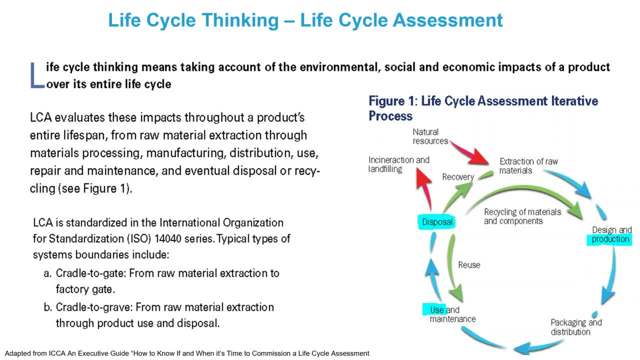 You can see here from figure one that lifecycle thinking and lifecycle assessment really covers all stages of a product's lifecycle, starting from the inception of the extraction of those basic raw materials out of the earth and following it through the various stages of production leading to the production of that final consumer product. 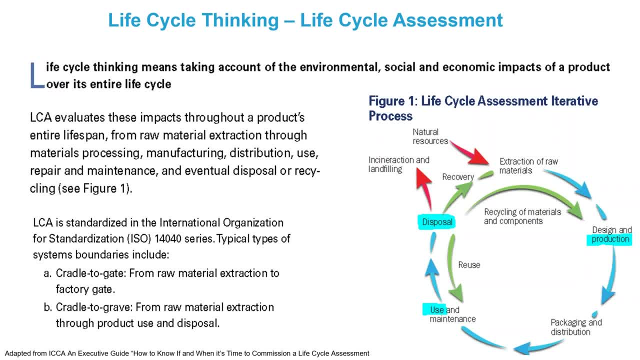 We assess the use of that product and its performance attributes, But also its end of life. what's happening in the disposal phase? Is it being incinerated, landfilled, or is it going back through recovery and recycling? Now, the procedure for conducting a lifecycle assessment, which is really that methodology of integrating lifecycle thinking in a more rigorous manner, is really governed by the ISO standards 14,040 and 44.. 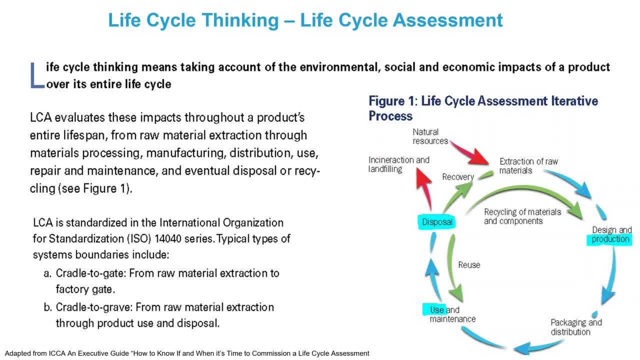 And they provide the framework and the structure for how you can use it. And then you can conduct that study. And again, this study covers the full lifecycle, which would be cradle-to-grave, but then you can also take some segments out of that, say, cradle-to-gate, where you're only looking at a portion of that full lifecycle. 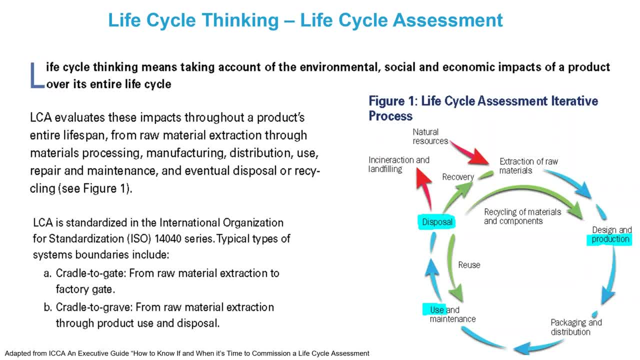 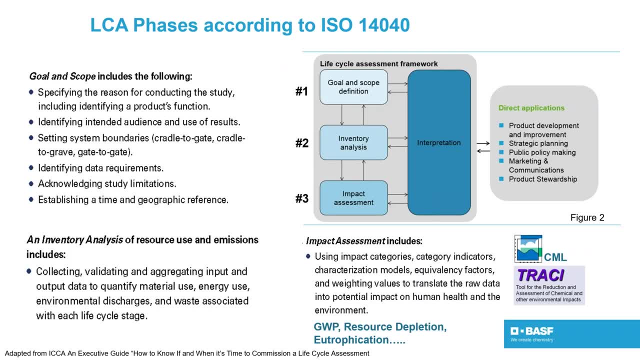 Say cradle-to-gate is really only looking at raw materials, to the factor gate, something that BASF would look at as we produce our raw materials and assess that, delivering that information to our customer. So looking at the guidelines from ISO. So with regards to how you conduct a lifecycle assessment, really from a high level, it's three different steps. 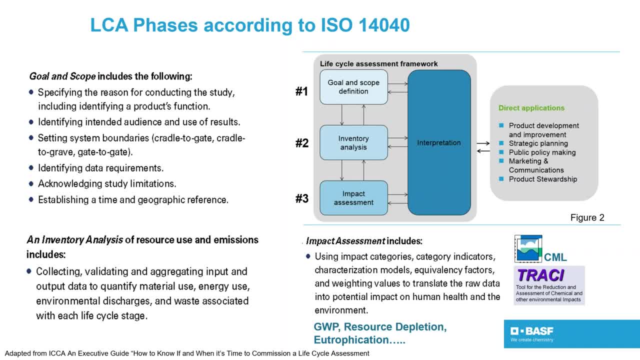 You really have to understand and define the scope of the study. What are you conducting the study for? What do you intend to learn? What is your comparisons going to be of the various alternatives? How broad is the system boundary that you're going to include? 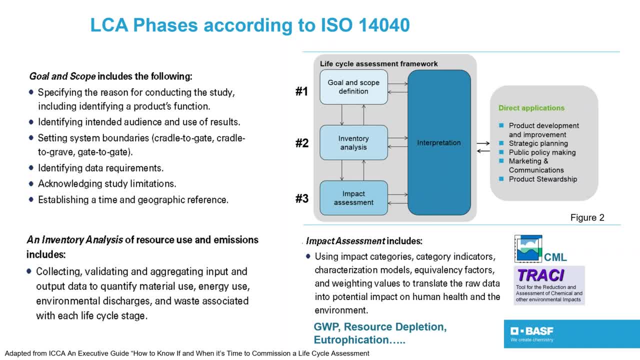 And when you get these results, who do you intend to communicate them to? So these are all important things to identify. You have to do that early on to make sure that you're measuring the right thing and you know who the audience for those results are going to be. 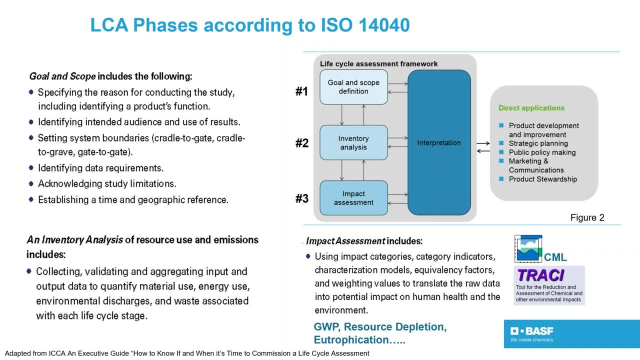 Second step in an LCA is doing that inventory analysis, And this is where you're collecting, confirming and aggregating all these inputs and outputs that are coming from nature. So outputs from nature could be we're extracting basic raw materials or we're using water and energy. 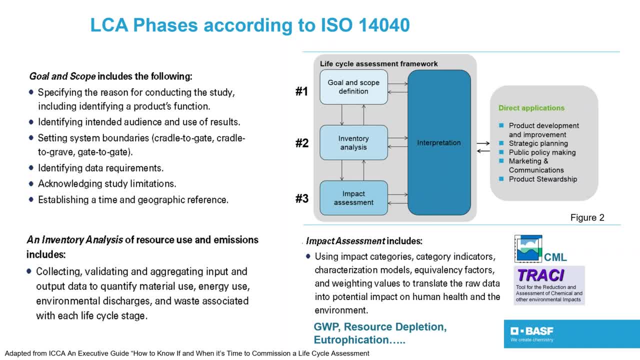 And then we also have to look at the emissions, The discharges, such as solid waste or water emissions. So this is all occurring in that inventory analysis phase. Once you've measured all those inputs and outputs, you can go into the impact assessment phase. 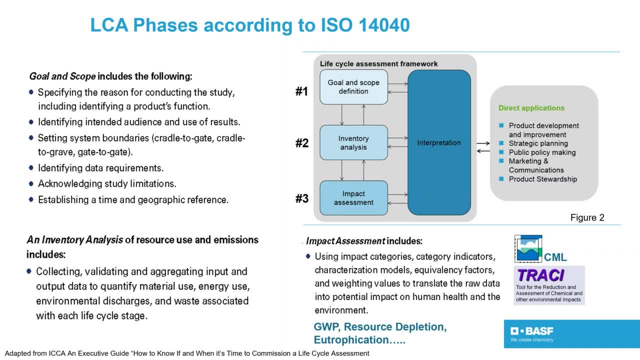 And this is where you characterize these flows through industry standards such as TRACY or CML, And they help you take those flows and assess those potential impacts on our environment. An example would be: you're measuring all the greenhouse gas emissions Over that. you're measuring all the greenhouse gas emissions. 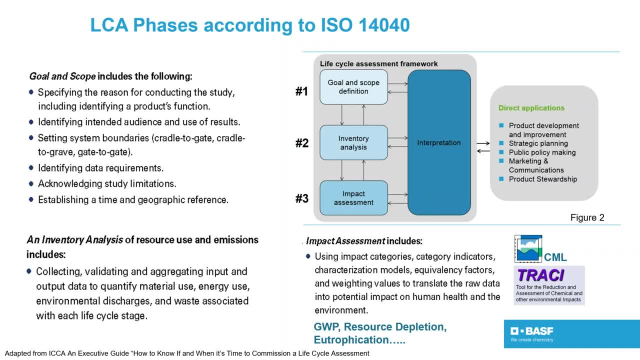 Over that life cycle. you aggregate those together, characterize those and then you can find the potential impact that's having on global warming and climate change. Now, throughout that whole LCA, you're going through these interpretation stages as well, where you're constantly reassessing and reviewing your data and your calculations to make sure that you're still staying true to what you define as the goal and scope of your study. here, 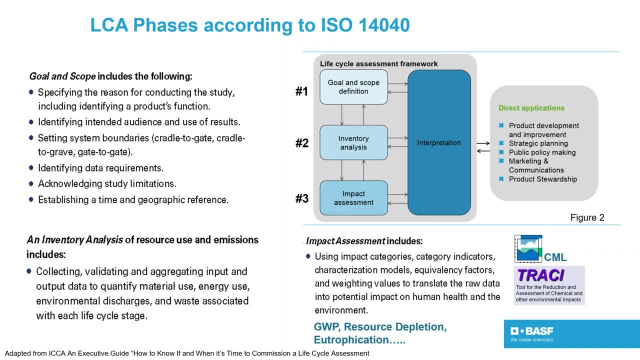 But that you also are understanding and formulating. So you're writing a report at the end where you're assessing this information, communicating what the findings were, any limitations that you may have with the study and ultimately directing that in its use in the business, whether it's in product development, using it in your marketing communications or supporting people within your R&D program or product stewardship. 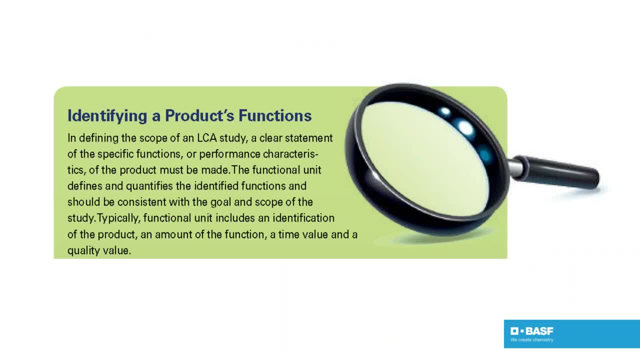 Now, when you start off an LCA, a key aspect is: what is that unit of comparison? You know how do you compare these various alternatives And you do that through the functional unit, or also known as the customer benefit, And this provides you really that measure of unit that you can compare these systems to, as you're combining and referencing these input and output flows. 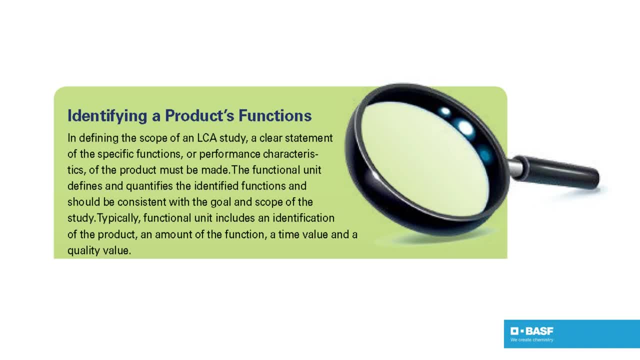 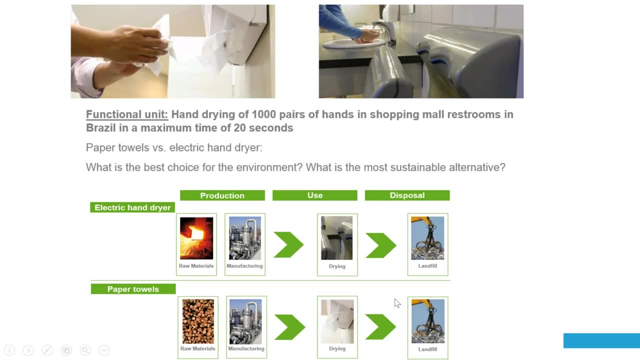 And it really enables you this comparison of really two different systems that perform the same function, And this function must again agree with the goal and scope of your study. Now, an example of this here, of a functional unit To really make it more relatable, is if you had drying of a thousand pair of hands in a shopping mall in Brazil over a time of 20 seconds. you can achieve this function two different ways. 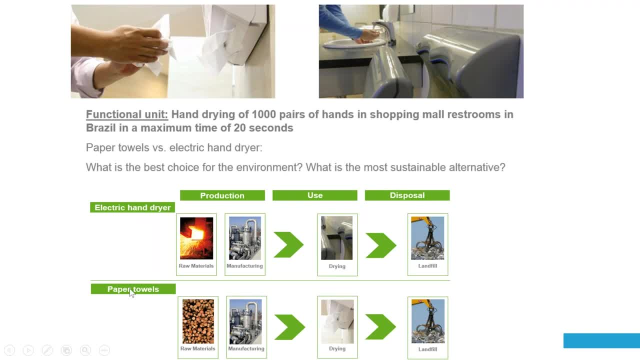 You can use an electric hair dryer or a paper towel, And this really then defines the alternatives, then that you assess their impacts in the production, the use and the disposal phases for that paper towel to achieve that functional unit, And you would do the same thing. 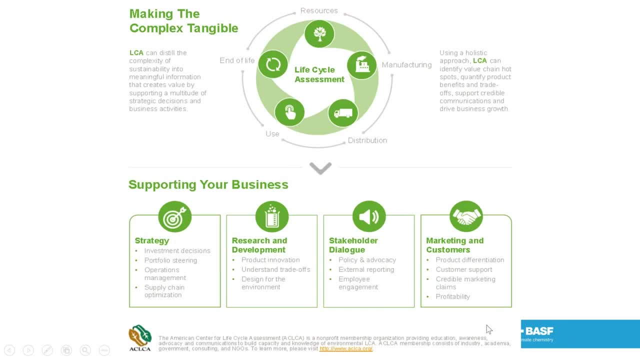 So you would do the same thing. So again, life cycle assessment is really helping us make the complexities of sustainability manageable and tangible for us to really integrate and better understand, And it really supports your entire business. You can see from the table here, which was adapted from a brochure from the American Center for Life Cycle Assessment, that LCA is really a great approach for us to really get our hands around. 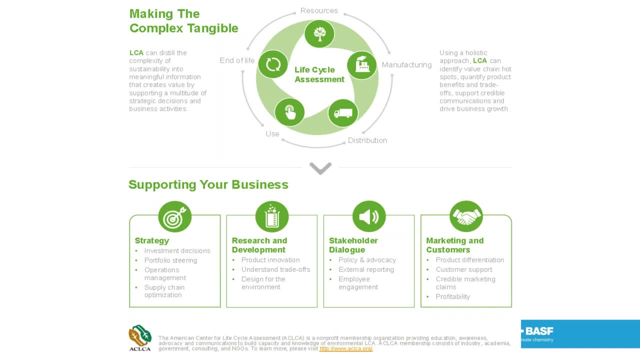 And it's a great approach for us to really get our hands around The environmental and also economic and societal impacts that our solutions are having over their full life cycle, understanding benefits and tradeoffs and really enabling us to drive more sustainable solutions out there in the marketplace. 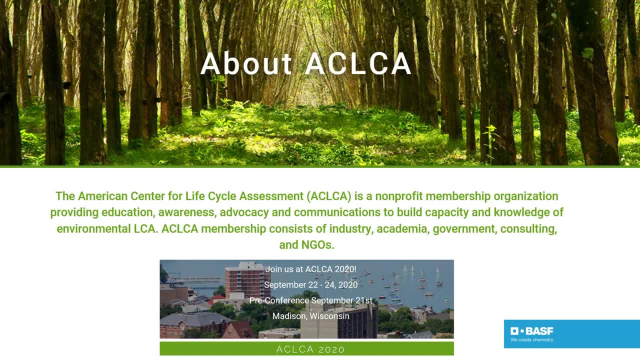 Now, if you're interested in learning a lot more about ACLCA or becoming part of that community, you can see here and reference their website. They have a conference coming up later this year in Wisconsin where a lot of people will be getting together to really discuss. 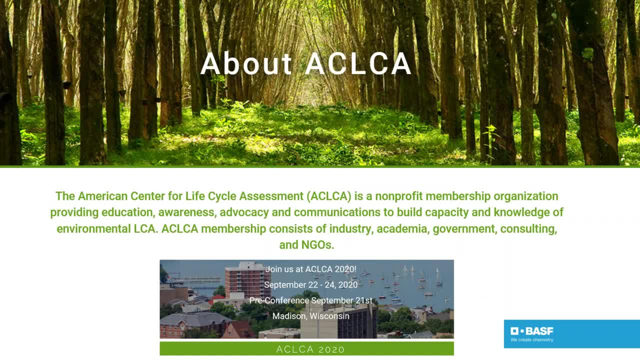 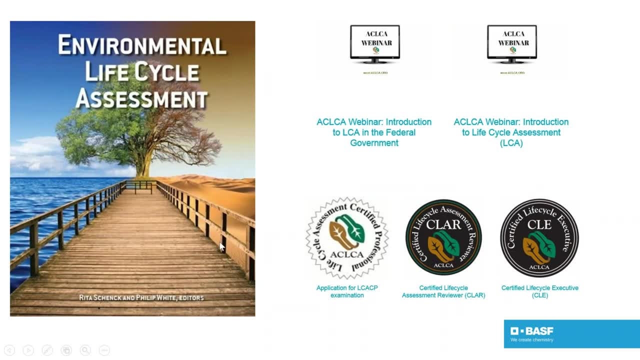 the benefits and implementations of LCA throughout industry, but also, in the broader sense, within our society. It's a great resource on their website, too, to learn more. They have academic books around teaching you around lifecycle assessment. There's webinars and information to know how to become, say, a certified LCA practitioners. 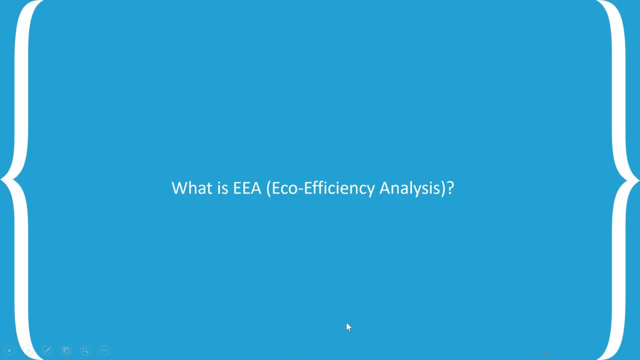 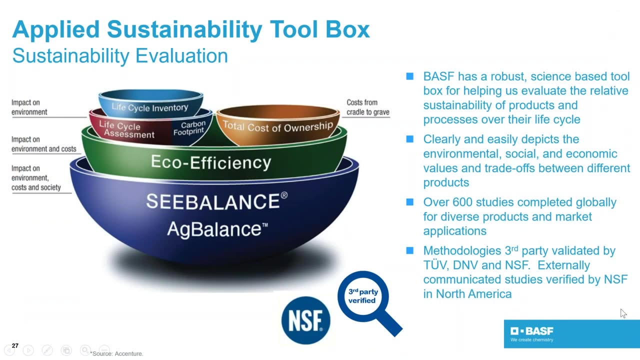 So great resources for everyone to really understand more about LCA. But now what is eco-efficiency analysis, specifically around BASF's methodology? So BASF has been developing a robust toolbox around lifecycle assessment for over 25 years. We've completed over 600 eco-efficiency analyses and we're really using this as a strategic tool for our businesses and customer engagements. 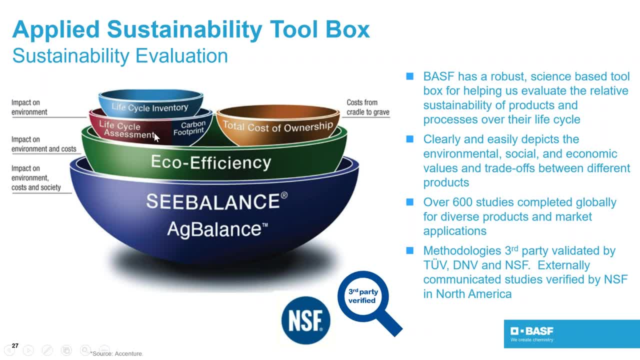 So we have traditional lifecycle assessment tools that enable us to measure that environmental pillar and measuring water footprint. So we have a total cost of ownership tool which is a lifecycle costing tool. But we knew we needed to combine the business case with the environmental impacts. 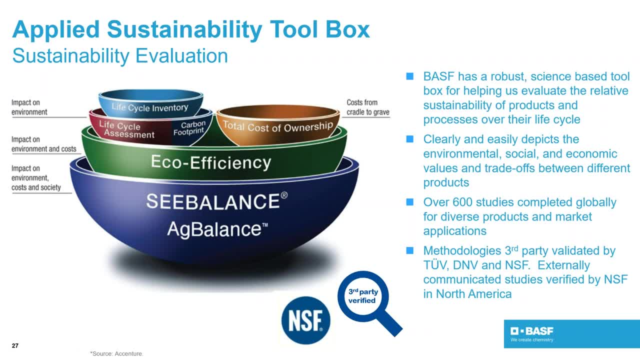 so we combined that in our eco-efficiency analysis. So here we're measuring together concurrently the environmental and economic impacts of solutions. But we also understand that we sometimes need to quantify social impacts, and we have the sea balance and ag balance tools To help us accomplish that. 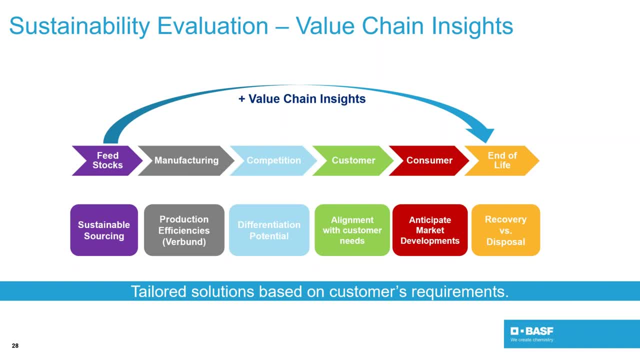 So LCA is really providing this great insight into our value chain At BASF and other companies too. you can use LCA to help evaluate feedstock choices. There's a lot of discussions about fossil versus renewable materials, which are more sustainable. 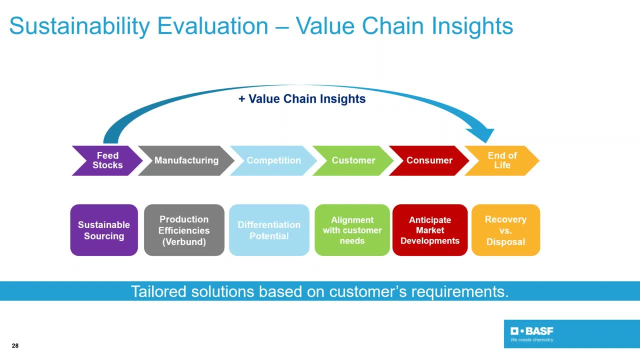 LCA can help you with that. It can also help you understand the benefits, say, at BASF, with our furbooned manufacturing plants where we have heat integration and resource recovery. What are the benefits of that? When you do a comparative LCA you can understand your differentiation potential with the competition. 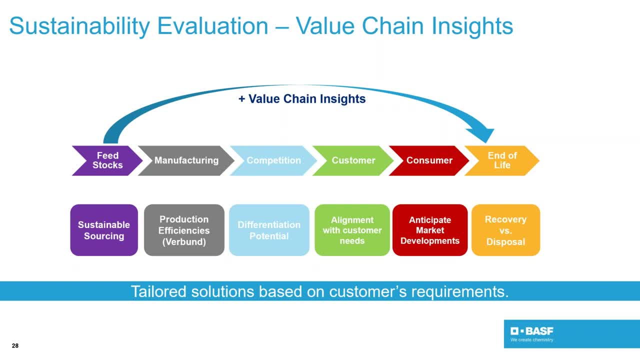 Sometimes you have benefits, in some cases you may have tradeoffs, But the most important thing is LCA, because of that full value chain perspective allows you to understand the needs of your customers, of society, and align your solutions environmentally and economically. 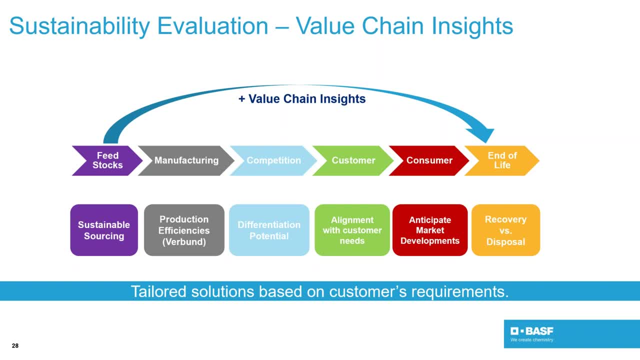 economic benefits with those and finally- and I'll give a case study later on in the presentation- it really enables you to get a better understanding of end-of-life options, of bringing some science and quantification to circularity. what are the impacts and benefits of, say, traditional disposal? 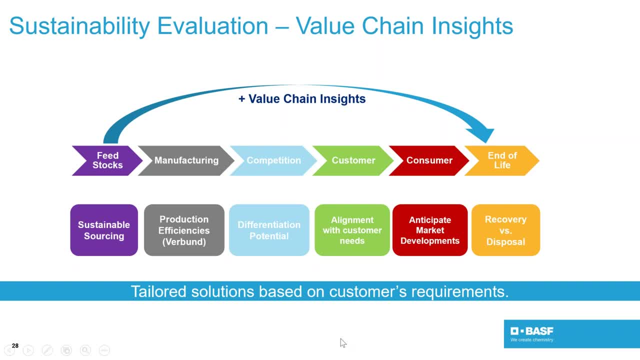 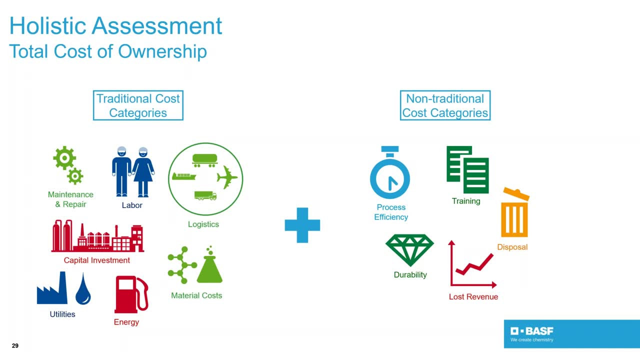 landfilling or incineration versus recovery and reuse. so within the eco efficiency analysis I explained, we're covering two pillars of sustainability, the first one being the economics, and you can see here that we look at a lot of traditional cost categories over products lifecycle, such as material costs, cost of energy, labor, maintenance and repair. but LCA allows us. 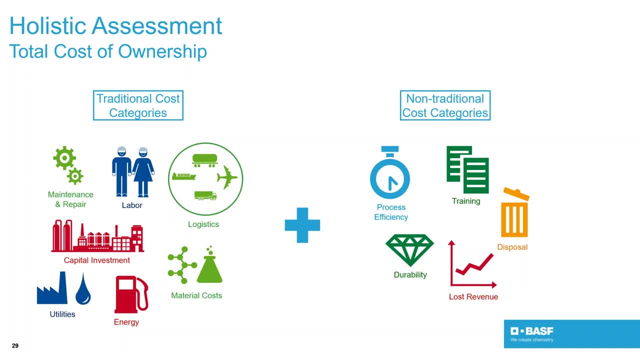 to take and look at things through a different lens as well, and it enables us to bring in other economic impact areas such as, you know, durability and process efficiencies. if your solutions are enabling those LCA's are enabling those LCA's are enabling those LCA's are enabling those. 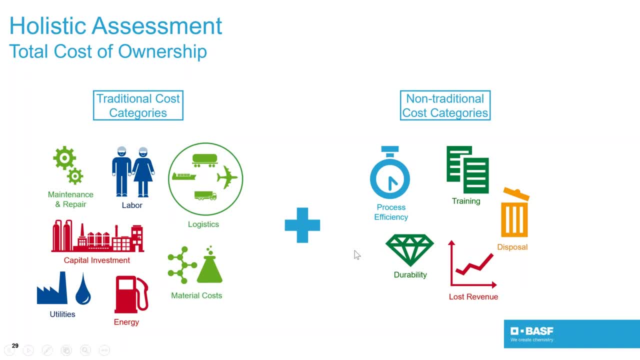 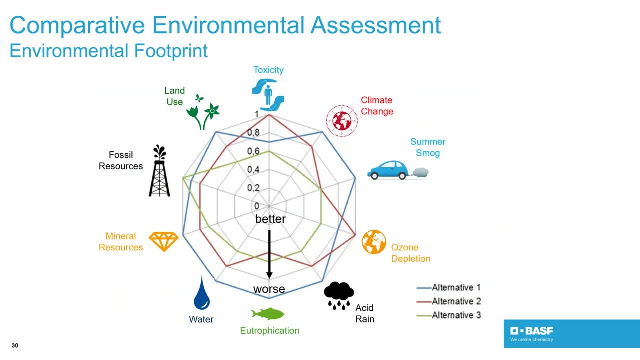 LCA enables you to capture those economic benefits, quantify those and communicate those. now, as I explained earlier, we're assessing a lot of environmental categories within lifecycle assessment. we're calculating input and output flows and then characterizing those into areas such as climate change, water use, land use, summer smog- and in many cases it can be. 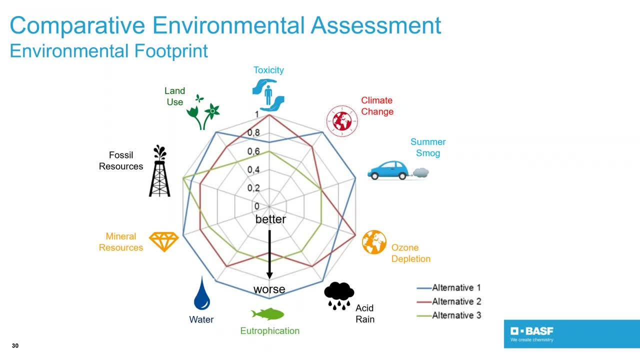 overwhelming with the amount of information that you have and the impact that you have and the impact that you have and the impact that you have. so we like to communicate those environmental results with LCA results in an environmental footprint or a spider diagram, and this enables you to really 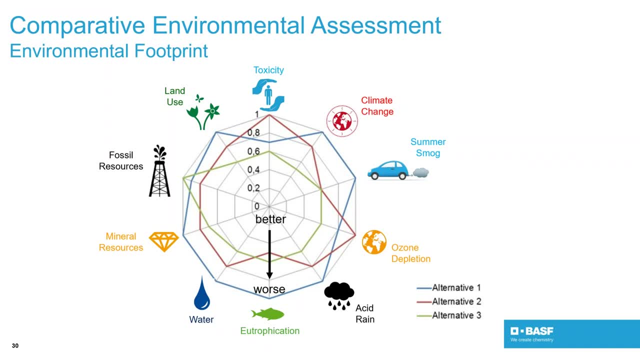 look at all three alternatives here that were assessed- you know, doing that same functional unit- and how they compared relative to one another in each of those environmental impact categories. if your alternative had the highest impact, it would be normalized to a value of one, and if you had lower impact with the 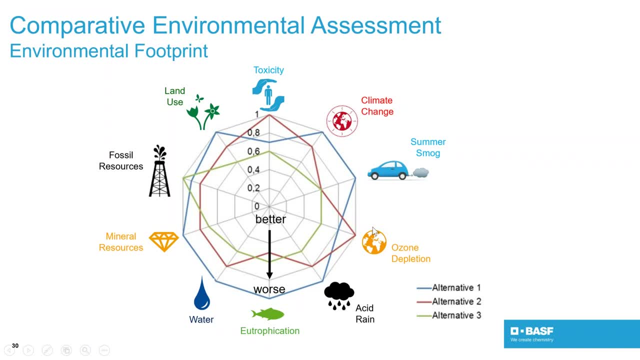 approaching zero and showing better performance. so this enables you to get that good overview. but, as you can see, sometimes you perform better in one area, sometimes you perform worse in other areas. so many cases you can use weighting factors to help you distill that down into, say, a single environmental score. 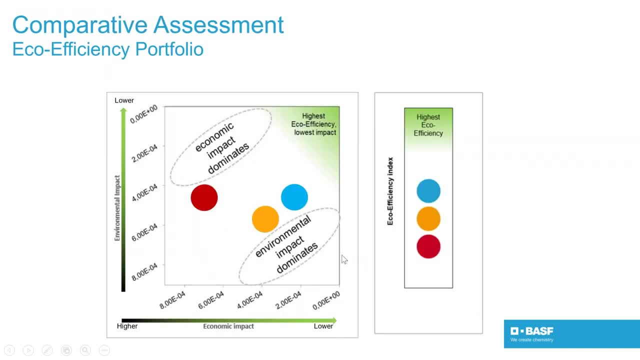 and we do that using our eco efficiency portfolio. here you can see, on the x-axis we use the total cost of ownership normalized score for all three alternatives, with the highest score being to left, lowest score to the right, and we show that single environmental impact. on the y-axis want to be up to 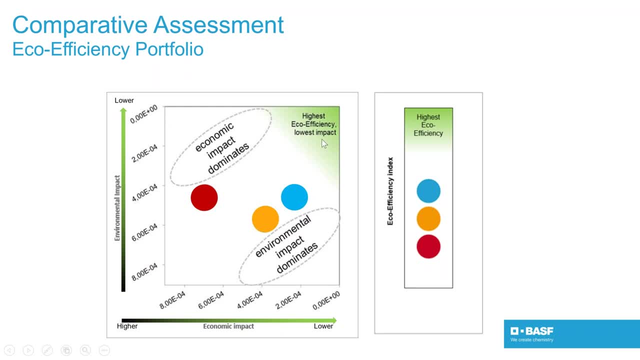 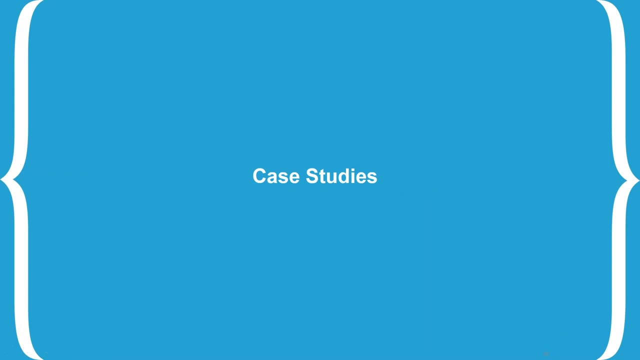 the top here, showing the lowest overall environmental impact, and you really want to drive those products up to the upper right-hand quadrant, which is really understanding driving the best business case with the lowest overall environmental impact. so that's all for this video so far, eco efficiency methodology. I'd like to move into some case studies here, which 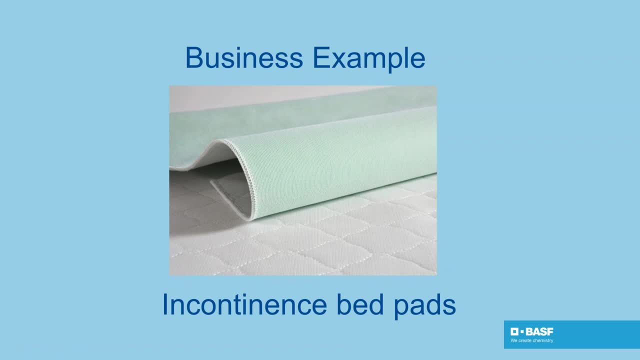 show the application of that methodology of LCA and eco efficiency analysis and I want to show here a case study around incontinence bed pads. so the healthcare industry is also concerned about their eco efficiency and the impact that they're having on the environment. they want to drive greater sustainability use. 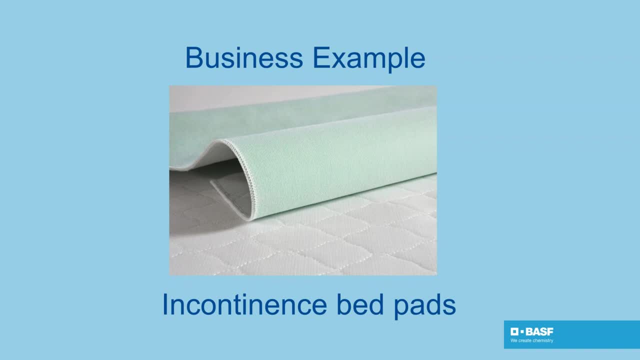 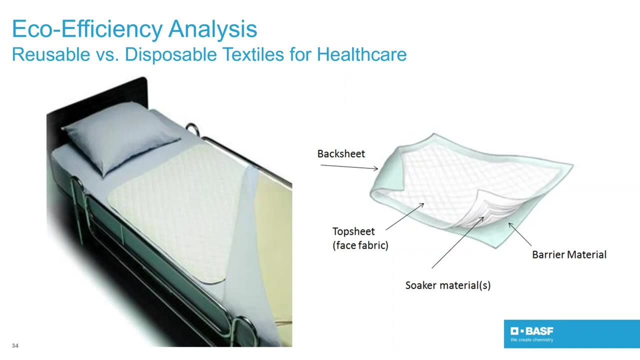 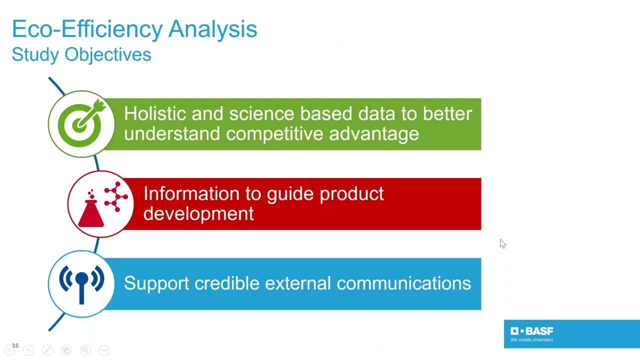 more sustainable materials and one of the debates that they've had longstanding debate is around reusable versus disposable textiles for healthcare. which one is more sustainable. well, our customer came to us and said: hey, we'd like to use LCA- eco efficiency analysis- to really provide some science-based and 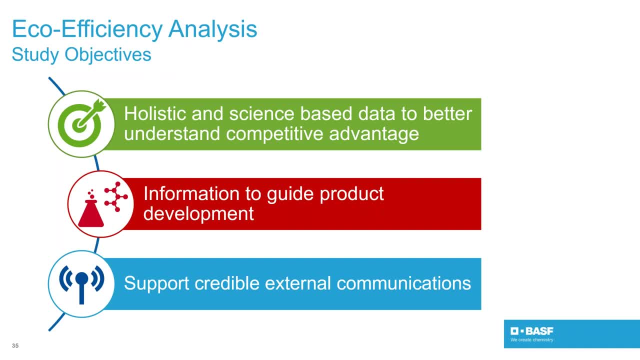 holistic information for us to really help us understand our competitive advantage. help gain some information on where our hot spots are and how it's going to impact our business case. study whom we guide our product development team to drive greater sustainability, reduce our impacts, improve our performance. 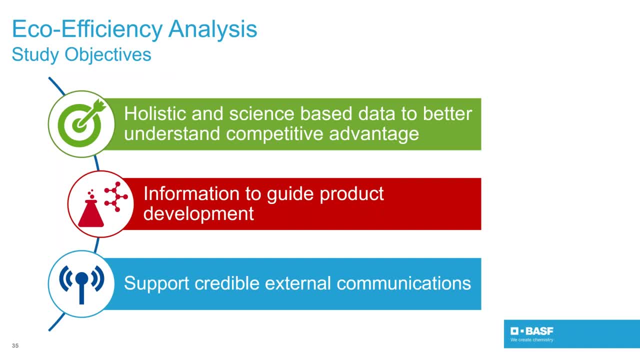 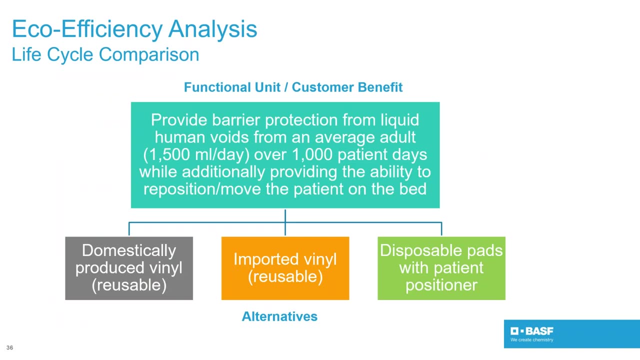 but also we want to not contribute to additional greenwashing. We want to have credible, science-based claims out there for our product. So can eco-efficiency and LCA support us? And it clearly can. So the functional unit that was devised for this study here wasn't just around. 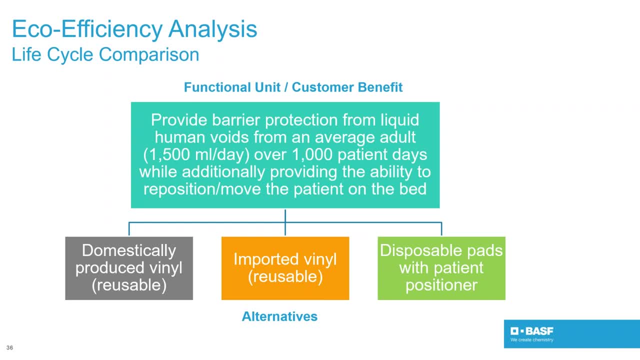 absorbency of these thousand patient days. but we had to look at the extended performance attributes of some of the reusable vinyl bed pads And we knew that the nurses and healthcare professionals could move patients with that. That was a very critical performance attribute. So we built that into the LCA and said that okay. 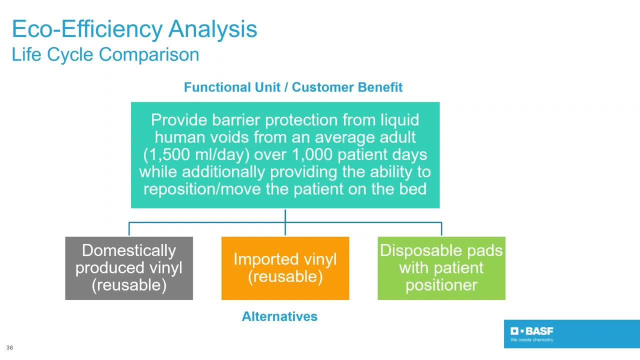 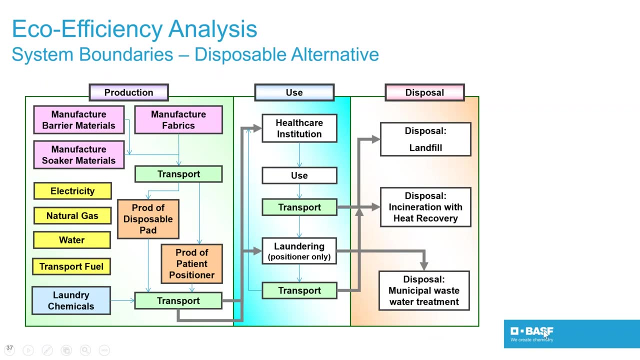 the disposable pad couldn't do it by itself. but to get that function equivalent we had to add a patient positioner to the scope of the disposable pads. So you can see here, just like in understanding the full scope of that life cycle. 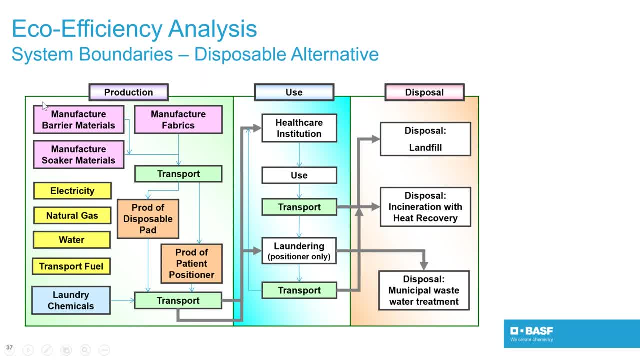 we had a holistic perspective of what we were measuring. You can see here, in the production phase we were looking at assessing all the raw materials, all the utilities. We looked downstream that the reusable pad had to be laundered, So we had to develop the laundry chemicals. 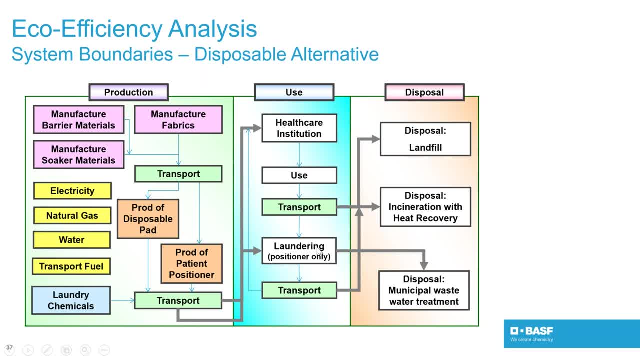 We looked at the use phase product here. So in the use phase for the laundering activities we had a look at transport to the laundering facility, the emissions from laundering And transport back to the healthcare facility, And then we looked at various end of life disposal for those alternatives. 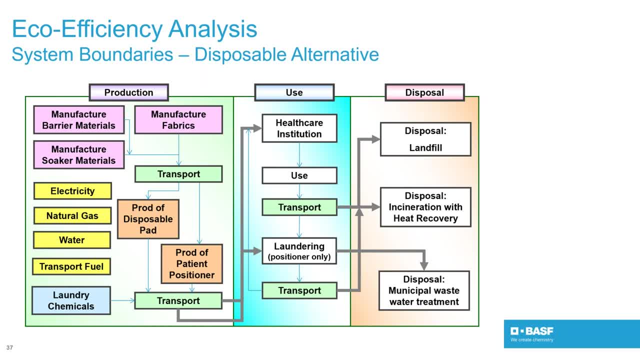 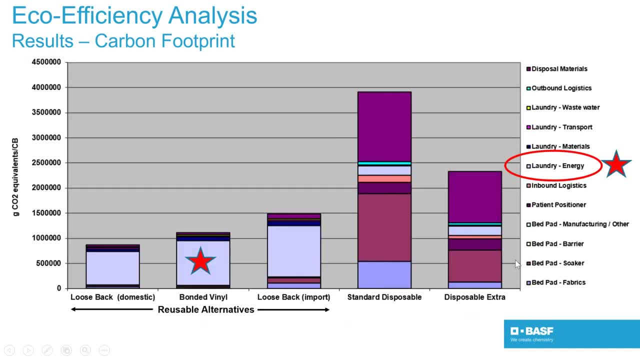 which could be traditional landfill or perhaps recovery through incineration. So what were the results of this study? Well, looking at one of the popular metrics here for carbon footprint, you could see that we learned for the reusable alternatives that the key driver for the carbon footprint was actually downstream of our customer. 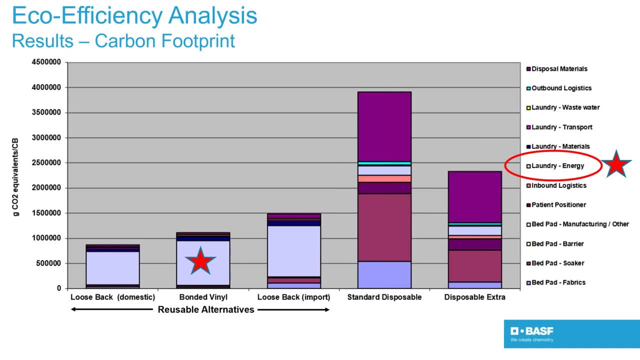 It was in the laundry phase, It was in the laundering activity. So all heating of the water, the getting of the water, the wastewater emissions were really the key driver for the carbon footprint. So that was a perspective LCA brought, that it was downstream. 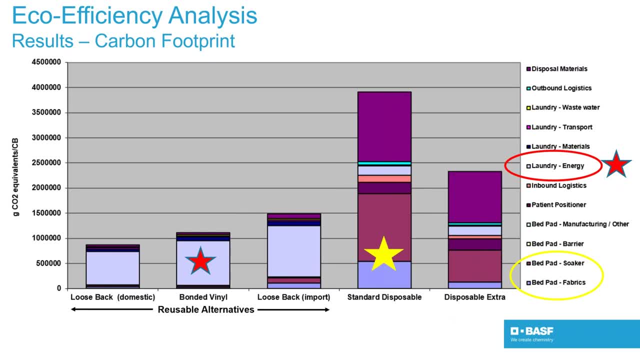 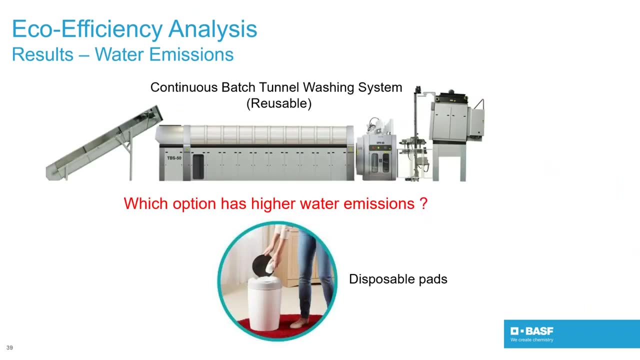 But for the disposable alternatives, we could see that the impacts were both at the raw material stage but also at the end of life, the end of life disposal here. So interesting perspective that the hotspots, as revealed by the LCA, were different from each of the alternatives. 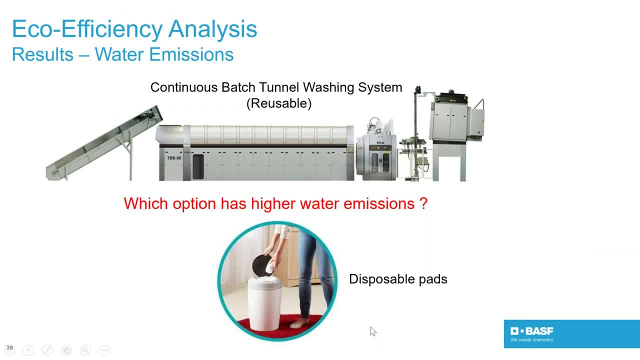 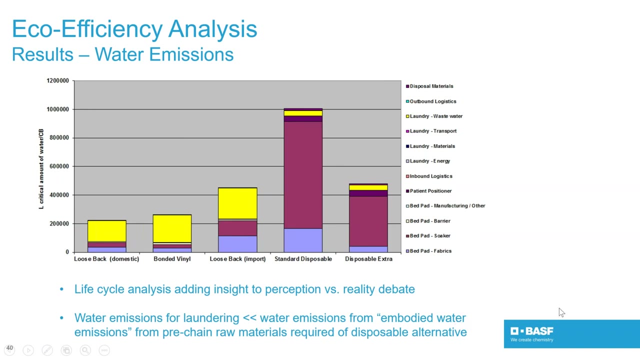 Now, how about a question around water emissions? Perception would say that the reusable alternatives that were using these big tunnel washers would have higher water emissions than disposable pads that you were only disposing of in a trash receptor. But the LCA brought a new perspective to that. 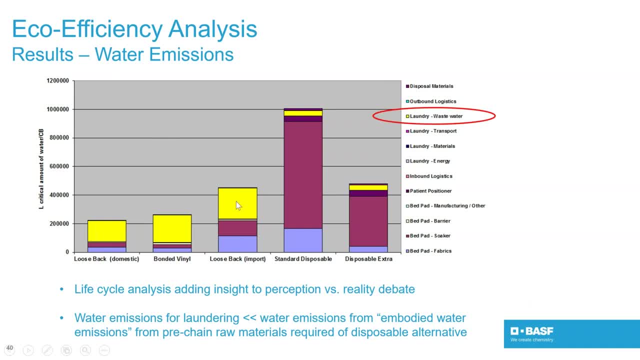 It actually, through measuring things, we understood that, yes, the hotspot for the reusable alternatives was the laundering, but the overall water emissions over that life cycle for the disposables were much higher. And how was that? Well, LCA enabled us to look upstream at those embodied water. 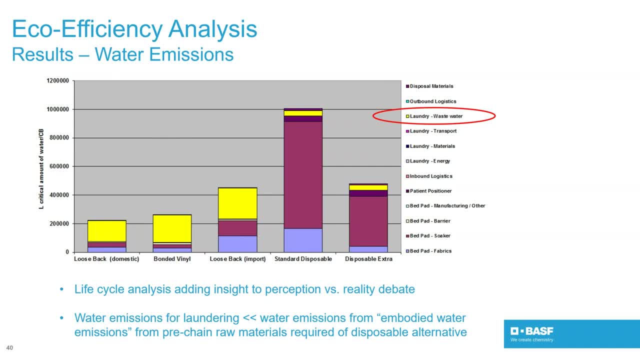 emissions that were being admitted through the production and extraction and production of all the raw materials that are being used by the disposable alternatives. So this was a way that LCA brought some science and reality to the perception of where those overall life cycle water emission impacts would have. 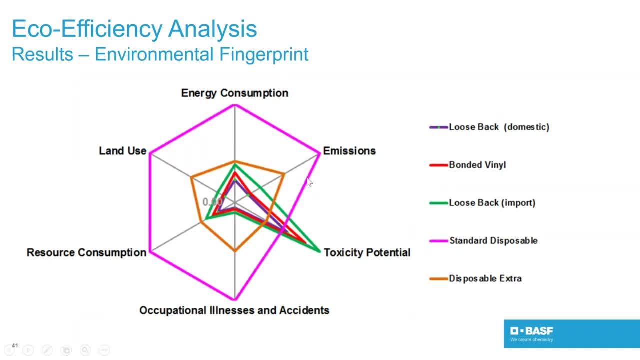 been So. here is the environmental fingerprint for the alternatives. You can see here that the first three alternatives, being the reusable ones, had overall inconsistency, the lowest overall environmental impact in most all the environmental impact categories, except for the toxicity potential, And this actually had to do with the use of all the chemicals in the laundering. 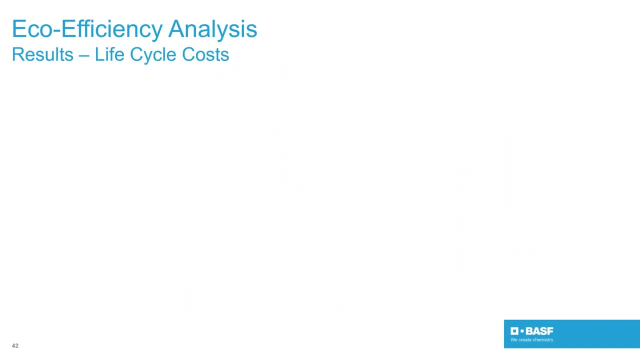 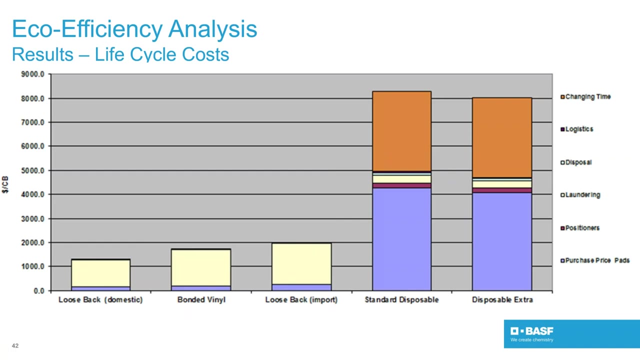 activities that were further down the value chain. We looked at the life cycle costs as well And using a total cost of ownership perspective. this enabled us to really bring a unique perspective and move, from our customer's perspective, the discussion away from the purchase price to the total cost of ownership. 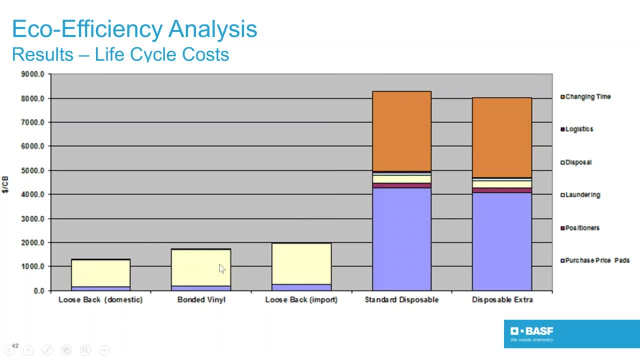 So you can see here the cost for the reusable were mostly around the cost for laundering and maintaining this reusable pad over its life cycle, And the cost for the disposable were from the materials. but also, from another perspective too, were from the cost of the materials. 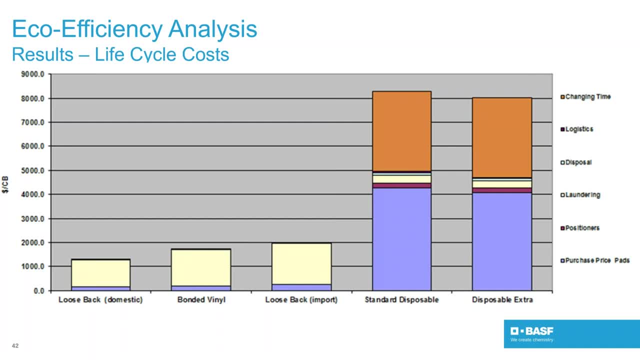 They were from the additional time that was required by the nurses to change the bed pads. They needed more frequent changes than the reusable pads, So we were actually, from a total cost of ownership perspective in the LCA, able to incorporate that in the economic assessment that we were able to do. 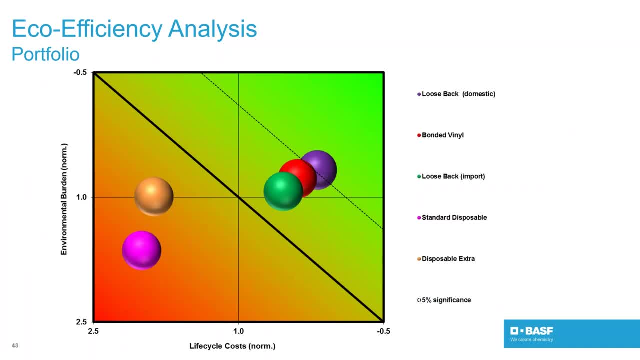 So when you combine those environmental and economic results together in our eco-efficiency portfolio, you can see that the reusable pads here were clearly from the business case, had the lowest total cost of ownership and the loose back domestic and the bonded vinyl had the lowest overall. 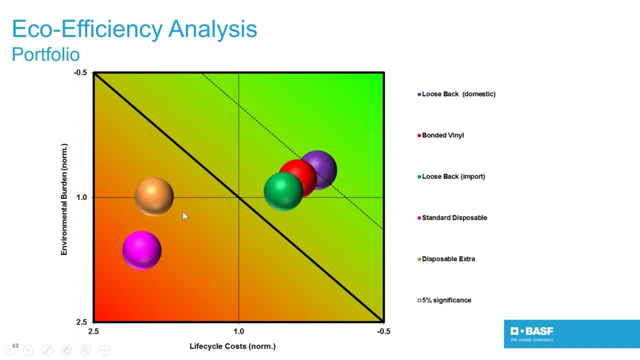 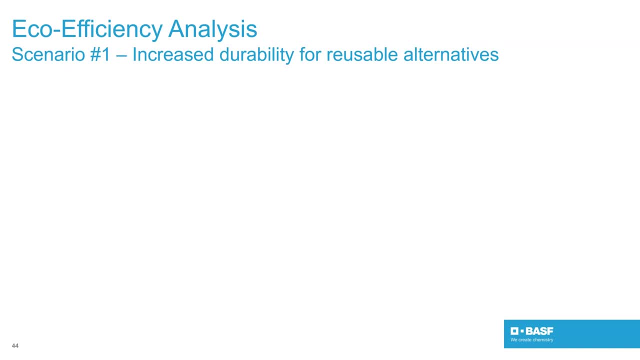 environmental impact of all the alternatives. And here you can see the disposable pads. But, as we said, that LCA can provide you insights that can support product development. our customer asks: well, we have a durable pad. If we increase durability, that must make us more sustainable, correct, Well? 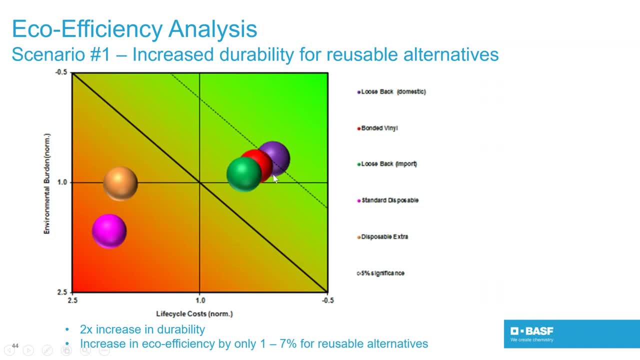 the LCA, we showed different results. If we showed through a sensitivity analysis that we increased the durability by double, it only increased the eco-efficiency of that product minimally by one to 7%, and that was because the majority of the impacts were occurring downstream in the 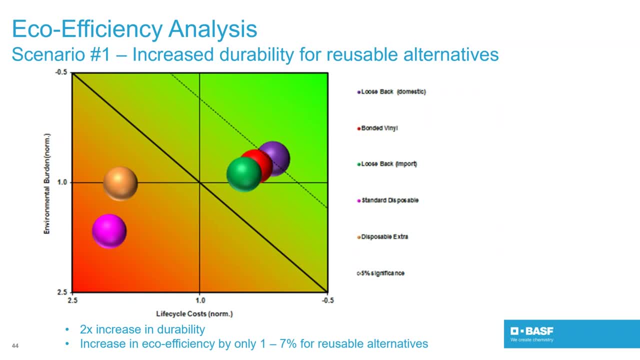 laundering activities and had really very little to do with the durability of the product. So if we wanted to optimize, then the sustainability of that entire operation we should focus on how can we make laundering more sustainable? Now can we look at the competing technology and say, well, 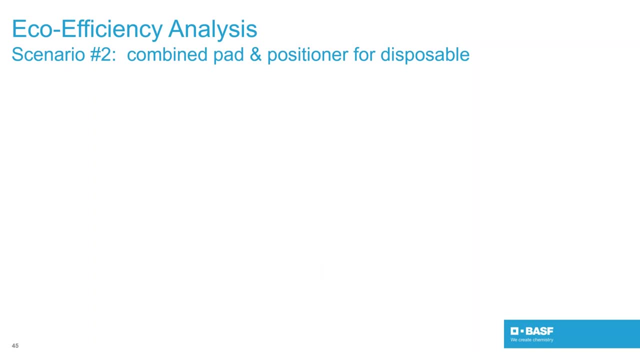 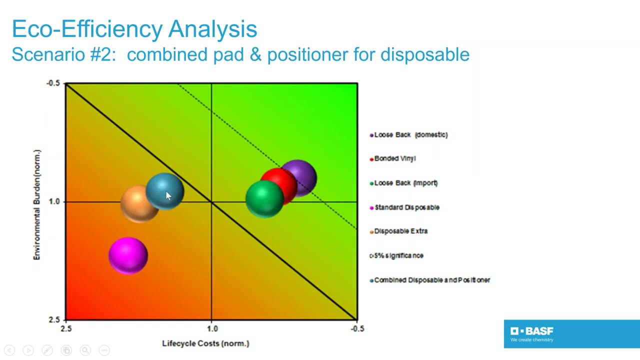 can we combine some functionality into that disposable pad to make it being able to move the patient? How can that drive that better sustainability? And you can see that alternative is here in that blue alternative. It did improve the overall sustainability but not enough to really overtake from an eco-efficiency standpoint. 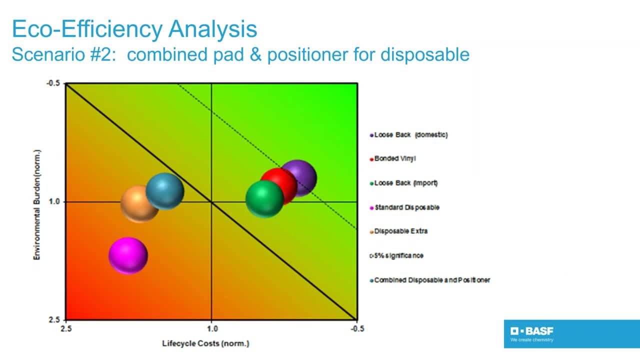 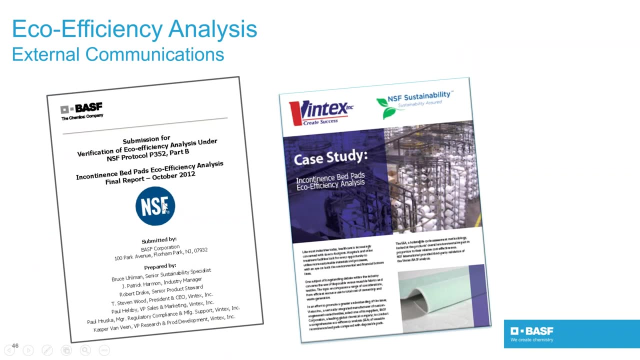 the reusable alternatives. So great insights that we were able to achieve, uh, through the LCA. Um, we did- because we were communicating this externally- go out and have a third party reviewed by NSF And, more importantly, we created some easy to understand marketing brochures for our customer to make. 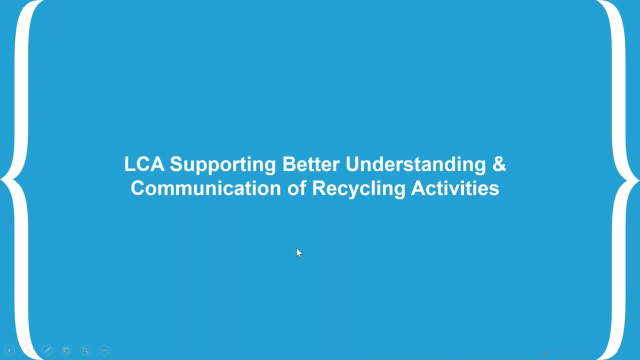 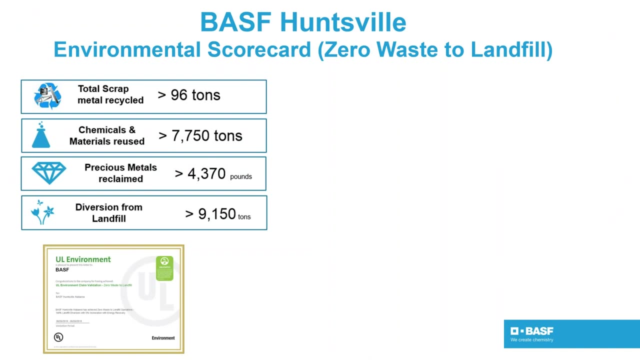 sure that this information, the rigor of the LCA, can be translated and understood more effectively. So, if we look at um how LCA can support recycling activities, this is a brief uh case study here. Uh, you can see here of how we were able to quantify and communicate the benefits. 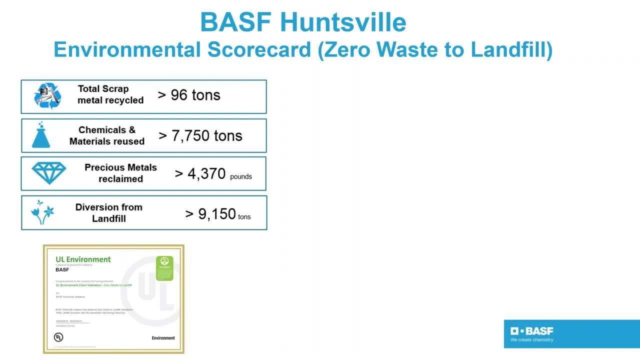 of one of our manufacturing sites going zero waste to landfill, really trying to optimize and reduce any type of waste streams and generation of any waste. So you can see over here they were collecting and reporting a lot of scrap material and chemicals being reused. uh, reclamation of precious metals from the site. 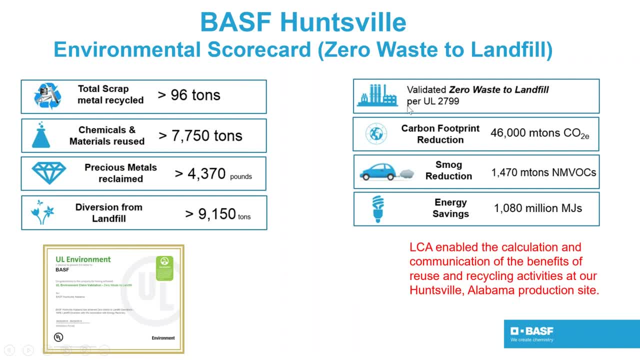 And we were able to use LCA to really quantify those benefits, As you can see over here: a significant reduction in waste, in carbon footprint reduction, in summer smog and energy savings. So LCA really enabled us to communicate, not only to be without. 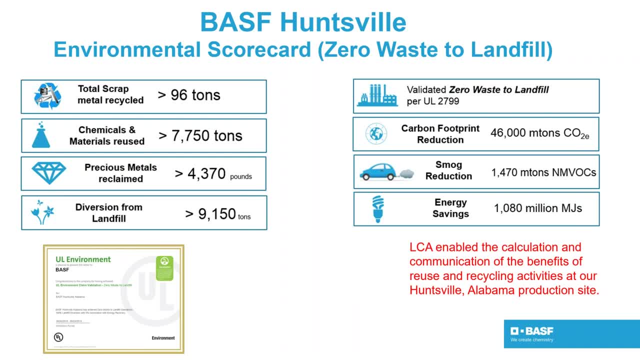 around BASF, but also to our stakeholders and to the communities that we operated in that by taking responsible action of minimizing waste. this is the impacts that we're having, both from a regional and a global basis and reducing environmental impacts, And we are recognized in 2018 for those efforts by the ACC. 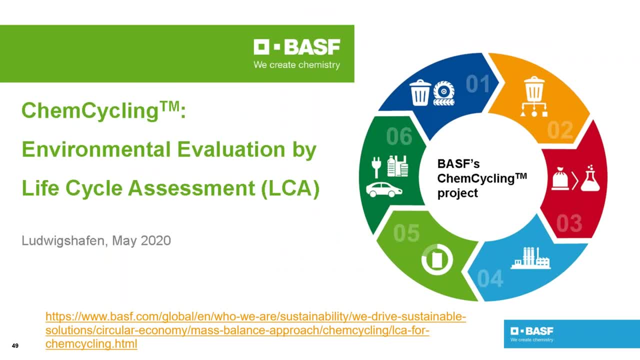 and also have gotten the certification for UO for zero waste to landfill site. So, uh, the last case study here I'd be happy to talk about here- and we just released those results recently- is around our chem cycling, uh, technology and process. So you know. 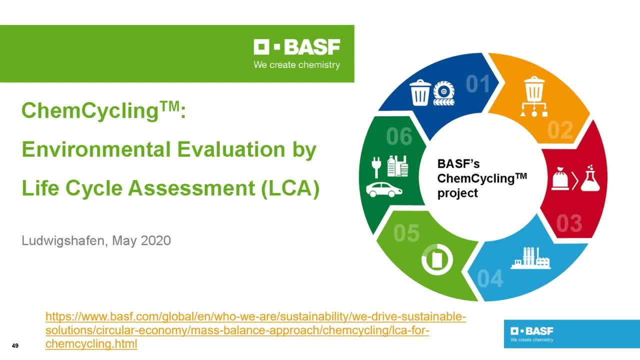 we all know that plastics have a real great benefit in their use: Um, they protect food preservation, light weighting of construction, uh building installation, so really a great sustainability story for plastics. But, however, there's a lot of negative press here and also some reality around plastic waste. 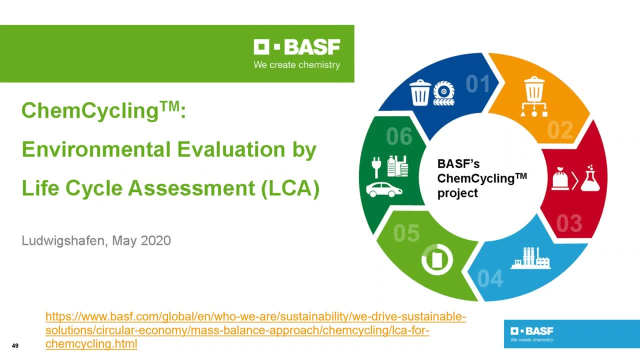 And it's a big challenge for us, And we know that. uh, you know, mechanically recycling plastics has its limitations. So BASF came up with this innovation of chem cycling, which really allows us to recycle these plastics so that, where there are no, 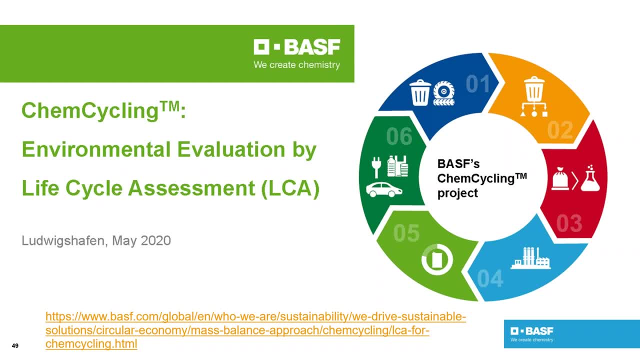 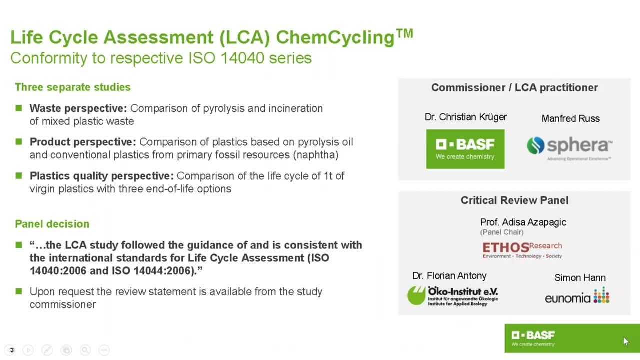 longer, some viable recycling options available and we can turn that back into a valuable resource. Take it away from the landfills and incineration and turn it back into a valuable raw material. If you're interested in getting more information, there's a hyperlink here, uh, to the final study here. 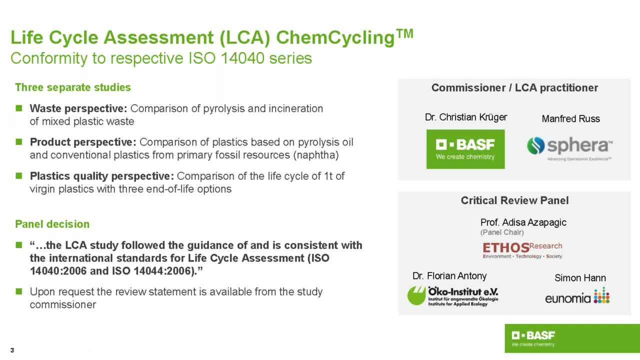 So basically the LCA that was done, uh, for our chem cycling process, looked at three unique applications. So you can see here from a waste perspective, uh, generating this pyrolysis oil from the plastic waste. How did that compare to traditional incineration? 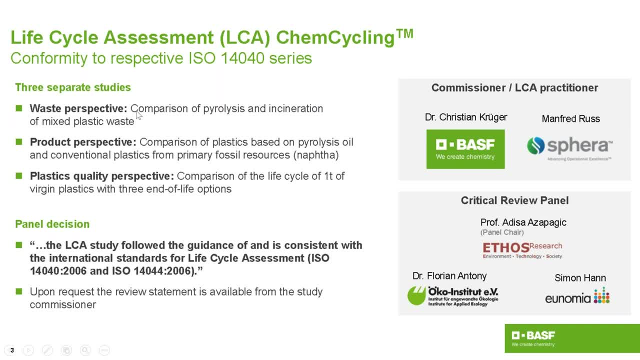 which could have, we see, recovery and generation of electricity. Can we compare then also the production of a plastic material with this pyrolysis oil versus a traditional method which uses oil, And then can we overall make the most holistic comparison of what is that one? 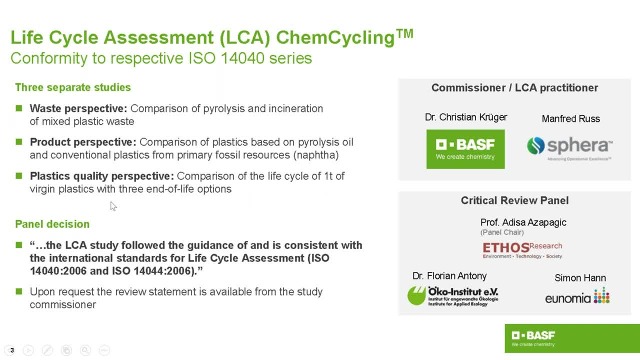 life cycle ton of a virgin plastic material with three end of life options being chem cycling, mechanical recycling or incineration. So this assessment that I'll be presenting the results from uh followed the ISO standard that did review, go through a critical review panel Um. 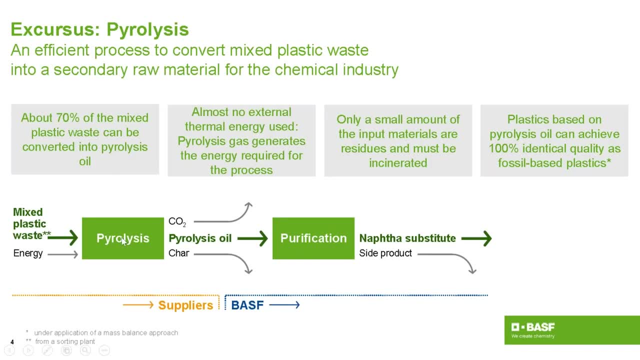 so it did have those expert eyes taking a look at it. So this is just the flow stream here of what we were assessing, uh, in the generation of this pyrolysis oil. So we were looking at generally a mixed plastic waste, Uh. 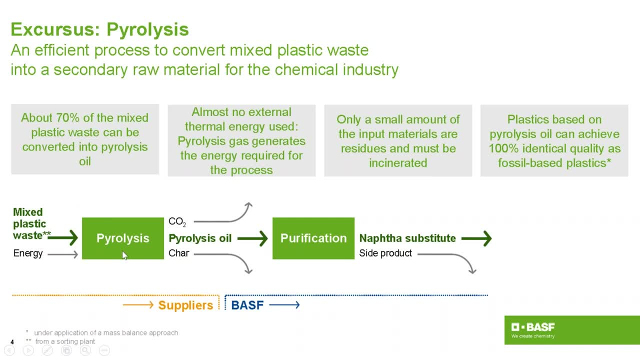 there's about a 70% recovery of those waste that we can use in creating this pyrolysis oil. Uh, through that process we are measuring some of the CO2 emissions, some waste streams. Uh, there is a downstream purification of that before it can be fed into our 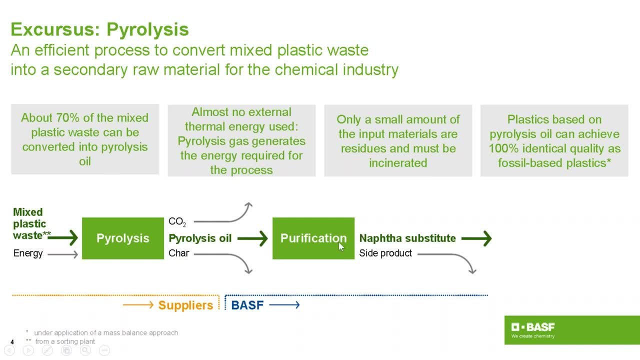 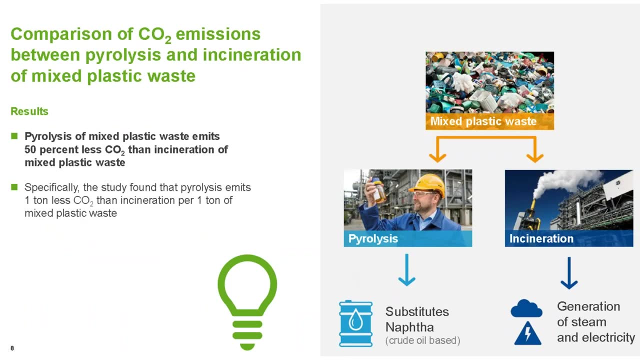 crackers to generate plastic materials, And this is really the scope of what we assess, uh, from our chem cycling process in production of that pyrolysis oil. So here is the first results, which is looking at the substitution of pyrolysis oil in our cracker. 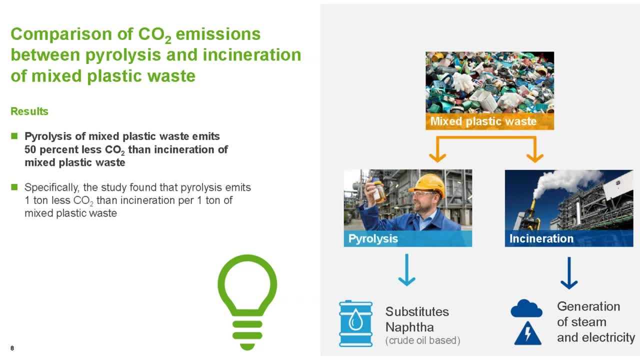 uh, and getting some benefit of not having to use a basic, a non-renewable resource such as napkin, which is a non-renewable resource that can be used in the production of plastic materials. And then the second is looking at the carbon footprint and comparing that to 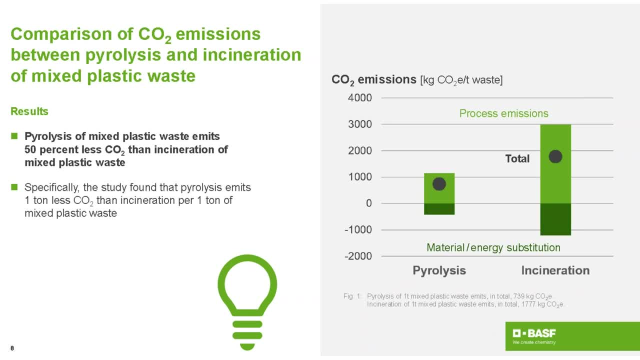 the traditional end of life of that plastic material, which would have been incineration with recovery of steam and electricity. So as you can see here um the carbon footprint is much reduced for the pyrolysis Uh overall the incineration here uh. 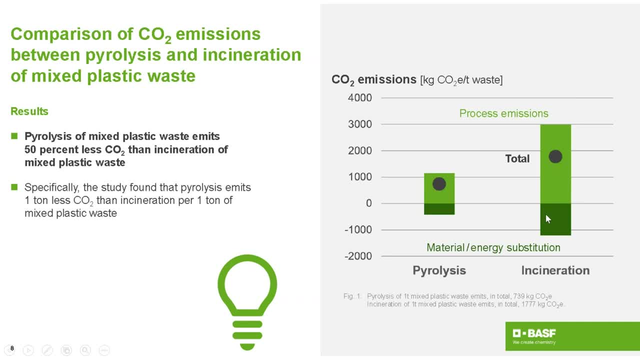 is about 1,777 kilograms of CO2, some benefits um from, as I said, the generation of electricity, So it did lower the overall carbon footprint. but clearly, even taking here some of the benefit of the NAFTA, the overall carbon footprint for the pyrolysis is much less saving about one. 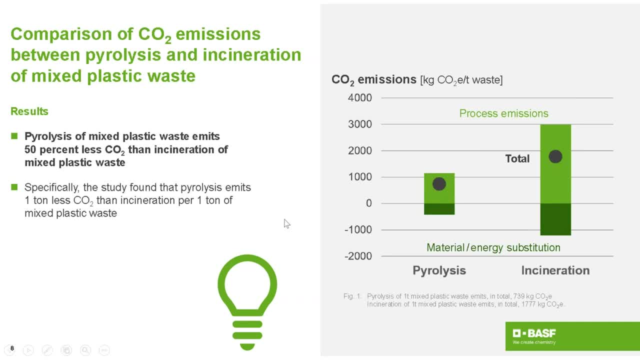 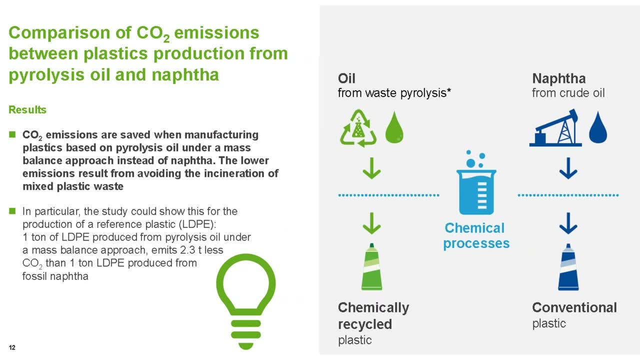 ton of CO2 per ton of plastic waste material- uh. that was being assessed So very significant. Now in the second case study we looked at the production of uh one ton of of plastic materials such as low density polyethylene uh. 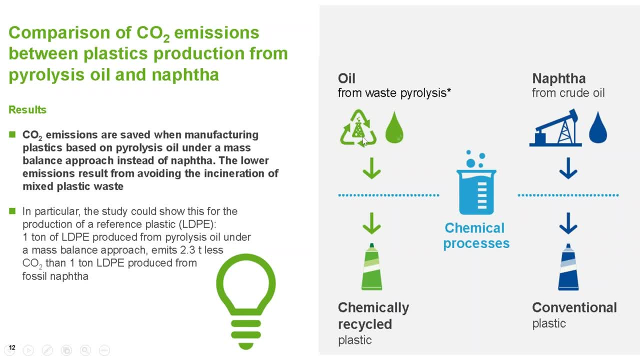 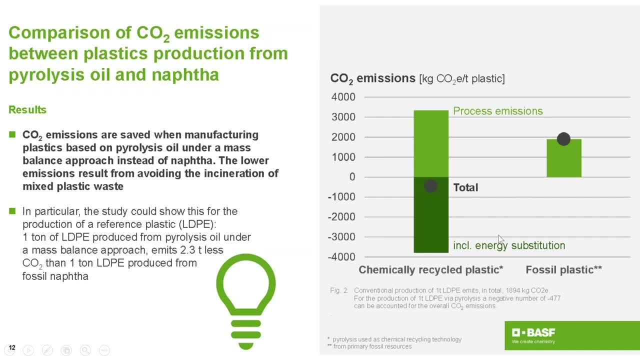 through either using uh, chemically recycled pyrolysis oil or traditional NAFTA. And when you look at those results here, you can see a much significant benefit: using that chemically recycled plastic material, savings of almost 2.3 tons less CO2 emissions. 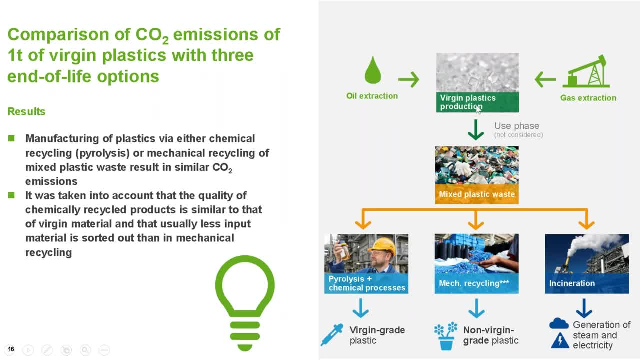 And finally, the last comparison here was looking at the production of virgin plastic material and looking at three uh end of life options. Should we generating pyrolysis oil and further use of that to generate virgin grade plastic? uh using that plastic material now into a mechanical recycling? 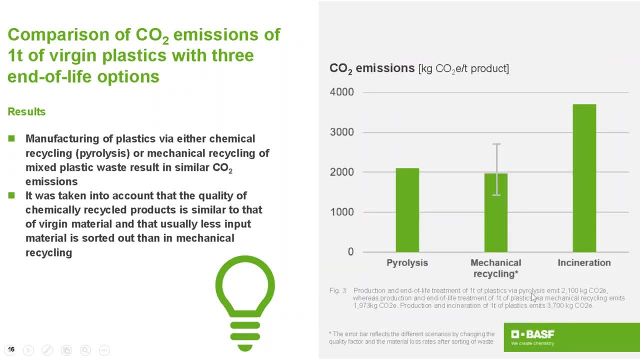 and then also traditional um disposal, such as incineration and landfilling, And overall. you can see here through the results um that and you can see the sensitivity um sensitivity band for the mechanical recycling, because um 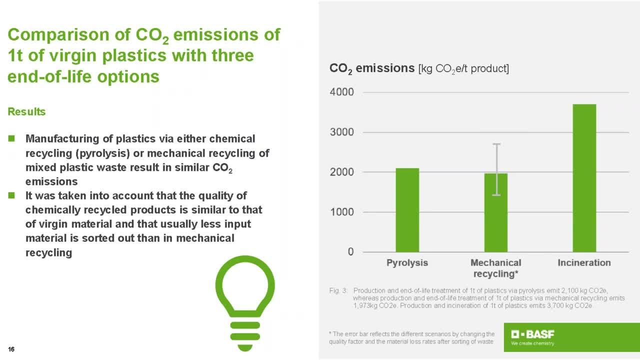 when you mechanically recycle the product you know there could be some quality factors um losses because of sorting, but overall pyrolysis oil use in this area was comparative uh to the mechanical recycling and clearly better than the traditional end of. 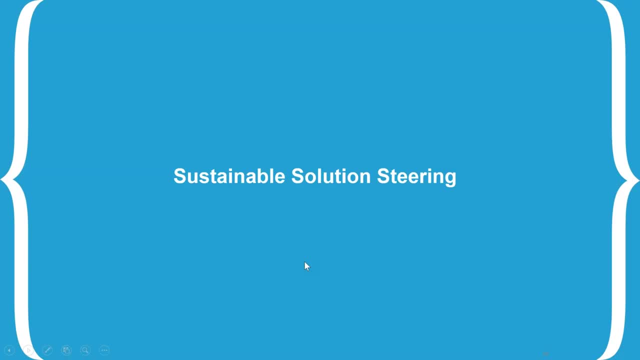 life through incineration. So great story here for us: using sustainability to better understand and life cycle assessment, the innovation of chem cycling And just to close off, here you can see the power of life cycle assessment and being able to really quantify in a science-based way. 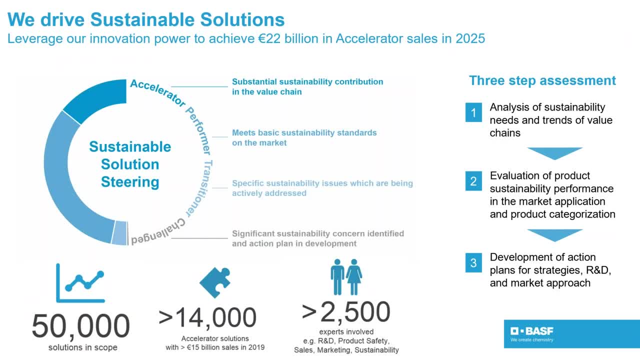 those environmental and economic impacts of our products. But the power would be: can you bring that to a company's entire portfolio? Can you bring life cycle thinking, even life cycle assessment, in a methodology and approach to assess all of our solutions, not just the the ones that you do these six months? 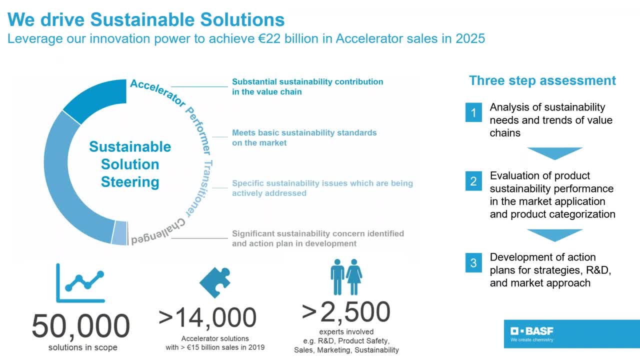 the one year LCA studies for. So BSF developed the methodology, uh and approach through sustainable solution theory that really enables us to take that life cycle perspective, assessing in a rigorous manner the environmental, economic and social impact and benefits our solutions are having and really enabling us to identify those. 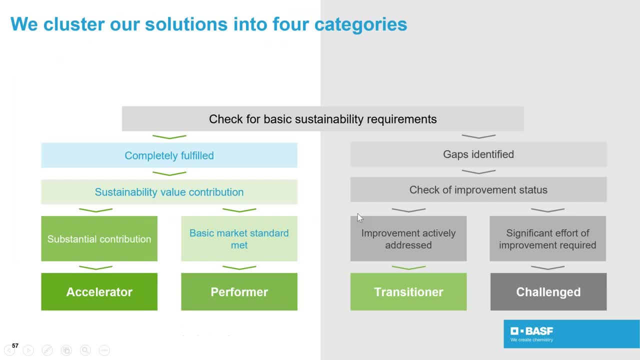 sustainability, leading solutions and being able to communicate that clearly to our customers With. the methodology and approach is out there. we've published a brochure and a methodology for that, but basically, uh, we go through here in a matrix decision-making process where we can. 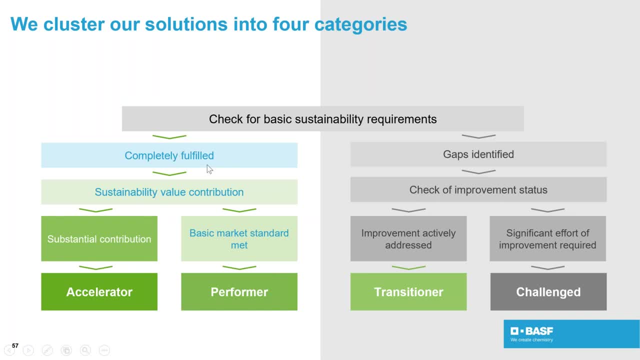 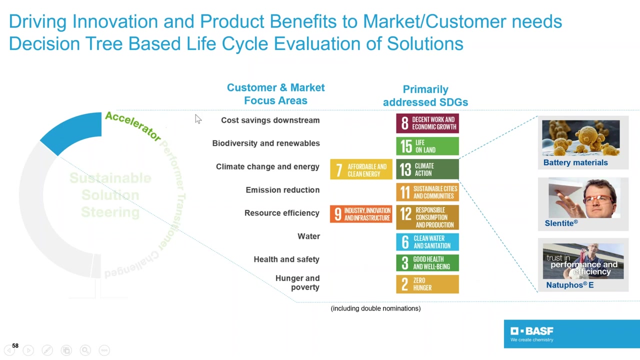 understand what the sustainability contributions of the solution are. understanding any trade-offs, we can also look and assess maybe we have identified some hot spots or some challenges with those products. we can help identify those and innovate those out or move towards our customers a more sustainable solution and it's really enabling us to here to make those connections so for. 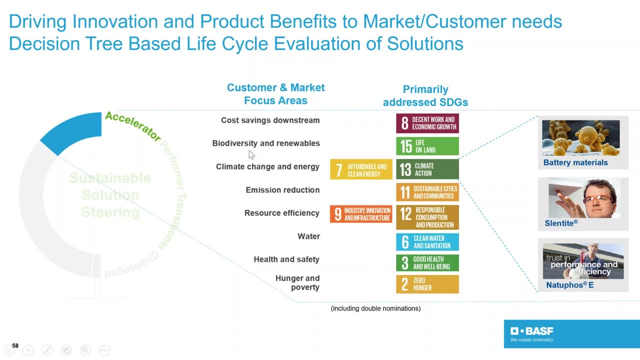 our accelerator solutions, where we can identify these environmental benefits through that lifecycle perspective, we can now clearly link these into these UN SDGs, the sustainable development goal drivers that are important for our society, important for our customers. so this is a great way for us to make the 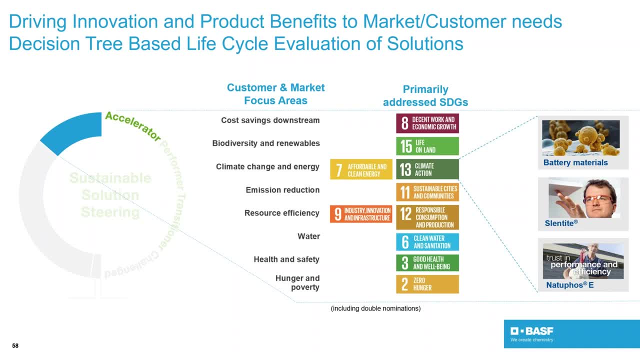 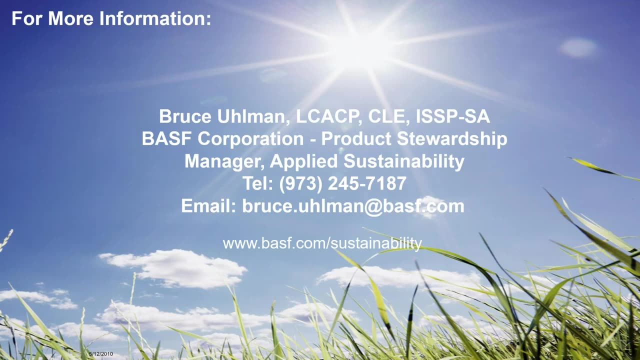 linkage of our solutions, driving value to our customers in society, using lifecycle thinking, using lifecycle assessment, and here is the brochure that is out there in the public, that's open for people to utilize. so with that, I'd like to thank you for the time and the opportunity here to talk and with that I'll turn it back to. 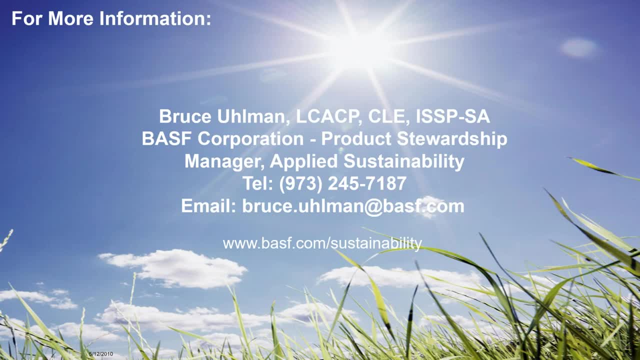 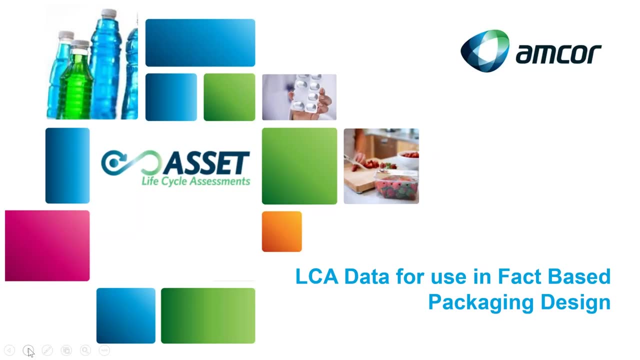 to Ashley and to Dennis. wonderful thank you, Bruce, excellent presentation, as I knew it would be. so I'm just going to advance here and you know, I think, what's what's really great about what we've tried to put together for you guys today? it is the coupling of local 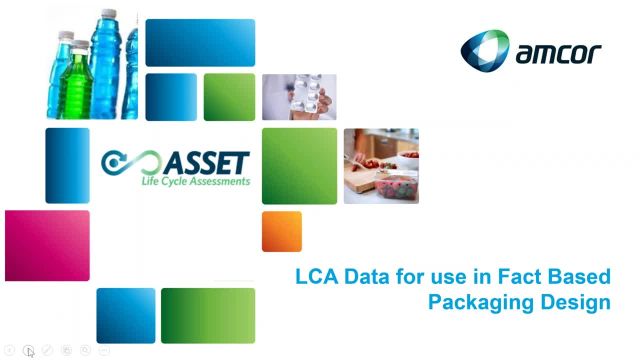 essential materials, and I think that's what's really great about what we're doing, and it's not just about the local and it's really about the local infrastructure as well. and so with that, we are looking at lifecycle assessment through kind of the lens of both a material supplier company as well as a. 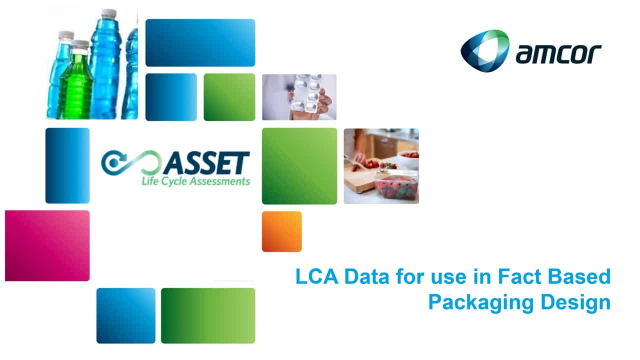 processor company. so looking at kind of two different perspectives in the plastic supply chain on how these tools can be utilized. so with that once again. But if you guys have questions for Bruce, go ahead, throw those in And again, if you do as well, during Dennis's presentation. 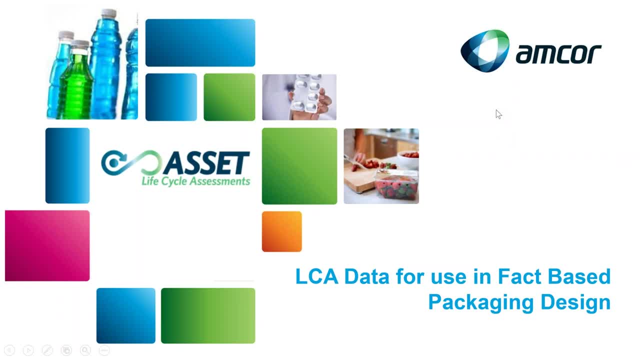 So with that, Dennis, I am going to. you should now have control of the slides, And if you'll unmute yourself, I will turn it over to you. Okay, Can you hear me? well, You are good to go. Thanks, Dennis. 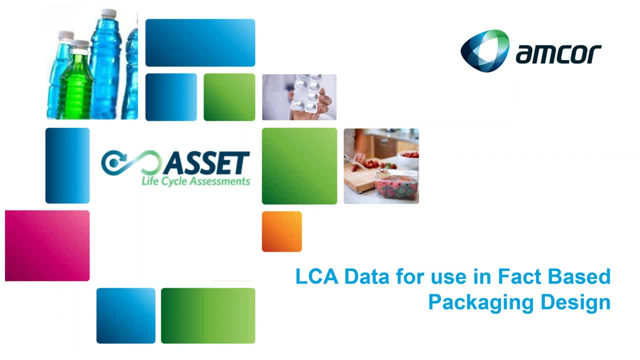 Okay, So I'm Dennis Kittle of Amcor Packaging Company. I work for the Rigid Packaging Division of Amcor And I'm going to talk a little bit about the LCA data and how we use it for consumer packaging. You're going to find a number of similarities between Bruce's presentation, which is very good. 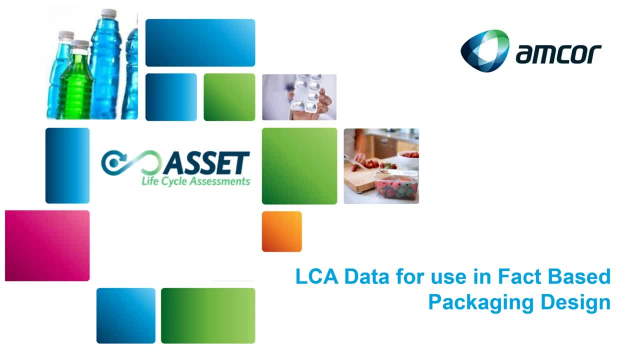 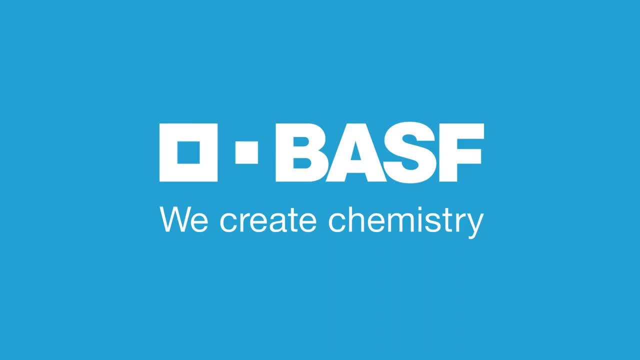 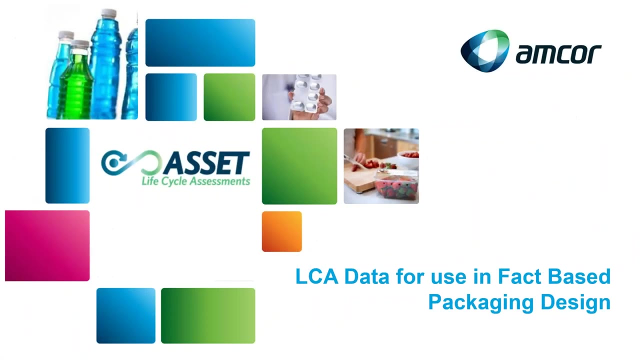 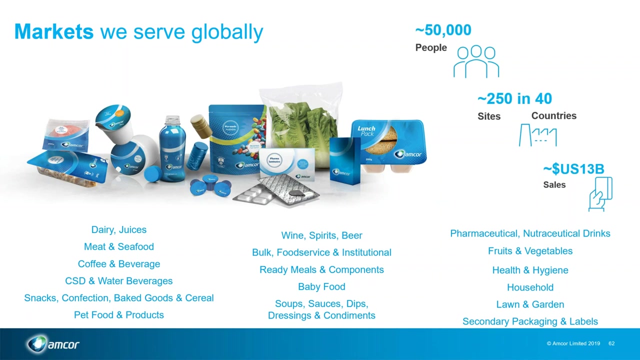 And ours is a little bit more focused on how we use our lifecycle analysis in a tool that we have. It's known as ASPEPT. First, who is Amcor? Amcor is, sorry, very sensitive control here. Amcor is a consumer packaging manufacturer. 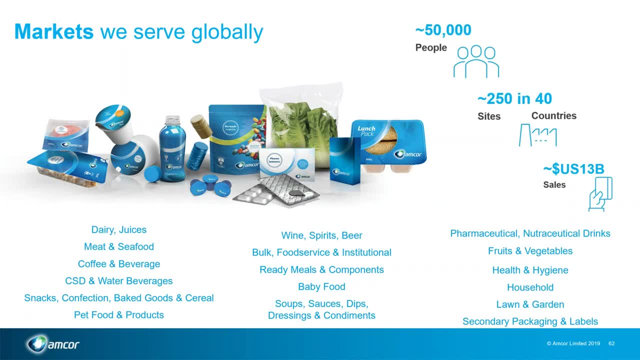 We're a very large company. We're one of the largest packaging manufacturers globally. We have over 50,000 people. We operate in 250 countries. We serve multiple markets in both rigid plastic formats, flexible packaging formats and specialty cartons. our major products: 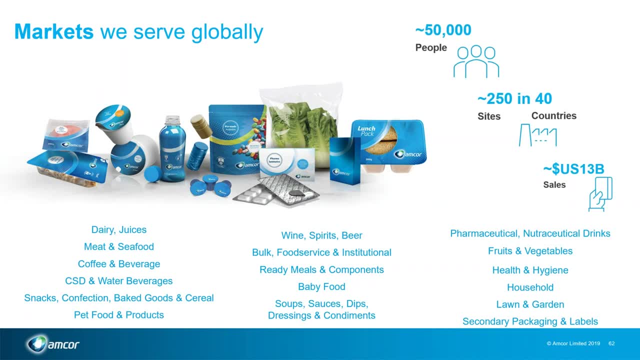 We also produce closures for containers as well. As you can see from the list, we're really servicing food, healthcare, personal care, pharmaceuticals, lawn yard household products. We really have a large bandwidth. We have a large portfolio of products within our portfolio. 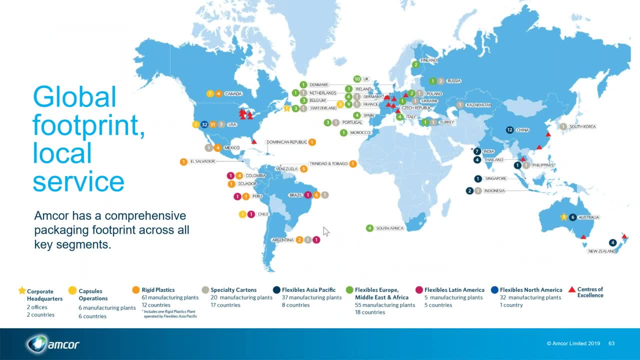 We are a global company And so when I talk about ASPEPT, we're trying to establish ourselves across the globe under multiple different transportation supply sources globally, So it's a very flexible tool within our portfolio, Amcor is very flexible. 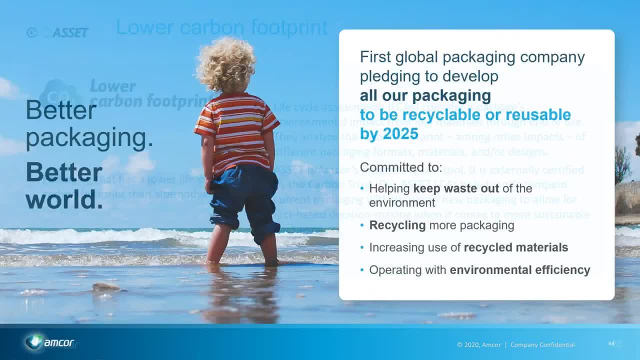 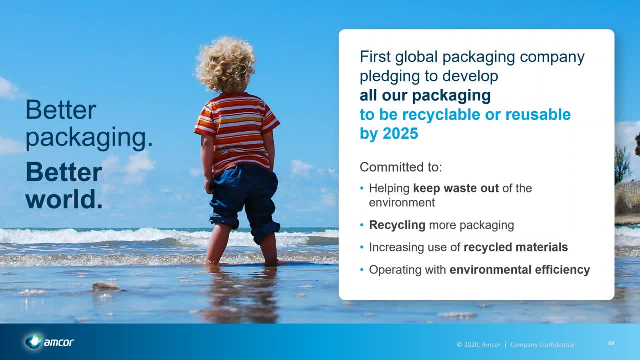 We're the first packaging company to pledge our products to be recyclable or reusable by 2025. And this is a large focus of our efforts in R&D and marketing campaigns to make recyclable packages. So what happens after you've achieved that? 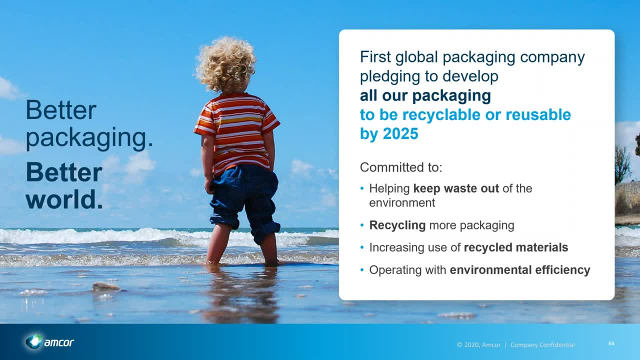 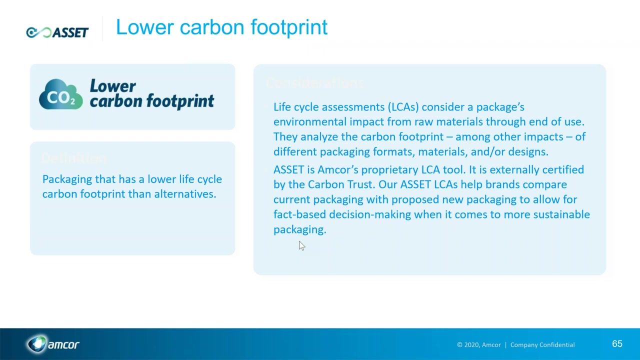 In rigid packaging. almost 97% of our products are considered to be recyclable or recyclable ready, And so, when we look at recyclability as one milestone, we really want to drive into the next milestone, which is the carbon footprint. That's really what we're trying to achieve as a sustainable packaging. 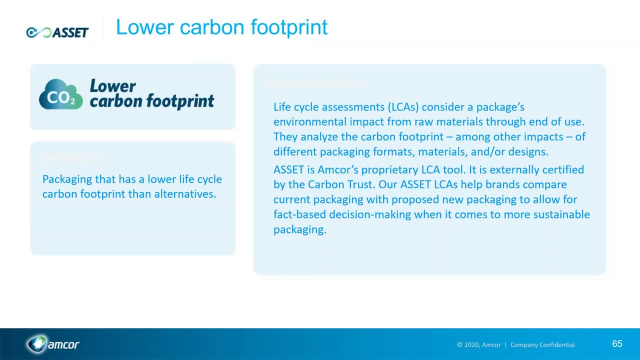 The carbon footprint and recyclability go hand in hand, but an LCA gives us that tool to come back to a package that has the best sustainable footprint and the most sustainable application that we can achieve. So Bruce explained very well what a lifecycle assessment was. 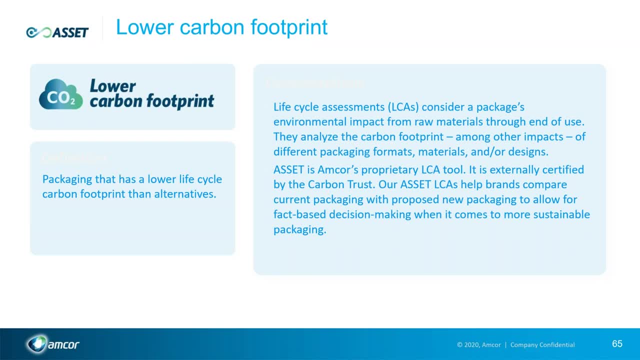 Amcor has a proprietary tool we call Asset, which is our LCA program that we use in the design of packaging and decision-making on how to come up with the best sustainable footprint for one of our customers, And Asset is a certified tool. 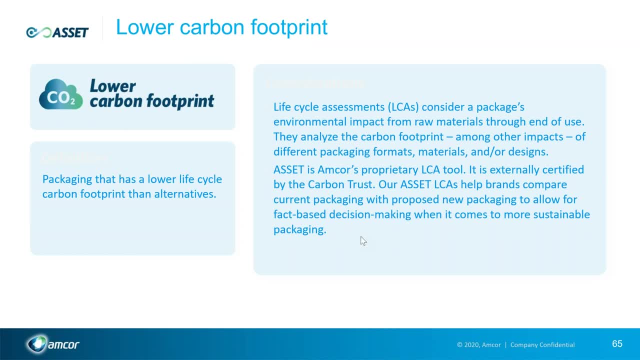 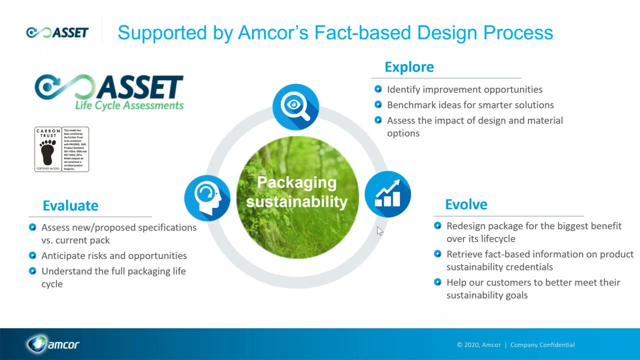 Again, it's a proprietary tool that we've developed for our use. It supports really our fact-based design process. We just don't want to go wrong. We just don't want to go off feelings and perceptions of what materials or transportation give us. 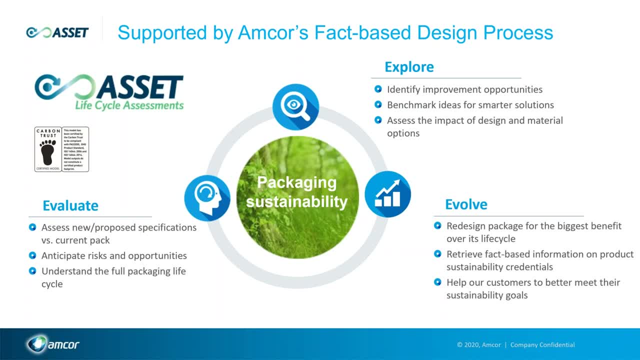 We really want fact-based information, So it helps us evaluate and assess the proposed specifications of the current package And we can anticipate the risks and the opportunities when we're under evaluation of many different formats, And these formats can be both sizes, size offerings. 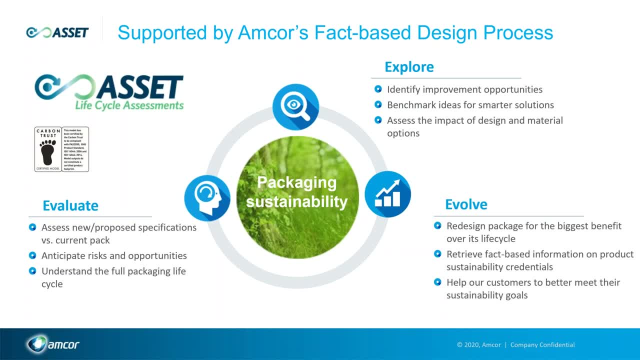 Or they could be a choice of materials. especially in flexible films where you have multiple materials making up a package, The choices between those packages are not apparent. Bruce gave a few examples of those, And so the Asset lifecycle assessments give us that really fact-based evaluation process of which materials would be favorable and which processes will be favorable, as that adds energy. 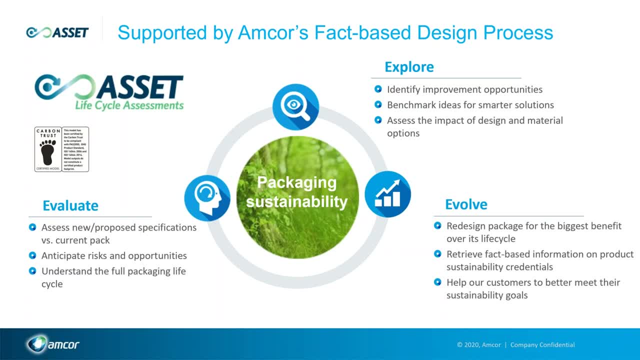 And it helps us explore. And it helps us explore the different opportunities and really benchmark the smarter solutions of what we're going to offer our customers And we can evolve that packaging. We can make rapid decisions and rapid redesigns and packaging knowing we're always moving in the right direction for sustainable solutions. 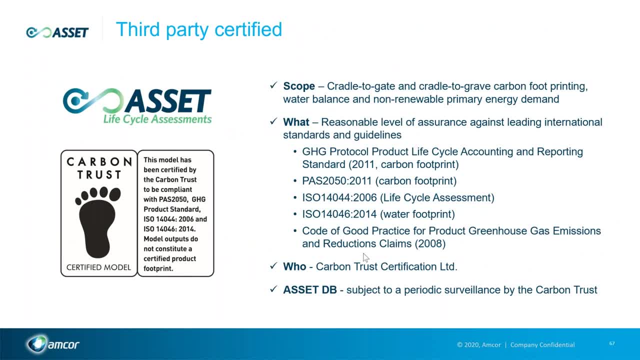 So Asset is a third-party tool And it's not just a product, It's a tool, It's a third-party certified program. We follow the same standards that Bruce had mentioned: ISO 14044, 14046 for water And the GHG protocol for product lifecycle accounting and reporting. 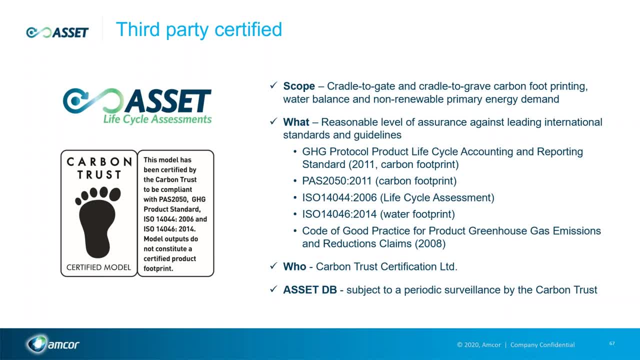 14.040 is really the substantial how-to guide for lifecycle analysis, And Carbon Trust certifies that we're following and we're compliant with these guidelines internationally for our tool. So we really rely on Carbon Trust. Now we're not certifying a product in the sense of a finished package with the product in it. 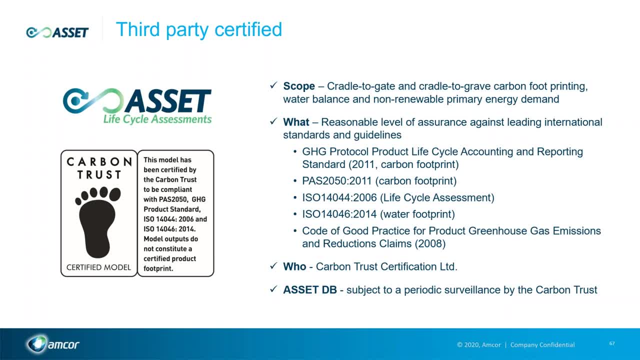 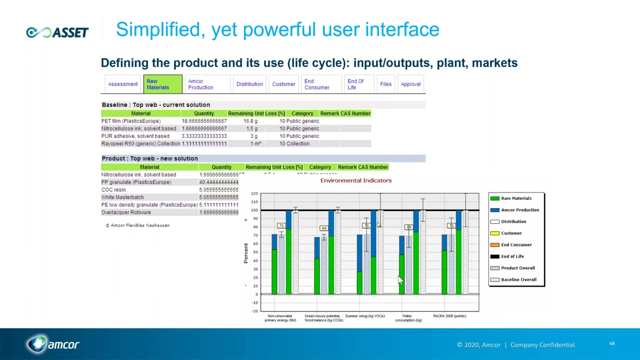 We're really looking at our product. We're looking at the model, the flexible pouch, and what that brings to the contribution. That's really what we're offering our customers and our customers are concerned with in that group. So Carbon Trust gives us that reliance that we're doing it in a method that's acceptable to the ISO standards. 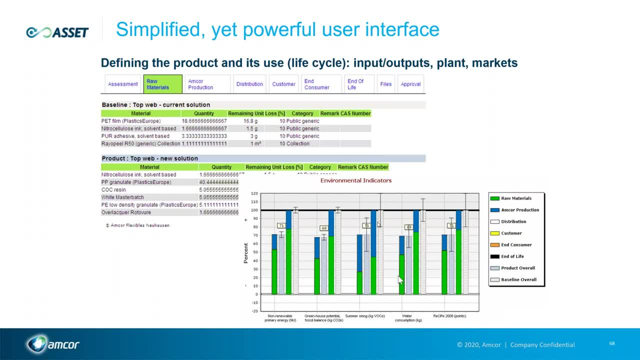 This is a glimpse of what the data looks like. within Asset We have a database with all of the materials that are very common to food packaging or household or packaging that we would sell. All of our standard materials are quantified in greenhouse gas, energy, water usage to manufacture those materials. 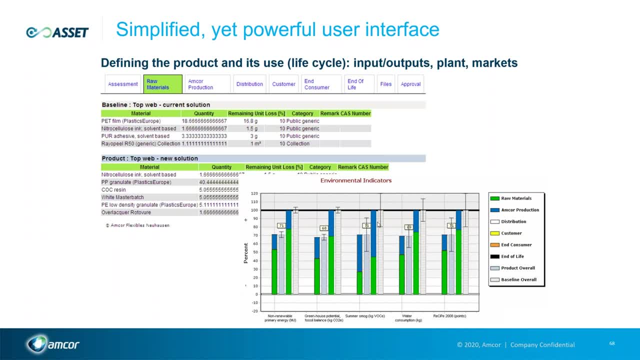 We also add on Amcor's production. We measure our energy use for our production platforms. Within the assessment, we're able to look at distribution in both the sense of transporting materials to one of our sites or from one of our sites distributing it to our customers. 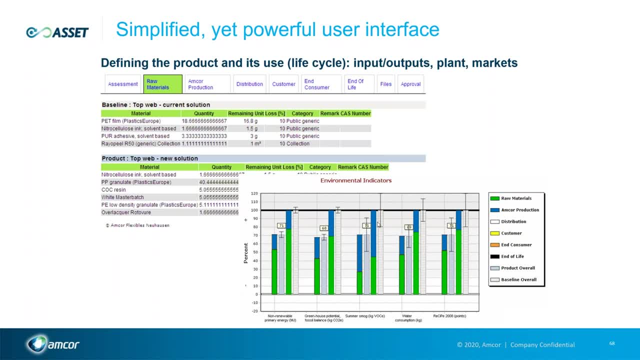 And then the end consumer and end of life, which also add the value. as Bruce explained, If you're going to recover this through recycling- mechanical recycling- or you're going to landfill, or you're going to recover energy from it, Asset takes that all into account as selections for your end of life. 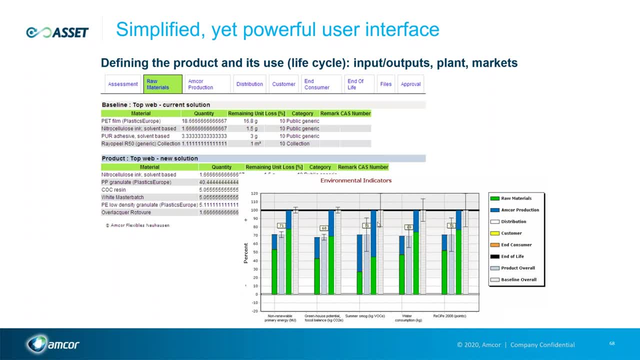 So not only do we have the materials to choose from, but we know how we're going to bring material back or at least recoup some type of energy for those solutions. And this data is updated on an annual basis, So we're always trying to pick out. 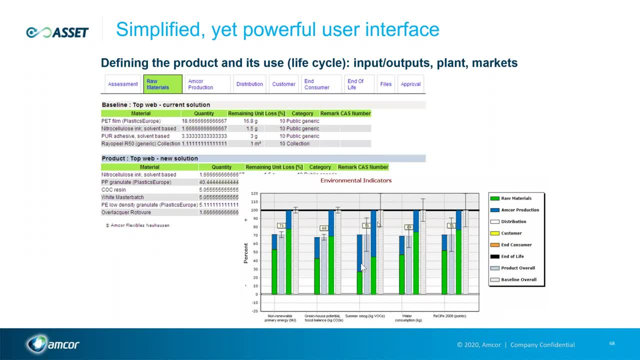 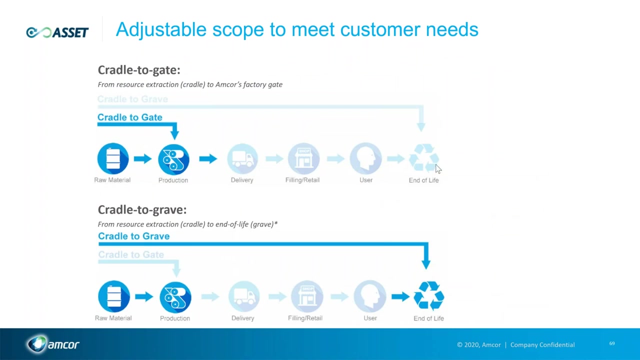 The latest information so we can keep our program up to date. And again, we're following the ISO standards of 14.040 and 44 for this assessment. I'm sorry, We can make choices on the scope, same as Bruce had mentioned. 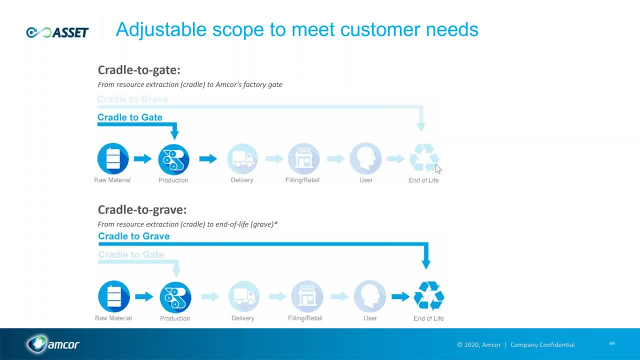 We can go cradle to great date Or we can go cradle to grave, And most of the time in flexible packaging or rigid packaging for consumer goods, the materials have a significant amount of influence on the lifecycle analysis, So we often look at cradle to gate. 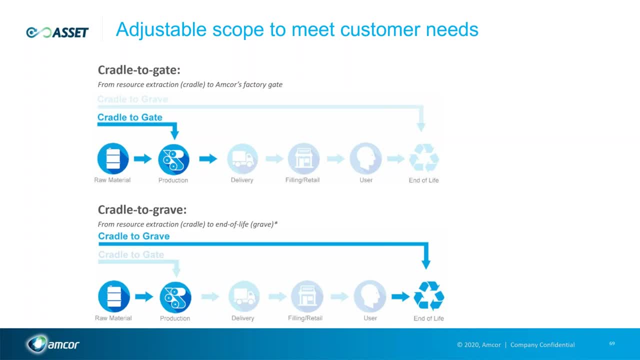 And that's our biggest impact. While delivery and end of life do bring back a certain amount of energy, end of life do bring back a certain amount of information or a certain amount of influence on the product. the materials are the significant influence. This cradle to gate. looking at materials and production energies. 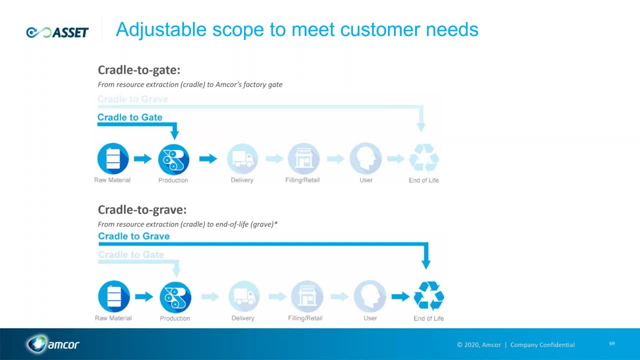 gives us a real rapid feedback to drill down on the one or the two selections that we're going to be making. And then, when we get down to the one and two, then we'll do an entire lifecycle analysis and capture all of the energy and all of the emissions that may come with the package. 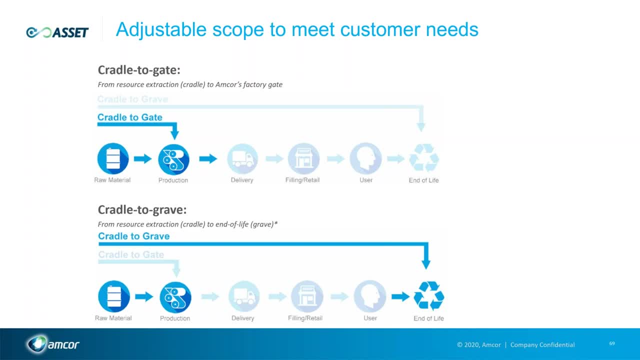 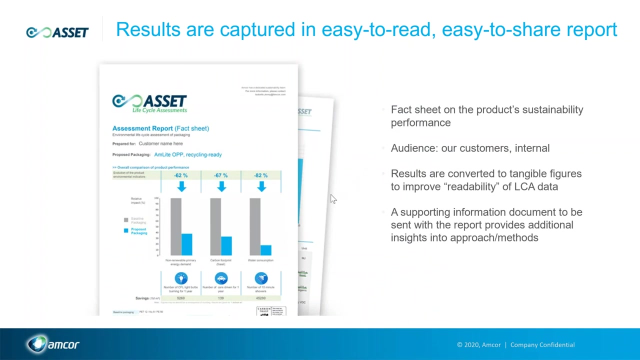 So the cradle to the gate and the flexibility of this gives us a really rapid turnaround within that lifecycle. Our reporting comes out in a very simple fashion. We're comparing the percentage of the materials as they compare one with the other one, So we can see the significance of the material and energy. 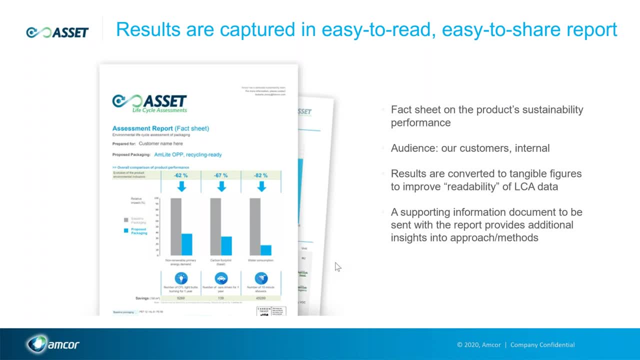 And then it also puts it into a tangible – one of the things that we see and one of the feedback items that we see from our customers is they don't really know how to scale greenhouse gas. What does a ton really mean? So we use the simple approach of the EPA calculator: comparison calculator. 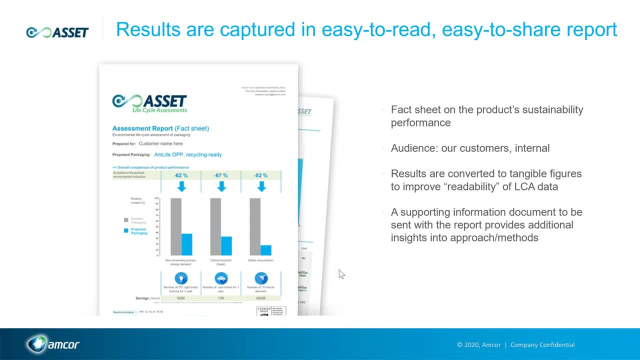 and you can easily see how many light bulbs or cars, or something that's measurable- from a substantial population, what's measurable, what's understandable, what these savings really are, And that also gives us a feel of how far we're moving the needle in those cases. 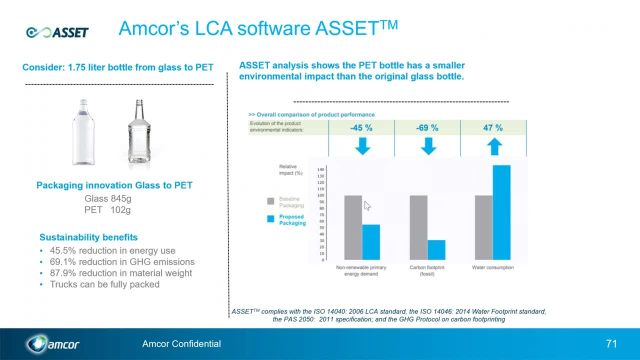 So when we look at an assessment, this is an assessment of comparing a plastic bottle to a glass bottle- And if we just look at the material, glass, one gram of glass has a significantly improved sustainable carbon footprint compared to one gram of plastic. 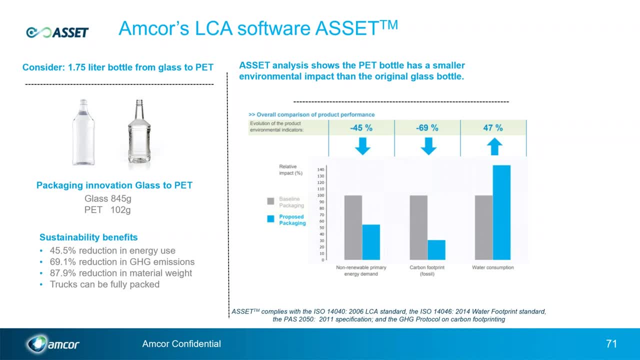 But that's not comparable in a package size. What we see in a package is that PET – and this is a spirits example – of a spirits bottle at 1.7 liters of relatively large bottles, we would use about eight times less material and weight glass compared to a PET bottle. 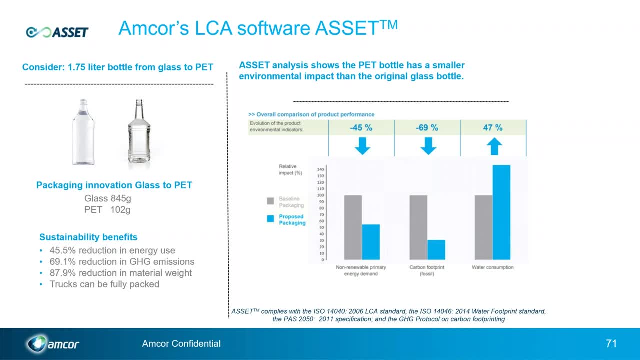 So we'd have 845 grams versus 102.. And what we see there is we'll have a 45 percent reduction in energy use, a 69 percent reduction in greenhouse gas emissions, And we're saving a significant amount of material In glass comparisons. 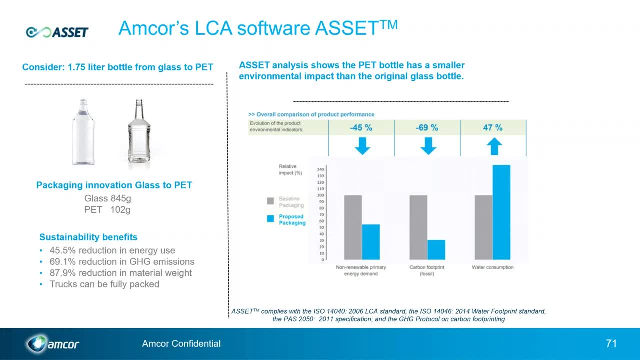 transportation becomes significant because the glass weight is heavy and typically you don't cube out a truck, where in a plastic bottle at much lighter weight you would cube out a truck. So in this example we would have a very favorable transportation weight. Now glass is favorable in water consumption. 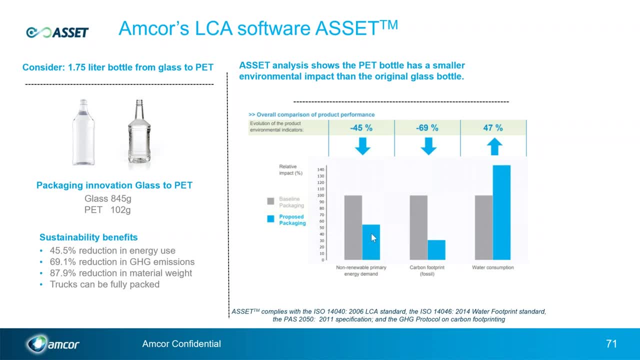 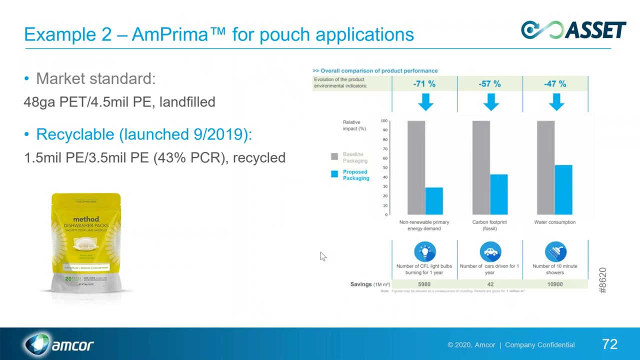 So, depending on a customer's goal, what they want in the greenhouse gas aspect, water is favorable in the glass packaging by almost 47 percent. So now we have data to look at and compare these two containers and material choices for those applications. In the case of a flexible pouch, 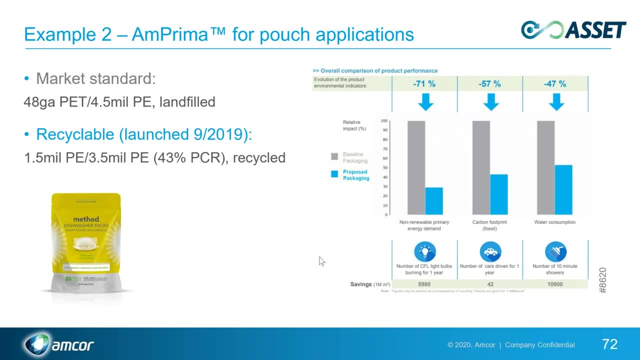 we're looking at a comparison between a laminated material and our new recyclable pouch made of PE laminates and 43 percent PCR. Standard packaging typically has a print film: 48 gauge PET laminated to PE. This is a landfill product. 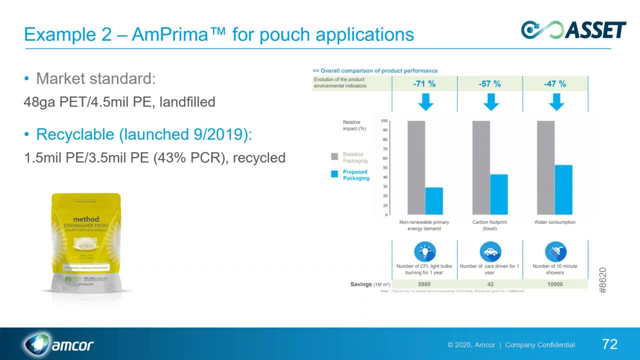 This really can't be recovered under mechanical recycling as exists today, But a full polyethylene pouch can be recycled. So here we're capturing material change in the same package footprint and we're recycling and capturing PCR back in the product, And in doing that we save 71 percent greenhouse gas. 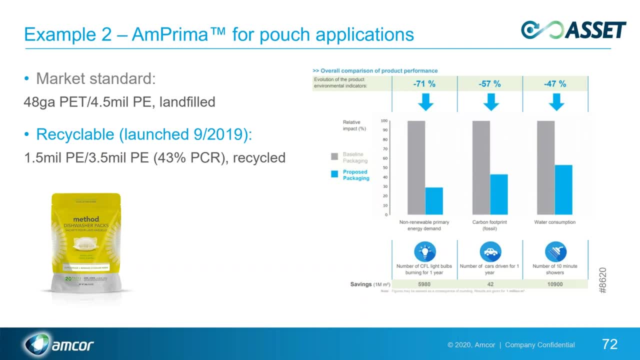 and that's the equivalent of almost 6,000 CFL light bulbs, according to the calculator. So we have a measurement, We have a reduction And then we have a feel for what is that in significance in people's minds. Carbon footprint using fossil fuels with savings of 57 percent. 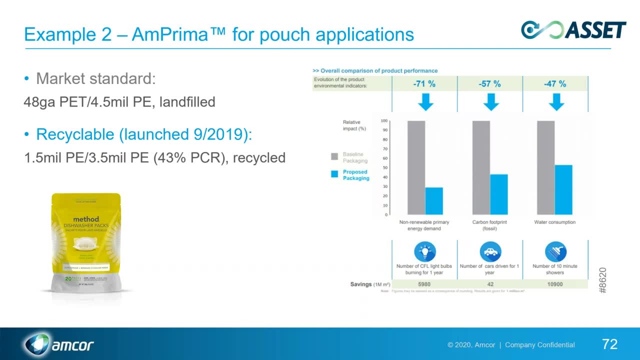 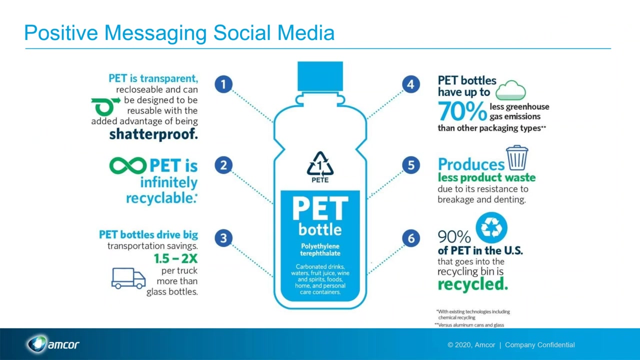 and 47 percent water consumption savings. So again, we're driving down to real data to make decisions. Is this a better package? And clearly in this example, a recyclable pouch is an advantage over a standard pouch. We also use this in marketing messaging. 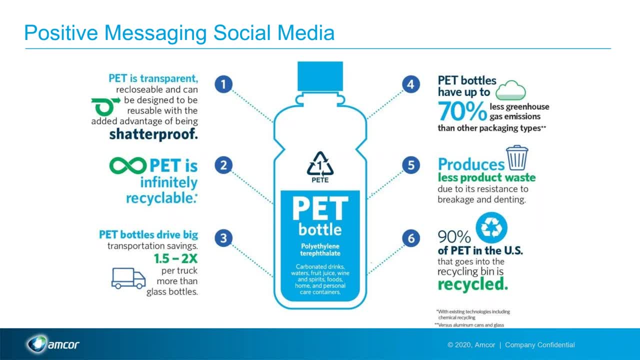 We typically are challenged with the plastic waste scenarios, but plastic has a significant greenhouse gas benefit compared to other packaging styles and packaging parts. So we try to always use third-party data when we make our messaging, but we can use the lifecycle analysis To verify that data or give us direction on what data to pull out. 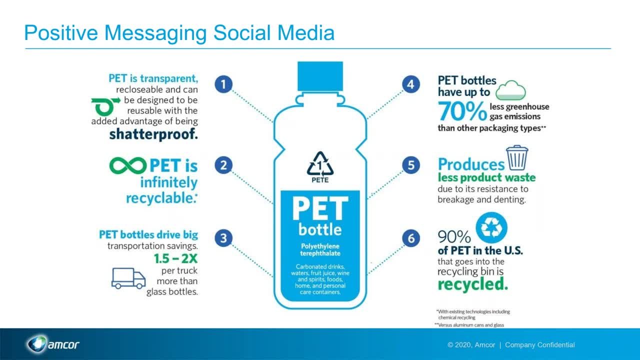 So in our positive messaging schemes for PET bottles, LCAs are used to bring back that data and make the right claims and really give direction of what a good packaging, sustainable packaging option is to a consumer. So not only is this used for our customers' benefits, 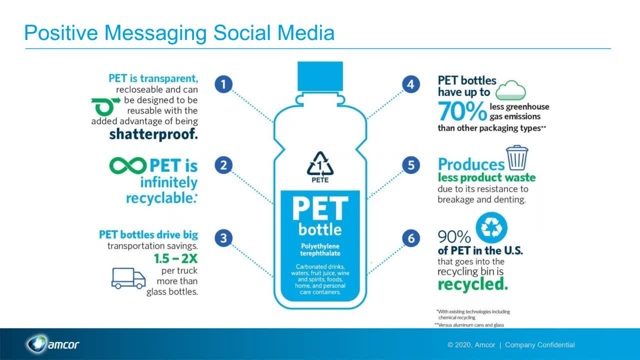 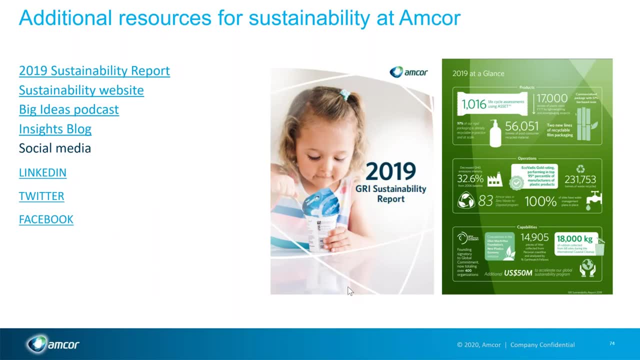 our design benefits, but also our marketing benefits. So AMCOR has, sorry, skipped one too many here. AMCOR has a very strong sustainability program. We offer- and I offer hyperlinks to our reports, our websites, our Big Ideas- podcasts. 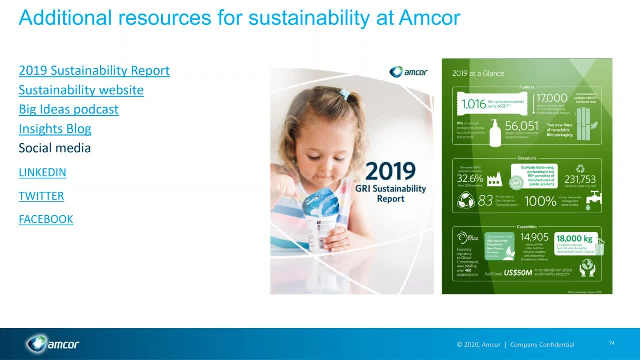 All can be reached on the AMCOR website if you'd like to know more, or you can contact me. So, Ashley, I'll turn it back to you. Excellent, excellent presentation, Dennis. Thank you so much. I love how you guys have taken all of the 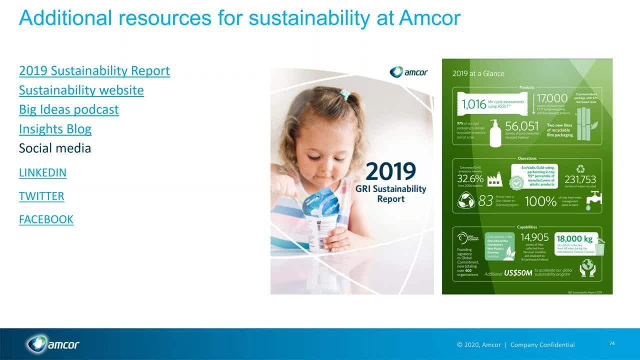 you know the science and the facts and turn that into you know you. you both boiled it down to you know the reporting styles, but also into just a very, very simple infographic. So thank you so much, Thank you. 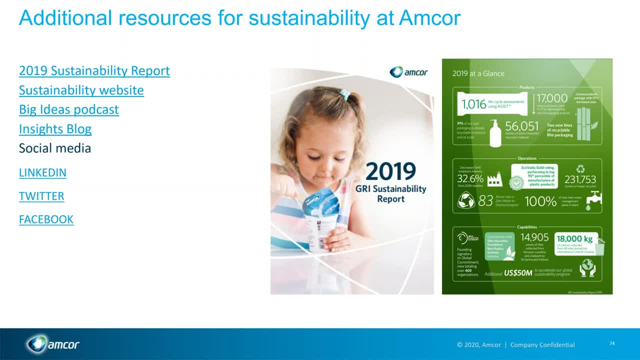 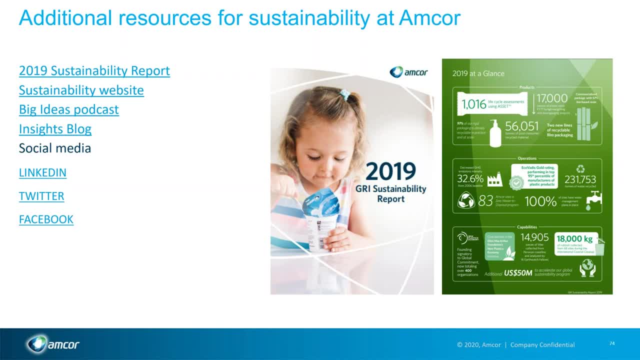 what that means and what you guys have done. So thank you so much for that example. So I will now take a quick look. So I'm going to hold on this slide for a minute and take a quick look at the questions that have come in. 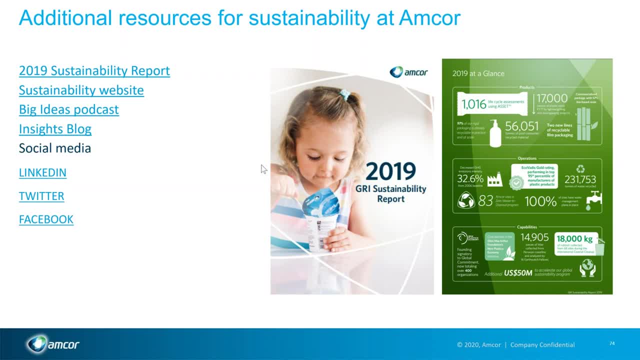 So again, if you guys haven't sent in your questions, um, send in your questions yet and have one, please feel free to send those in. so, um, let me see what we have. okay, so this one, i think, is directed. this came in during um, during bruce's uh presentation. 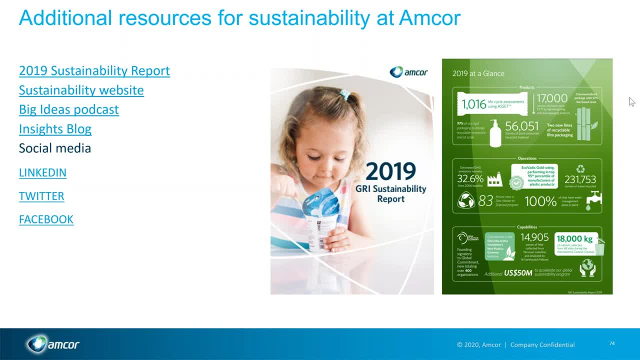 so, oops, apologies, let me uh re-pop that question, okay. okay, this came in during bruce's presentation, so i think it's directed um towards him, but probably something that both can answer. so i'll let you guys um, we'll start with bruce and then dennis. feel free to chime in. so the question. 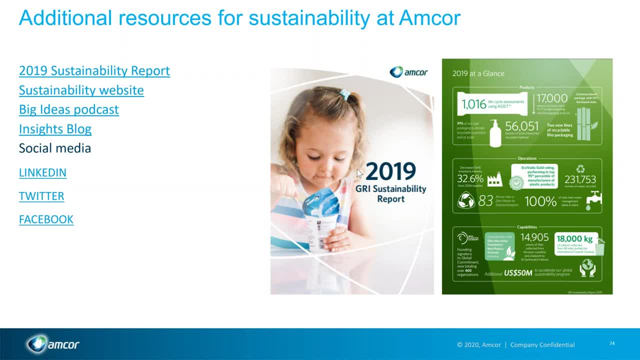 reads: when you consider an lca where one option is a method that uses assets like a hand dryer and the other is a disposable product, how do you really compare them? do you compare over the likely useful life of the asset? so, bruce, i don't know if you want to take a stab at that first. 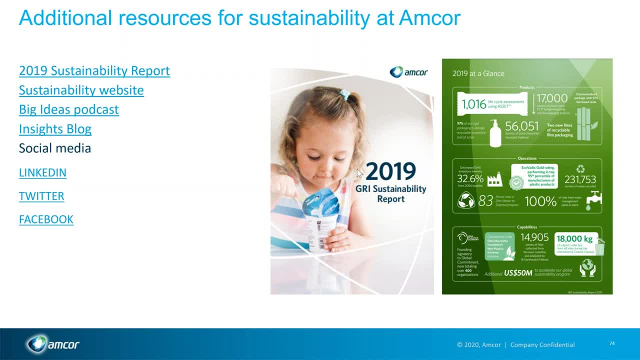 yes, exactly yeah. so that is one of the key aspects of, you know, when you set up in that goal and scope, part of defining that functional unit, which must also include aspects around durability. so you don't want to take just like one instantaneous drying of the hands, but you want to. 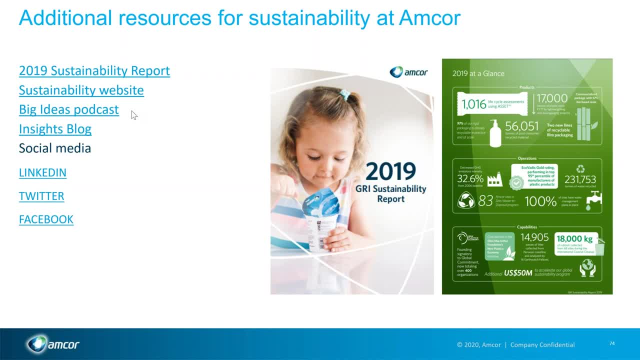 consider durability, so it could be over a period of time. for the hand drying one it was a thousand hand dryers but when you look at the functionality, the hand dryer that may last for five years. you may want to include that into the life cycle assessment. so you're including the full. 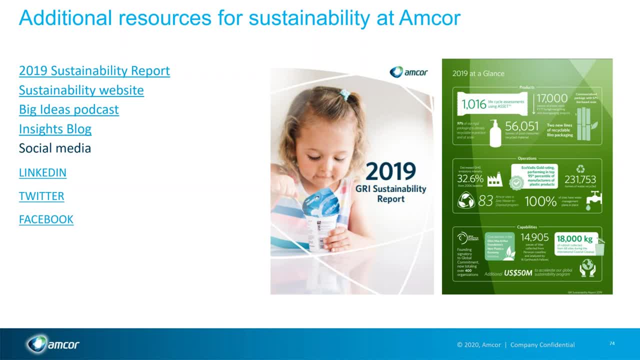 durability of those items, similar to the incontinence pads which could last for, say, so many uses. you want to make sure that the durability of those items are being, the benefits of that are being fully reflected in that functional unit and the scope of your study there. so, yes, durability. 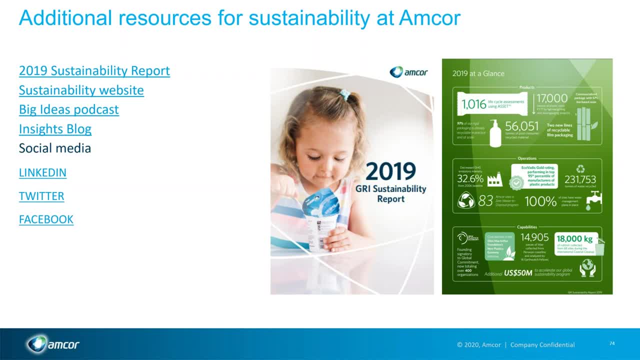 the lifespan of the lca is a very important aspect to include when you're comparing different alternatives to this model. but i think the next step would be to add additional components to the concept of the lca and thinking about that in more detail, and that's why we've been so. 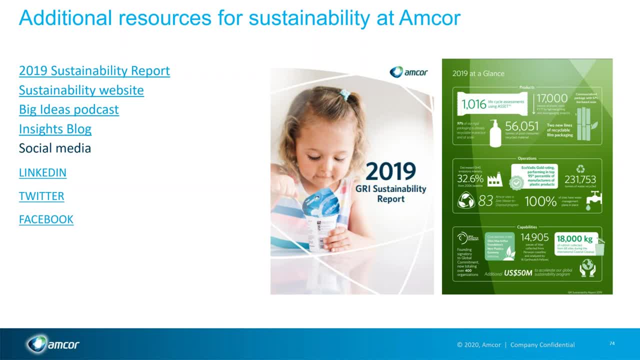 focused on this kind of in the past to help us really make sure that we have the best possible application and the best possible solution to achieve that goal in the long term. perfect, thank you, i don't know. i don't know if i can add anything to that. we i would agree with. 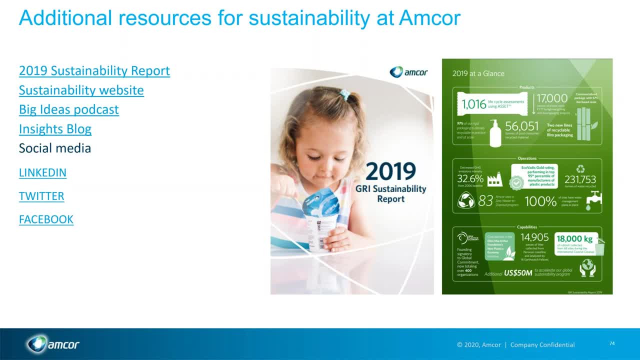 that 100 um. part of our challenge, uh is that this space changes rapidly of time as we see better recovery systems, better technology and recovery, more efficient recovery. there's large efforts in there, so one of the things I would say is that, if you look at this in a space of time, keep track of some of 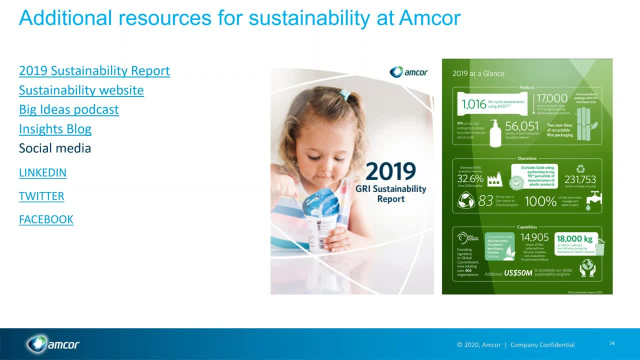 these influences that continue to evolve, because, if it's close, you might see the scales start tipping in the next year as technology helps recycling and end-of-life decision-making and end-of-life data. yes, no, excellent, excellent points from both of you. let's see what else we have. 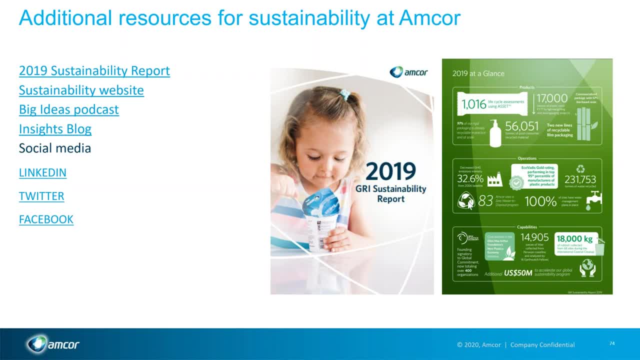 we have a lot, so what? let me try to pick one. let's see. okay, somebody has that is asking the question and just want to re-emphasize that. yes, we have recorded this, this webinar, and we're happy to make that available to anyone who helps us answer our survey. 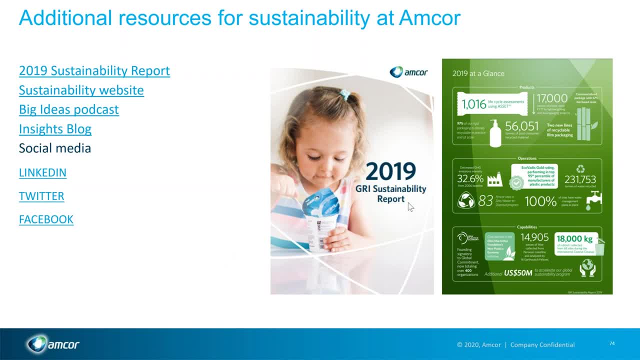 questions at the end, okay, so let's see who else has come in. so a couple of questions, and these are for both of you guys, a couple of general questions about you know- and I get these questions a lot kind of as a point person at Plastics. 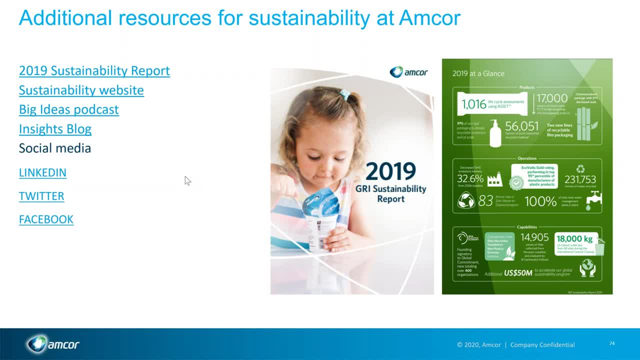 for materials and and sustainability and um folks are really interested in and and what i'll let you guys share with what resources you know that are available. folks are asking about what: are there good studies that exist um using lca that compare various materials, and so, specifically, this person. 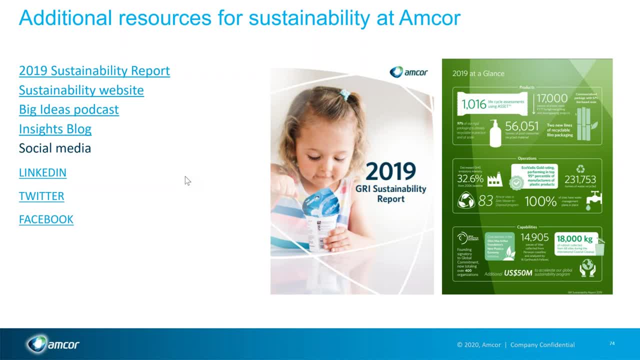 has asked you know comparing hdpe, pet, paperboard, aluminum and glass? and then the second kind of similar but different question is: are there good studies and reports out there looking at mechanical versus chemical recycling um holistically? so i'll let you guys chime in um on on what you know is available. 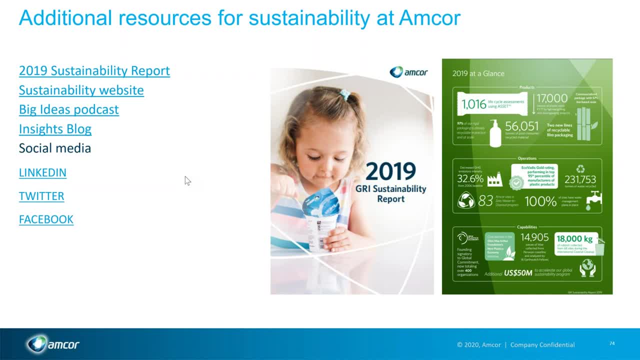 yes, sorry i'll, i'll take the first part of that. as far as um good studies comparing different packaging formats, uh, i would say you really need to dig into the details, and i think this is the value of setting up your own study of based on your goals. so my answer is tending to know i see too many. 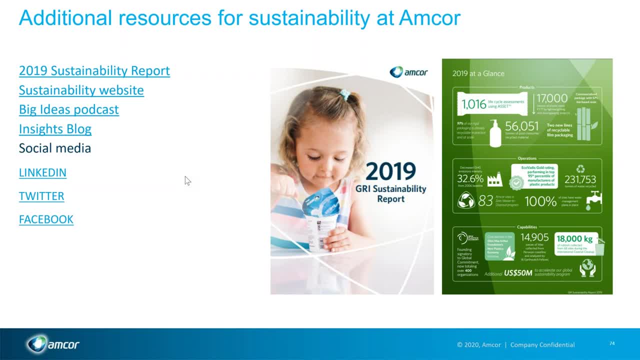 influences. i see too many trade associations- the aluminum trade association- putting the lca in their scope, definitions or the paper board and and i'll say a little bit more about that in just a few minutes and then i'll let you guys go ahead and answer your questions. and then i'll let you guys go ahead and answer some of the questions. 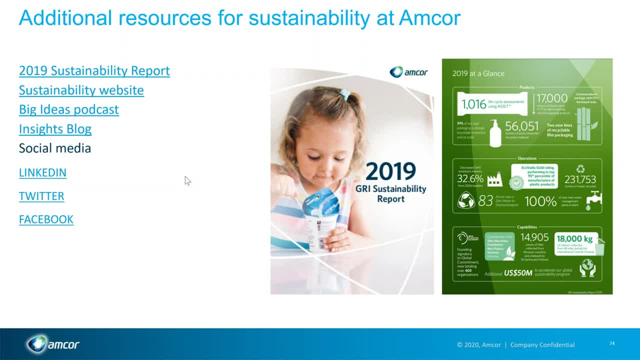 and then i'll let you guys go ahead and answer some of the questions. so i would really approach the studies i've seen out there with some skepticism because of that scope setup of what they want to compare. i've seen glass just be very, very favorable to plastics because it's compared on a gram basis, not on a packaging basis, and so your 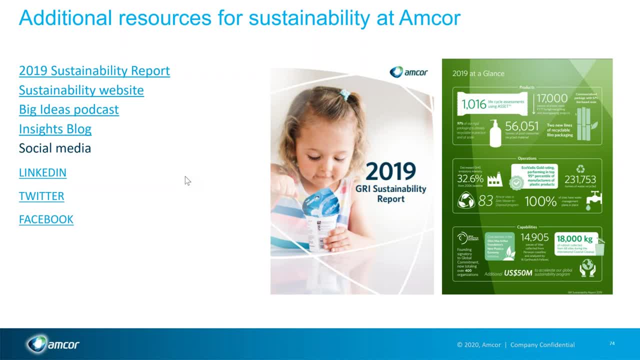 packaging typically is unique to your application, your size, your weight, your your goals of what you want that packaging to accomplish in its journey from manufacturing to end of life, and the only way to do that is really have your own study completed and that's, in the packaging world, our plastic. 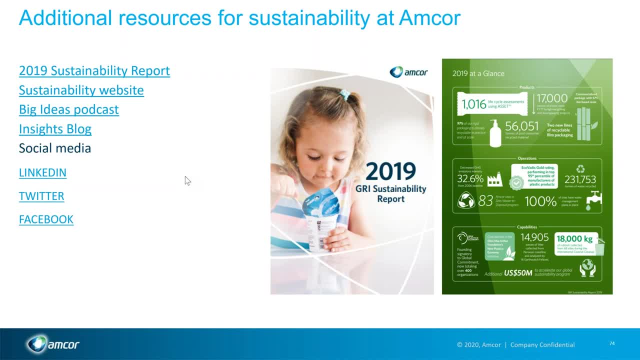 packaging world. that's what asset was made to do, so we could quickly compare one versus another in your goals and your format, your size. you can't just extrapolate what's out there into your your packaging size and weight. bruce, yeah, i think that was a great explanation there. just highlighting two points is that: 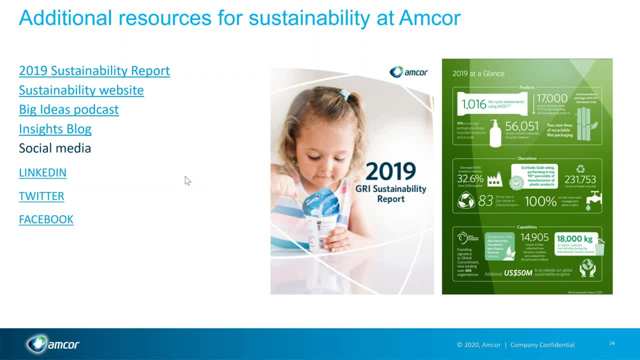 you know, though, you can do some comparisons. you know cradle to gate of, you know, perhaps, a kilogram or a pound of material. it's very dangerous in that you really need to look in the use and the application- is what dennis had mentioned there- into the packaging application, because there you look at comparing. 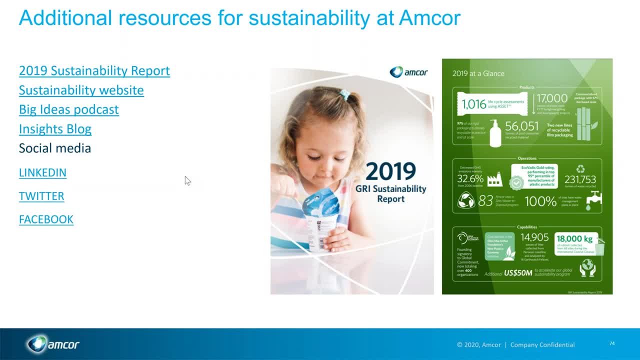 functionality and performance attributes. you look at longevity of certain aspects, which you heard in the first question there, so you're not just comparing a pound versus a pound. you need to look at better understanding of the technical performance attributes, end of life options and it is very specific on the application. 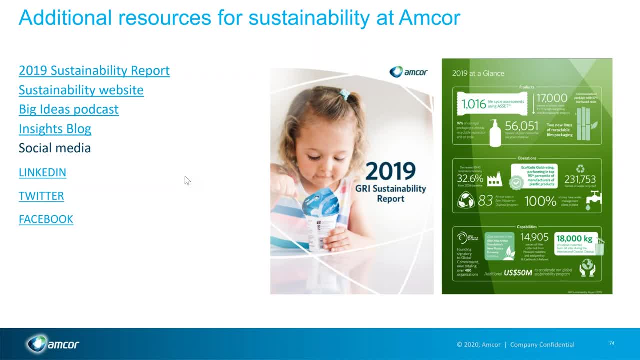 or on the application and so on. in the second part of that is start with the engineering, other applications. i think the customer experience is more important because we have a lot of different programs who are competing against each other, whether it's a drug or a chemical that's organically produced or anything that's a chemical in. 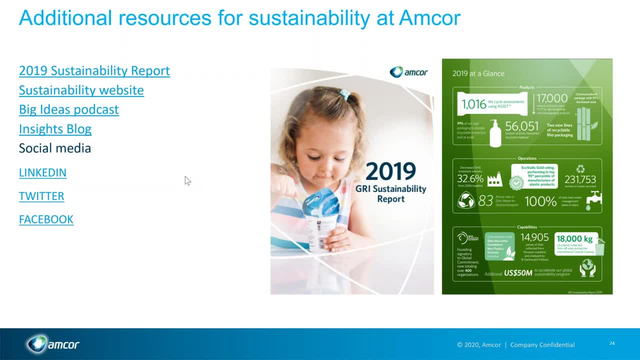 the product, or you can. you can not- use a chemical in a product of literature out there. the International Journal of LCA has good case studies and even companies post a lot of their reports out there, which is good for getting a general understanding and awareness of hot spots and drivers. 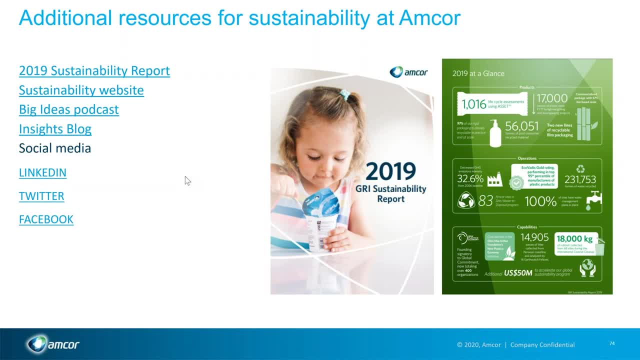 within value chains. but to really make credible decision-making you really need to internalize that, as Dennis said, to your specific product, your specific manufacturing and supply chain and then, with your customers, application and what those end-of-life options are reasonably going to be. so you need to go. 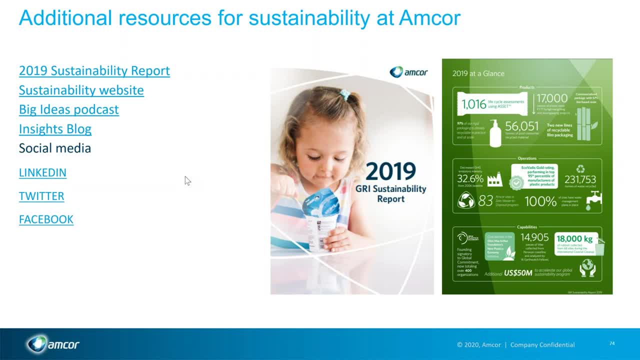 case-by-case to really inform decision. but I think a lot of the studies out there do help inform lifecycle awareness and thinking of hot spots and value chain drivers. excellent, thank you, go ahead. and there was a yeah. a second part of that question was mechanical versus chemical recycling. I think today is one of the 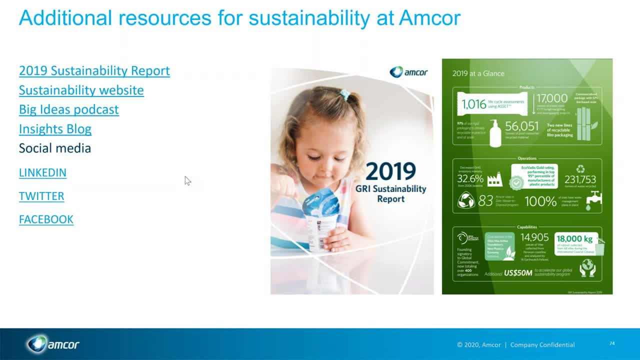 first times I've seen a very substantial looking at that with Bruce's analysis. chemical is emerging. it's not always at scale. so we're seeing some projected LC a's on chemical recycling, but this is emerging and there's more to come. so we don't. we don't have a wealth of information and 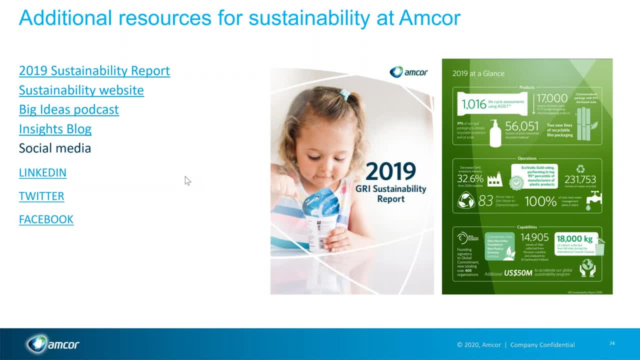 LC a's, with all of the different chemical recycling methods that are out there today, and to that point there is a link in my slide deck there for further information on the LCA that was done for our chem cycling technology and the LCA that was done, perfect. and while we're on that topic, I have a very similar well a. 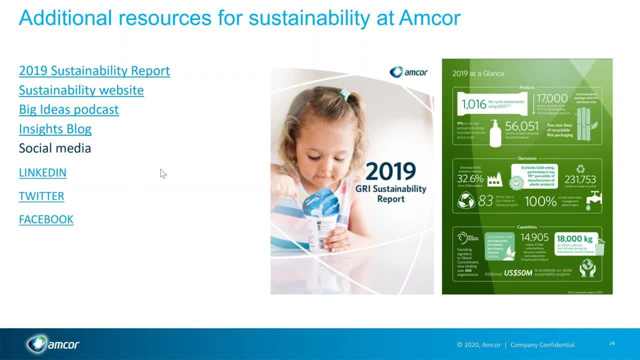 question that's in that same, in that same regard. so- and this may be something, Bruce, that's answered via the Q&A session, but I wanted to go back to that question a little bit and I would like to go back to my question- of the analysis that you have- and I know we 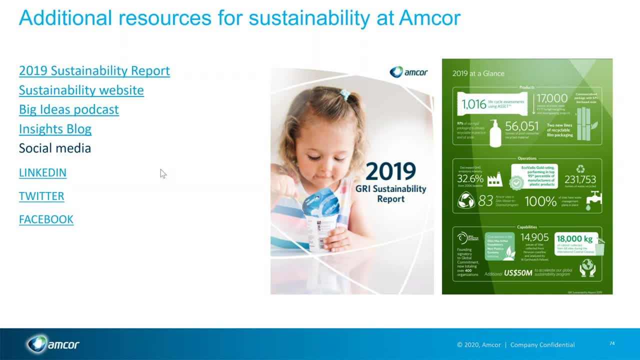 talked about that a little bit, but I just wanted to say that the analysis that you did on the LCA was really effective and I think it was a very helpful way to identify what was the problem with the analysis, and I think that was a great answer and I'm glad that you shared that. and just on that, 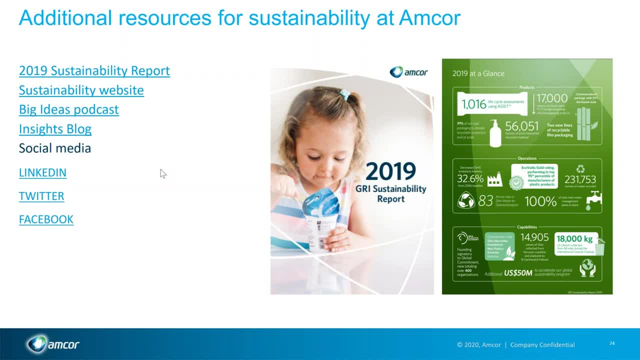 note. I wanted to ask if there were any other questions that came in. you know that report, that's out there, but just have a couple of folks on on the webinar on the input streams there. yes, I think- and I may be quoting it incorrect- but they used a. the study was done and overseen by our colleagues over in. 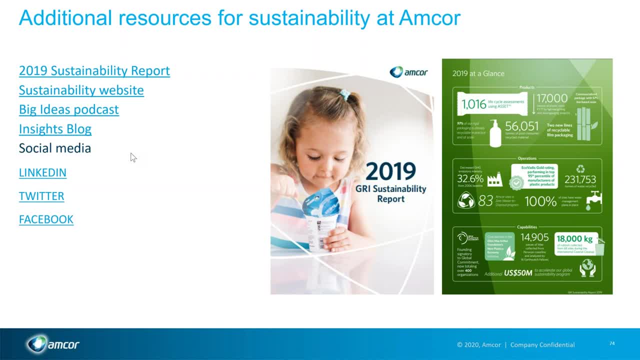 Germany. so I think there was a typical. maybe they called a yellow bag of mixed plastic waste that was used as the makeup for that plastic. I guess that went into the sorting and the assessment for the generation of the pyrolysis oil. but all that is spelled out in that link there which takes you to the LCA. 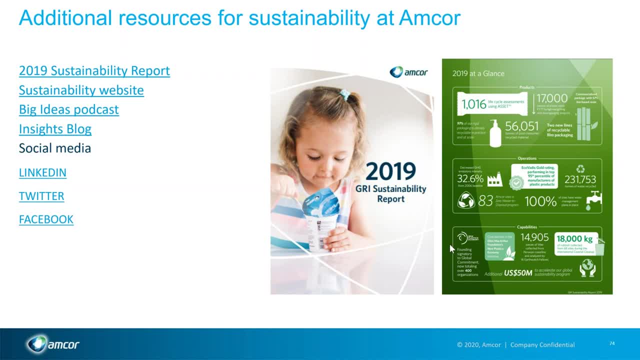 report. perfect, okay. okay, here's a couple of questions for both of you. so a general question: do you use different data sets based on geographical location? so I'll punt to Dennis first on that one. yes, transportation is a big as a big influence on bulk purchases of plastics. also, the manufacturing sites, energy use. 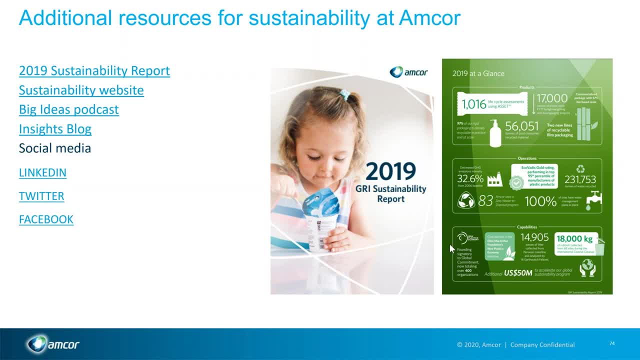 there's some very favorable energy areas of the country and world. so the energy methods of making materials all play into the LCA. so we have PET, for example, US based Europe based in Asia's, space based LC a's and cry or materials. we would go geographically okay and 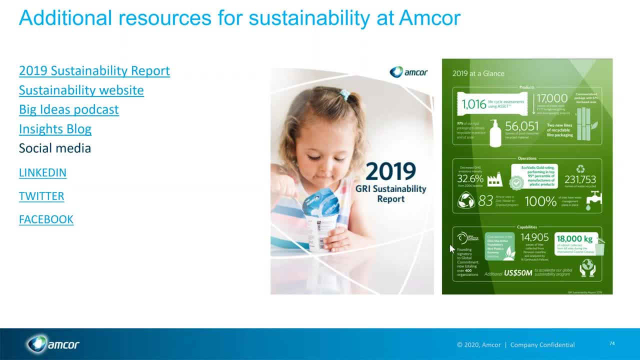 Bruce, would you? would you echo some of the same or have anything to add there? yes, absolutely. you need to have the specificity of that specific manufacturing plan on in. the inherent efficiencies of that plan are כ perhaps the regional electricity grids that are being used and what end-of-life disposal mechanisms are available there. 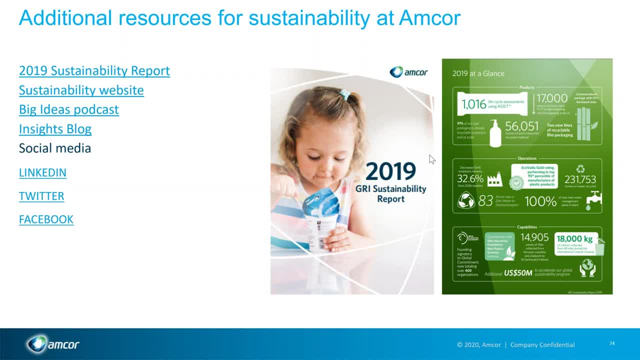 So, yes, so when we work with our customers, we try to give them very plant-specific, you know primary data-generated lifecycle inventory data so that they know that we're not just using necessarily proxy data or you know other information, but they're getting the most accurate data to help. really that what LCA is doing. 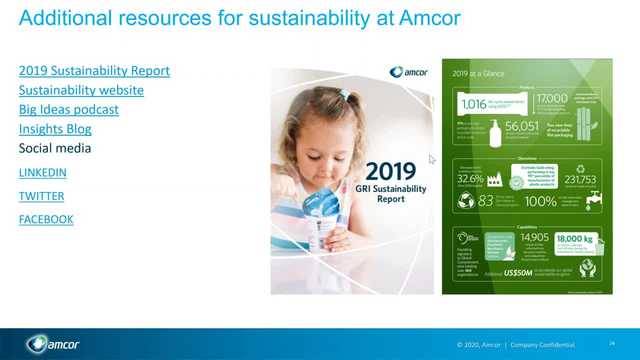 having informed decision-making and understanding the regional specificity of environmental impacts and logistics, as Dennis pointed out, that really help them really innovate and make the best decisions for their solutions. Perfect, And I think you know, as I'm continuing to try to read all the different questions. 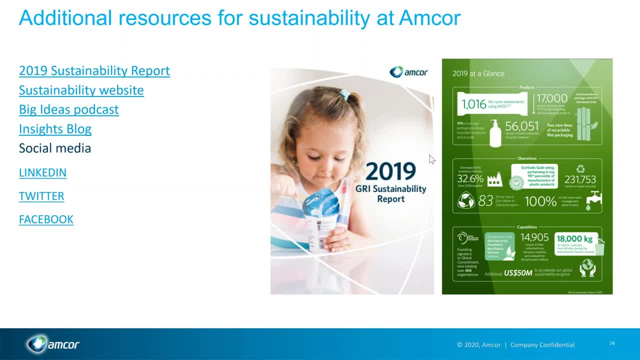 I think we've answered a couple from folks that have another one in here that asked about factoring in local impacts and cited water as an example of something that would you know, have certainly more of a significant impact depending on what region that you're in. 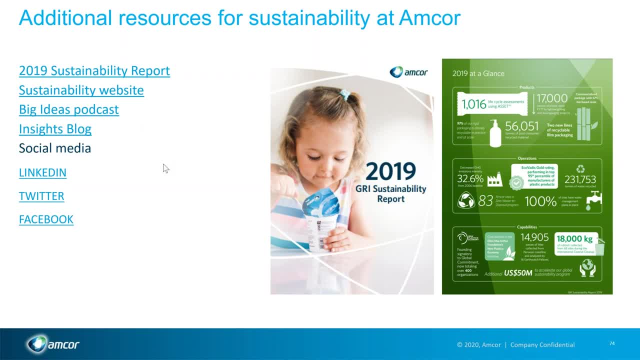 Okay, let's see. So there's another question that's come in, and I think this came in during the time. I think this was targeted towards Dennis and I think I can probably answer this, but I'll let you answer it, Dennis. 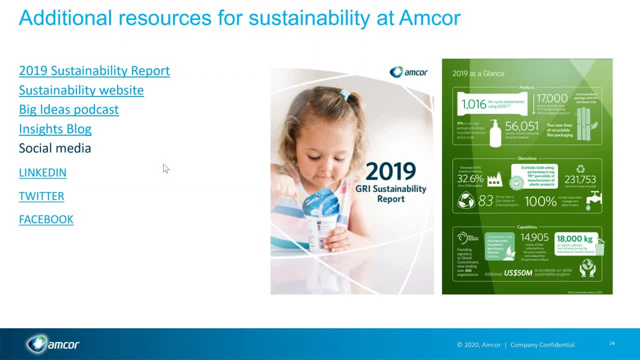 So you mentioned recyclability as a goal. Do you also have targets for recycled content? Yes, we do. We want to significantly increase the recycled content, And PCR is a fantastic way to lower greenhouse gas in the LCA sense. There was a previous question on LCA's comparing packaging types, if there's any good ones out there. 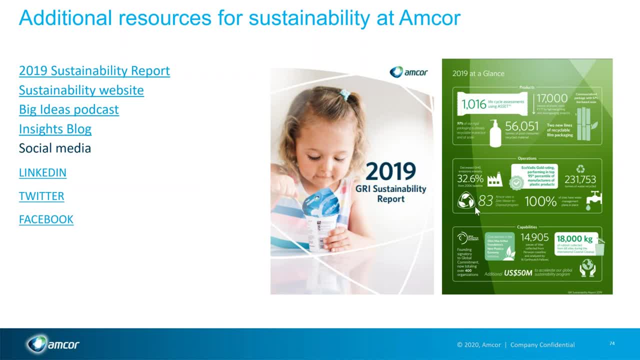 Both NAPCOR and ARP released a 2018 study on materials showing PCR is. it's a little less than half the greenhouse gas impact, So it's a great way to get greenhouse gas reduction and also circular economy for plastic packaging. 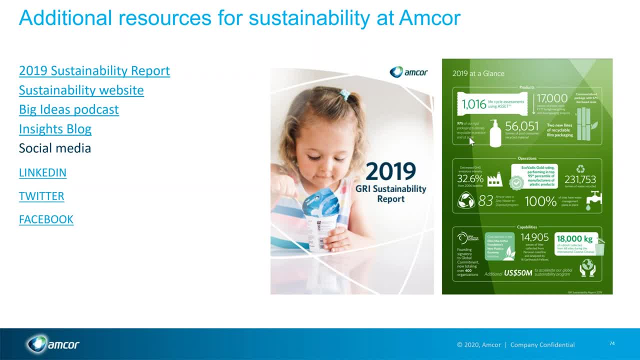 So the 2025 goal is to use more PCR and our goal is 25% through our portfolio by 2025. Perfect, Thank you for that, Bruce. this is a question directed towards you. Is there anything more that you can tell us about the status of ChemStockling? 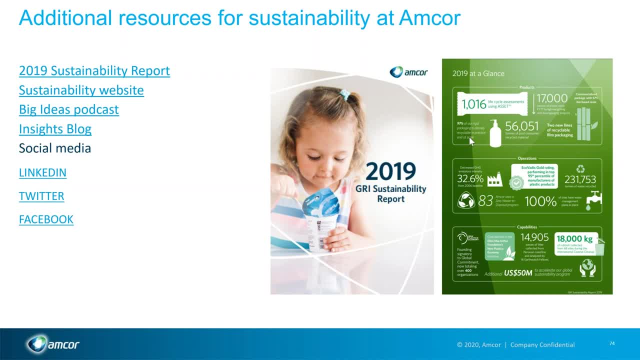 Is it fully operational or still in the testing phase? Yeah, we're piloting with a few of our customers currently with the use of the pyrolysis oil and the products that we produce from that. Yeah, we're piloting with a few of our customers currently with the use of the pyrolysis oil and the products that we produce from that. 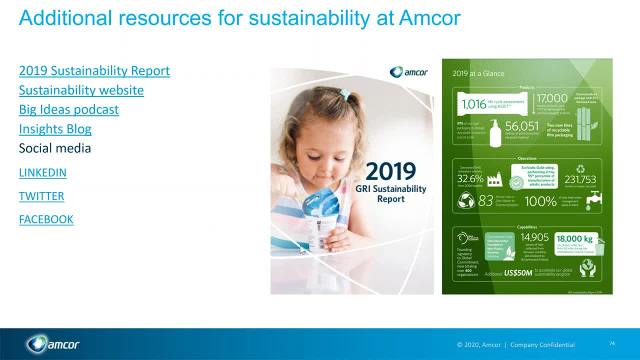 So, yes, it is on a smaller scale, It hasn't yet been scaled up But, no, it is currently in with a few of our customers in the piloting where they're taking our materials that are produced from the spiral oil and seeing the performance and, you know, understanding what those environmental and sustainability benefits of using that solution are, which is obviously here supported further from the LCA, where we've actually taken that deep dive. 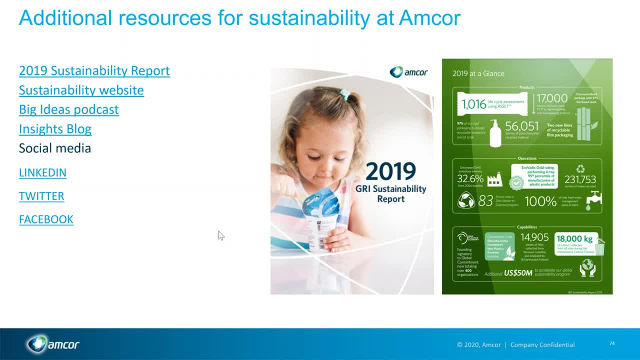 in making sure we fully understand what the impacts are for recovering the plastic waste and converting it into a usable raw material, versus traditional other methods that are available and really using LCA to say in a credible way: yes, it is delivering pure environmental benefits versus these other options there. 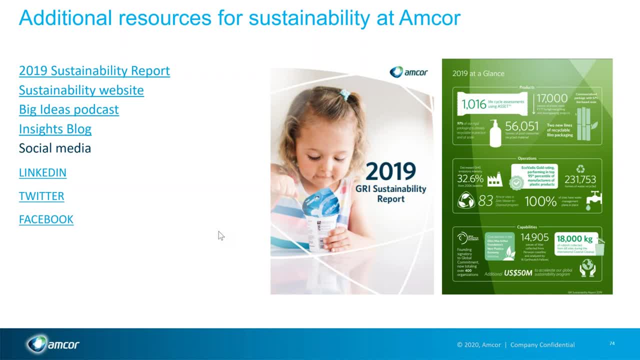 So, yes, we are working with our customers on that- currently Wonderful Thank you. So this is a question that can definitely go to both of you. So, Bruce, I'll start with you and then Dennis chime in, And it's a big question. 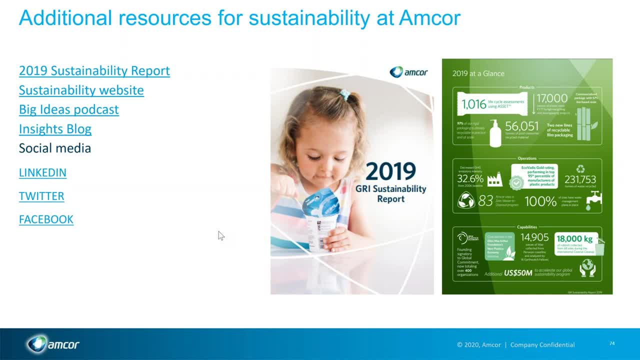 It's a good question. So, to the extent that you can comment on, how do we reconcile the different LCA software tools that might generate different results? Well, I think that goes into- maybe not necessarily the tools, But the data that goes behind them, maybe that's part of it- the databases of the lifecycle profiles of the various materials. we kind of touched on that before about using, you know, your supplier-specific LCI data versus proxy data could have very different results that are generating that. 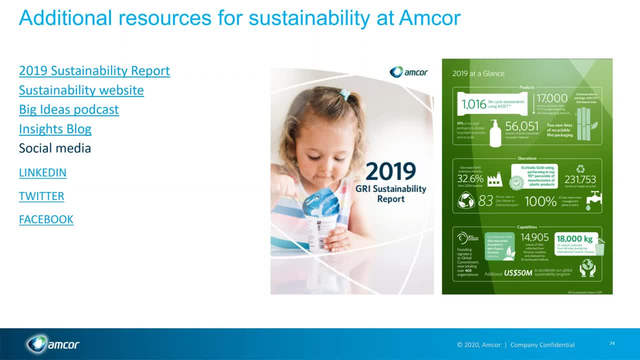 But you know, as much as we have a methodology and a structure within ISO to frame how you conduct studies, there is still a need to have a methodology to frame how you conduct studies. So that's an art around how you what do you define as the scope and what is the data quality that you're using and the comparisons that you're making and how you're characterizing. 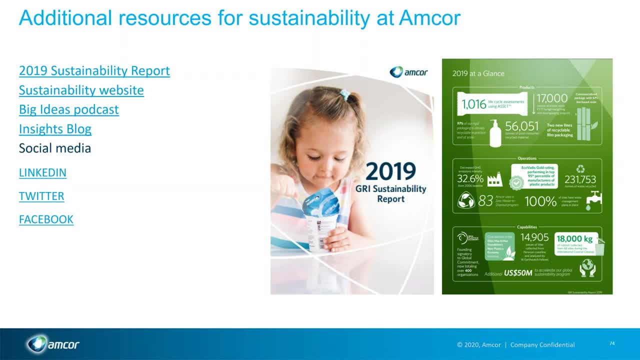 So that's why it's very important that you try to work with your suppliers and your customers, if you're doing an LCA, to get the best available primary data, Have really that informed decision about your specific product and its specific application. But then in some cases it's good to have a critical review of that study and just like 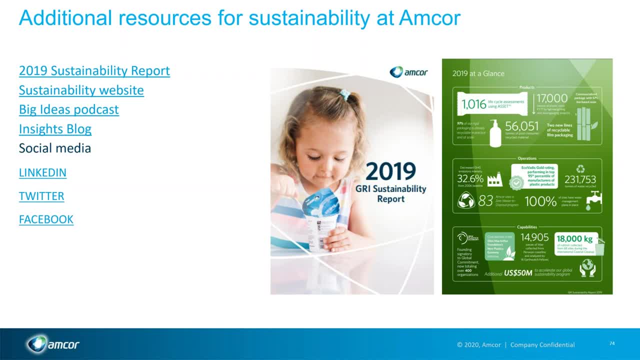 with the asset tool, that you have a third party that comes in and looks and assesses the credibility and the data and the scope and boundary conditions to make sure that you haven't overlooked anything and that the results are credible and that you can use those in a confident way for external communications or for also- you know- internal decision making here. 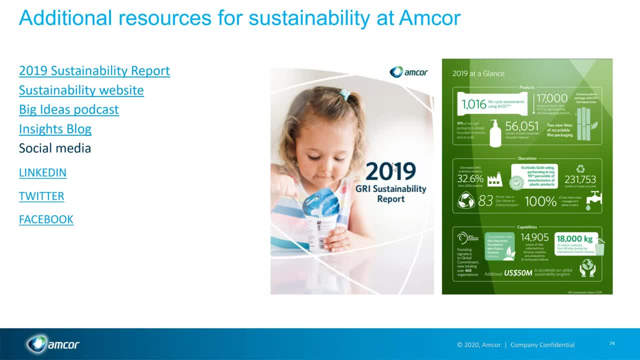 So I think all the tools are great. They can be very complex, Sometimes you need to have very an expertise in using those, But I think the key part is, as we've heard before, it's the quality of the data that goes in generating good data quality coming out and results. 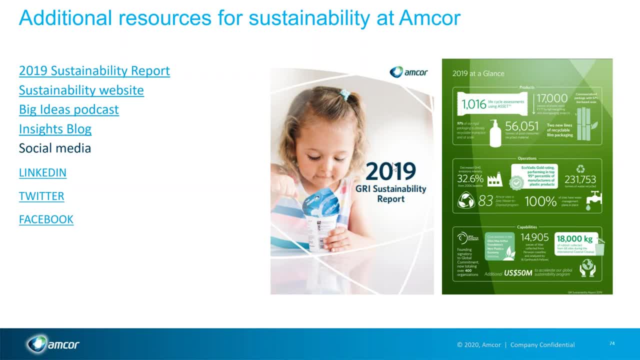 So I think that's the most important aspect is work with your suppliers, work with your customers to get the best data going into those software tools. I would agree 100%. That's typically would drive the differences. the data sets Okay great. 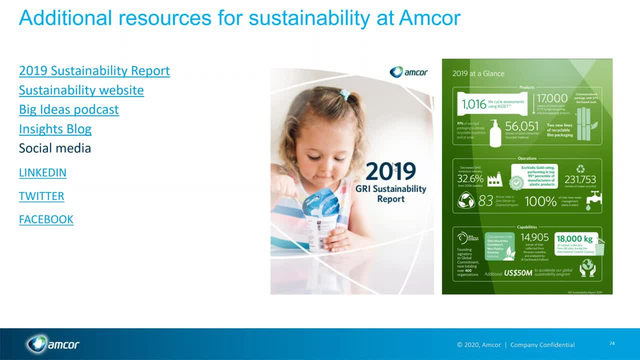 This question also was specifically addressed to both of you, so I'll just seesaw over to Dennis and let you start on this one. So here's the question and kind of a comment that goes along with it. So are you able to comment on the use of certified EPDs as a tool for your program? 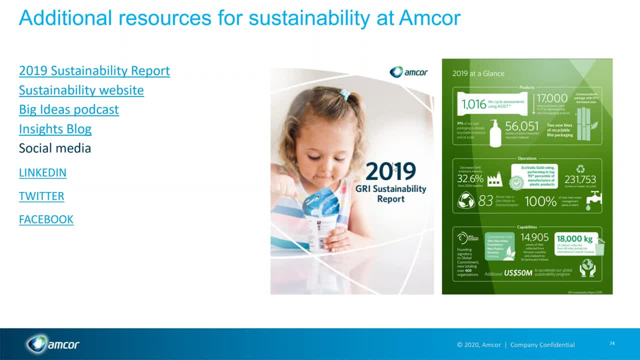 Most EPDs provide a litany of limitations for comparison purposes. I was going to say to repeat the question again, Asking commenting on the use. do you have a comment on the use of EPDs as a tool for your program? I really don't. 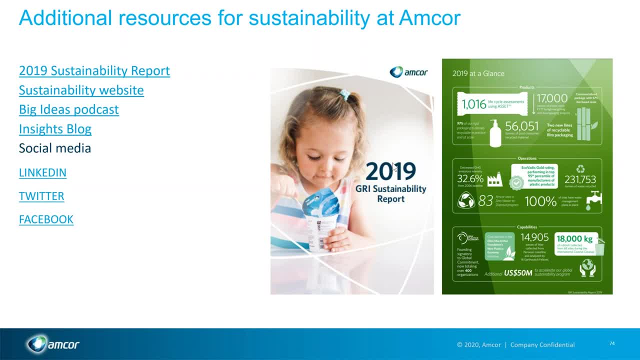 I think I'll let Bruce handle that one first. Okay, I think insomuch that EPDs are critical, they are the most important things for our program. They are very, very important for our business and our industry. EPDs are allowing you to assess environmental impacts of your product to 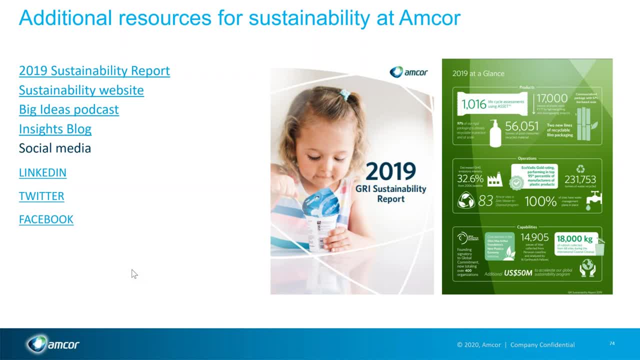 a defined, you know, functional unit. that's very beneficial. I think there could be some confusion out there that if you have an EPD it means the product is has like environmental benefits or is a preferred product. all you're doing is declaring and disclosing what those environmental impacts are could be high. 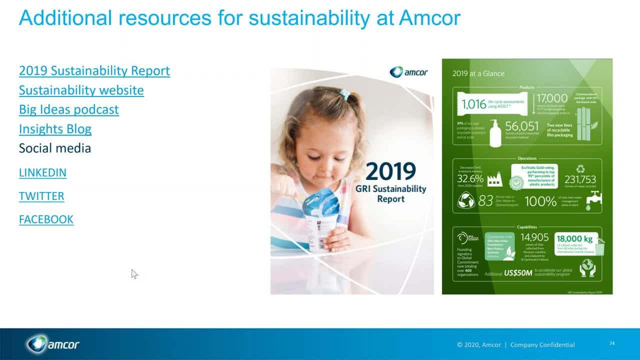 could be low, could be leading, could be trailing. so I think EPDs are good in that it allows you to take a lifecycle perspective at assessing your products in lieu of some other methods. but I think there is obviously limitations in comparability. there are a lot of efforts out there to alleviate some of those. 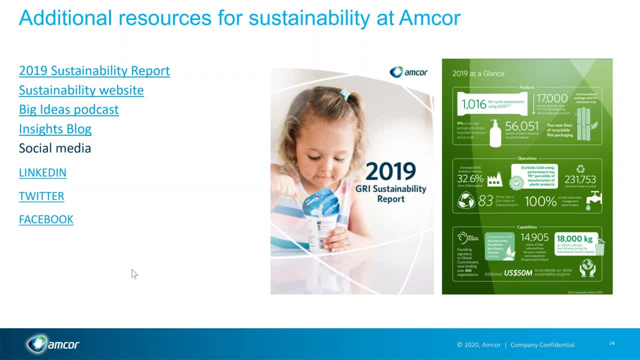 things I know in the building construction area. there's the ec3 tool that is allowing some capture of these certified data from EPDs, that are allowing the comparison of embodied carbon and they're giving sensitivity bands to account for some of this uncertainty and maybe comparability of these EPDs. so I 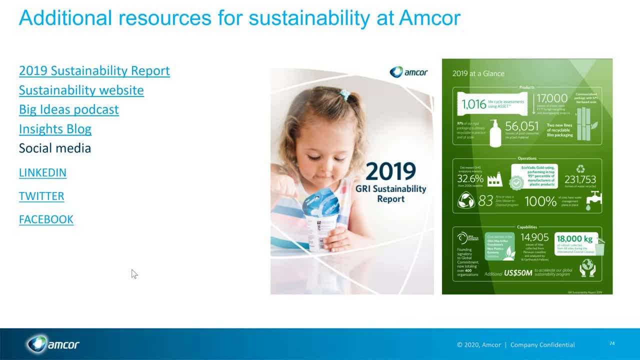 think there is a need for that. I think the method of communicating EPDs in the way they are can be confusing because it's a lot of data, like six or seven, eight pages of a lot of numbers and, as Dennis had said before, you know you need. 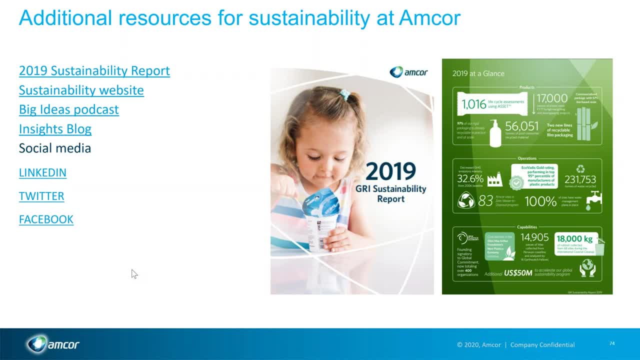 to fulfill LCA through not only scoping it correctly, measuring it better, but it's also the communication. if it's confusing, confusing and overwhelming, the stakeholders and people who need to understand that aren't going to understand the value and capture the value out of the LCA. so, just like you can, 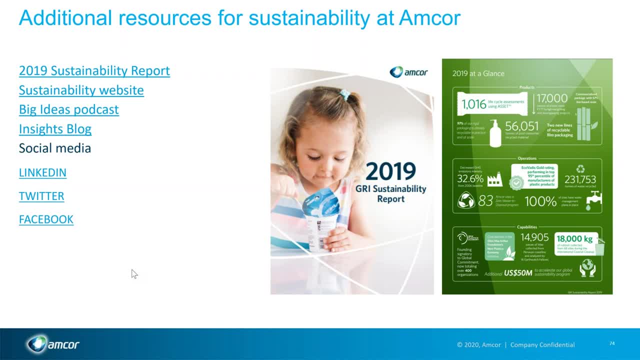 use environmental equivalencies from that EP EPA calculator. I think the challenge is that we need to distill the information down while still being transparent on some of the limitations of the value of what this study was measuring. what did we learn? how can you use that information? 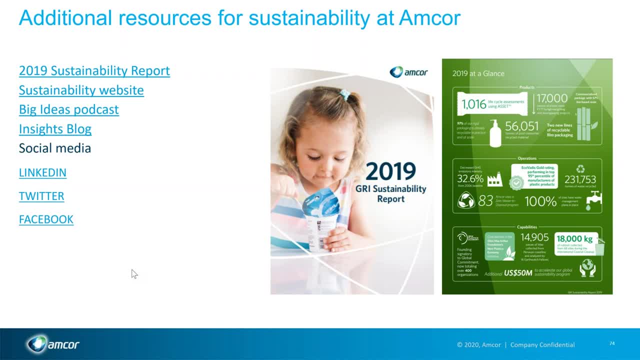 really to the non-LCA practitioner right. We don't want to communicate results. In some cases we do, but we need to distill it down and that's the challenge of LCAs. How do you take that rigor of a 40-page report? 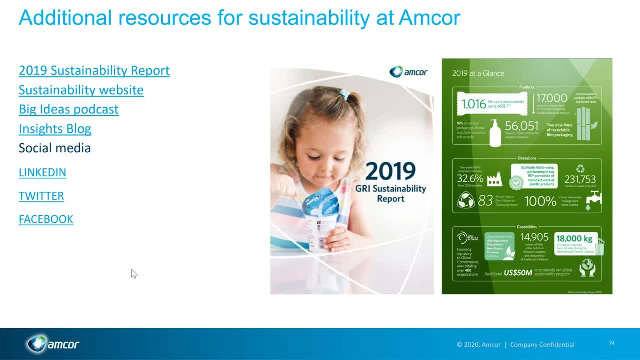 and get it down into that elevator speech, that one pager. that makes it important. So EPDs have their value. They also have their limitations. BASF does have EPDs for a lot of our products because it serves the market need for our customers. 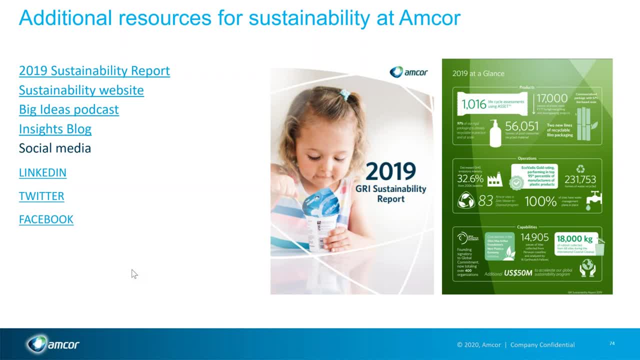 but we also understand where those limitations and benefits are. Yeah, the hesitation part of my response is we typically don't really participate for the end result We contribute. I have a great slide that explains this. but packaging is just one portion of our customers' carbon footprint. 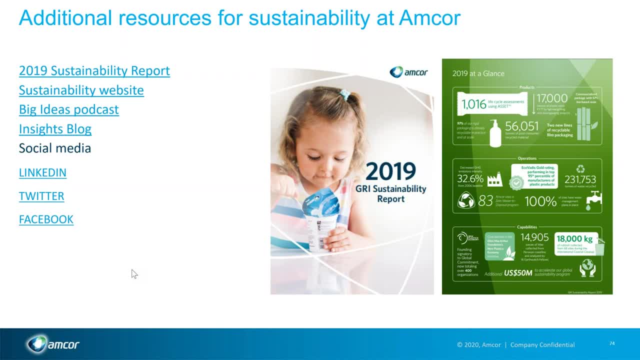 So we're taking into account a bottle where you also have to take into account the product, the label, the cap, and then maybe even broader than that, if there's agricultural inputs into it for feeding beef that you may package in a flexible package. 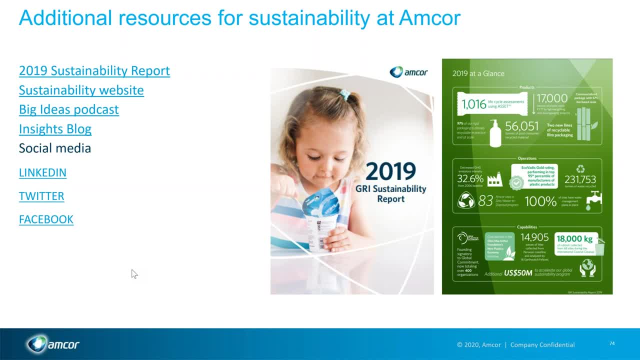 So typically our customer wants a larger scope when they go to this stage and we only contribute the packaging part of it and we really don't see a lot of activity just for that part of the scope. So it's not something we participate in considerably. 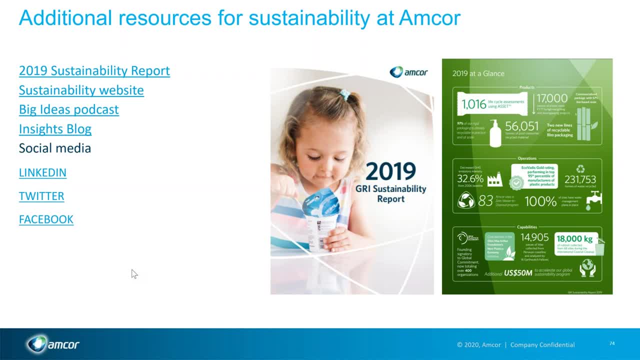 Sure, That makes sense. So we've reached 1226, and I have just a couple of closing comments. But before I do that, I just want to give both of you, and I'll start with Bruce and then go to Dennis. 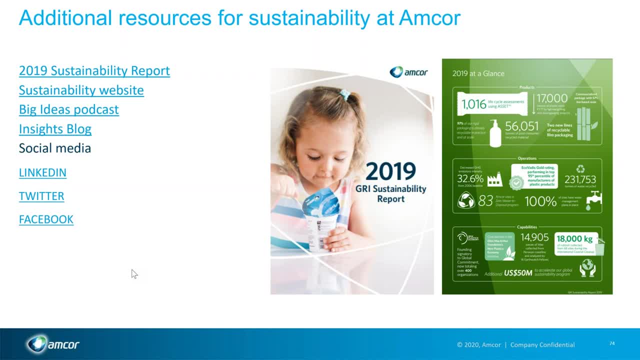 just 30 seconds on. if you have anything that you any other comments you'd like to make, or any closing thoughts, or one thing that you'd like for folks to walk away with today, to wrap us up here, Yeah, I would just say to the audience: 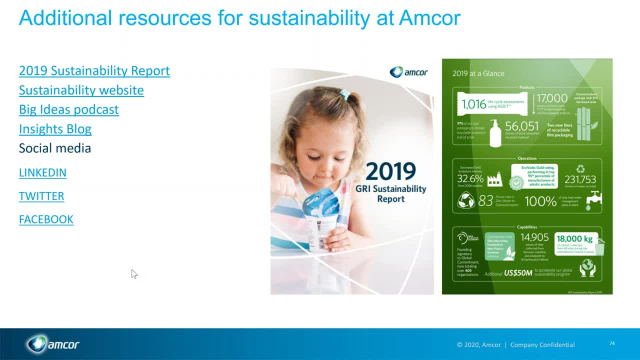 that we all want to drive greater sustainability and make improvements into our environmental footprint that we're leaving and really lifecycle thinking, lifecycle assessment, of being able to look outside the boundaries of our own companies or even our own lives Really and understanding the broader impacts. 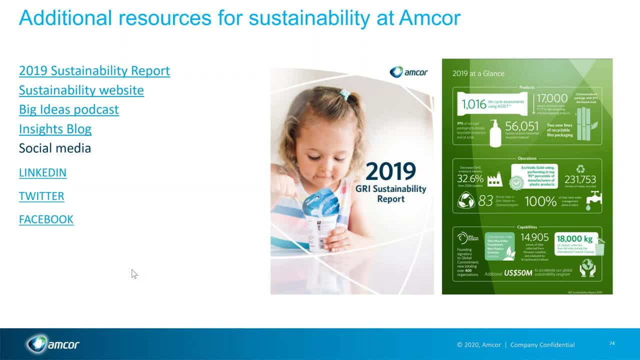 and benefits that our actions are having is very critical for us to meet these challenges that we see coming down the road. So lifecycle assessment has a great power behind it in being able to quantify in a very credible and comprehensive way these impacts, but also understanding benefits and trade-offs. 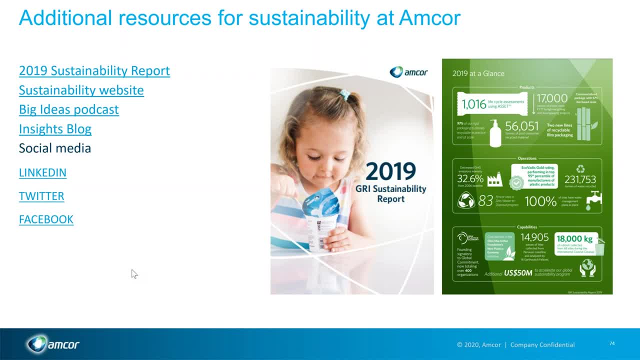 And I think it should be, if it's too complex. start with lifecycle thinking and then build upon that, Because I think having this holistic perspective is really important for us to really communicate effectively the benefits that our companies are enabling out there in our value chains. 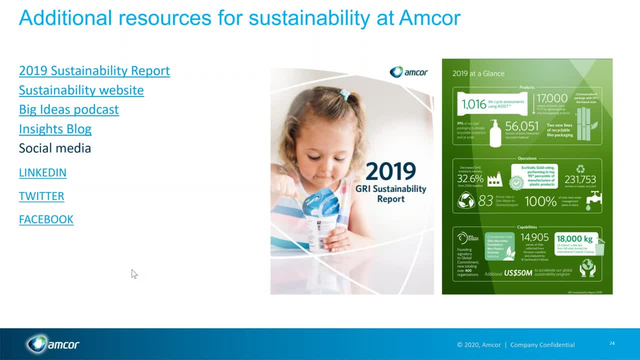 and really supporting our customers and the downstream consumers and helping them have products that are out there that are more sustainable and reducing environmental impacts, adding social benefits, reducing costs overall. So LCA is a powerful tool and we should be trying to implement that more. 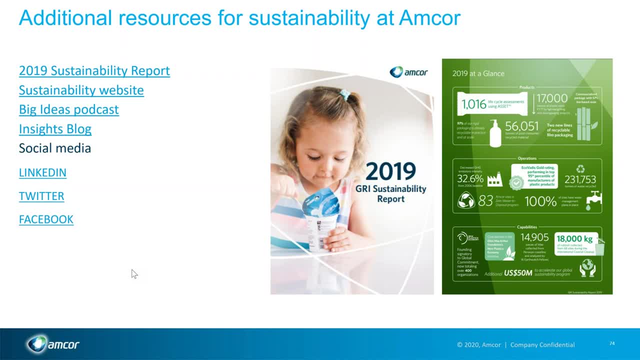 within our organizations to really help us innovate better but also engage with our customers in a more sustainable way. Excellent, Dennis, I'll offer you the same opportunity. Yes, a very similar answer. LCAs give you a perspective and a viewpoint that's really as holistic. 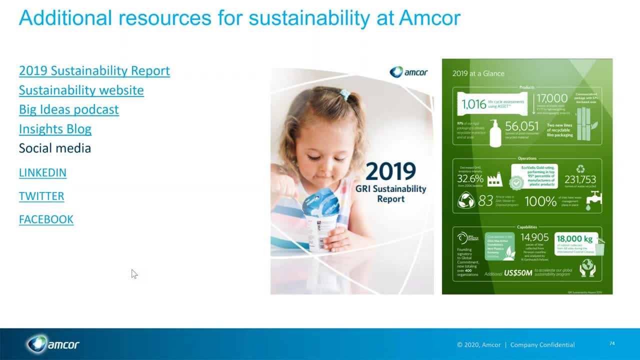 We often do talk about the big topics in the news of plastic waste And we've seen in cases where we observe a shift in the national demand for materials, whether they be paper, especially in the bag. the bag area is a big one. 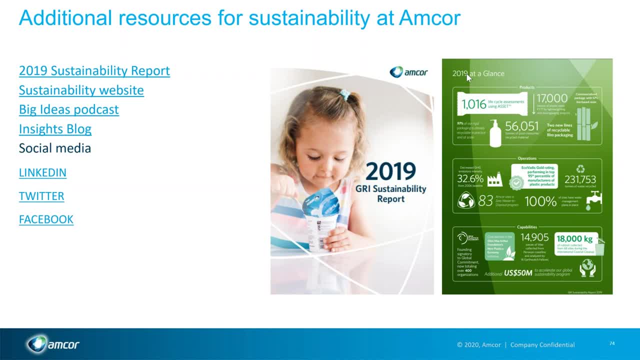 Just because we want to address one aspect. what else do we impact? And we see the wrong decisions for greenhouse gas impacts being made with a reaction to an event or reaction to something in the news, And the LCA really does bring it into perspective. 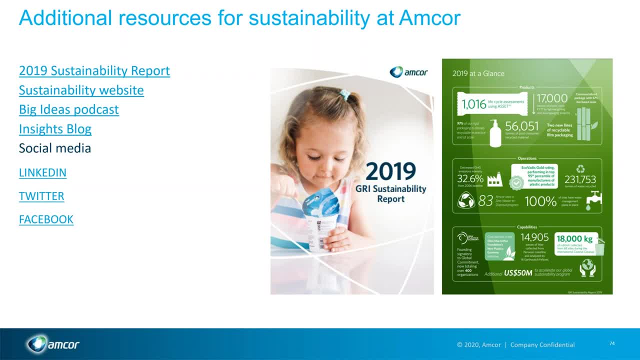 It's a holistic viewpoint And even if you don't participate in an LCA, understanding the process brings just more to your portfolio of understanding on how to make decisions You're taking and encompassing the entire picture through the end life and how the end life can come back as PCR or reusable materials. 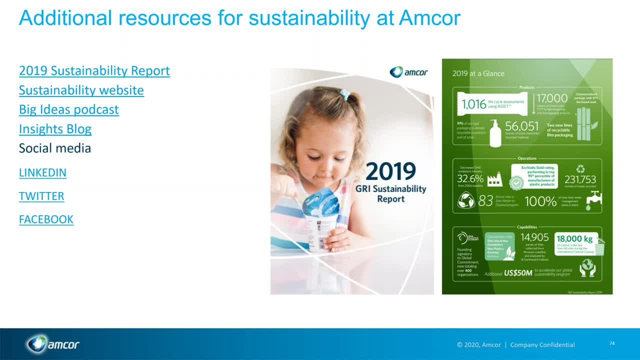 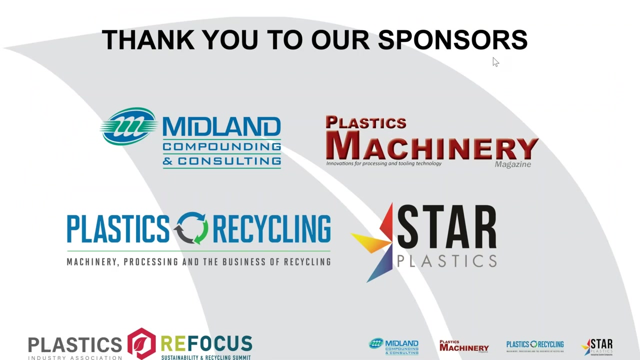 What does that really mean for the overall picture? So it truly gives you a broader understanding of decision making for packaging in my world or any product that we're manufacturing. LCAs are a powerful tool for that. Excellent, So I'm just going to have a couple of closing comments and I'll hop back on the webcam for everybody for just a second so that you can see the sincerity in my eyes. 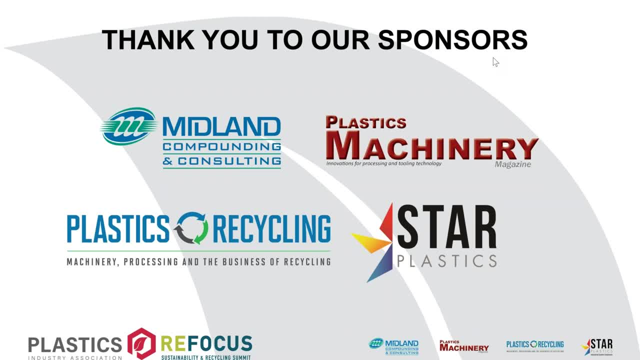 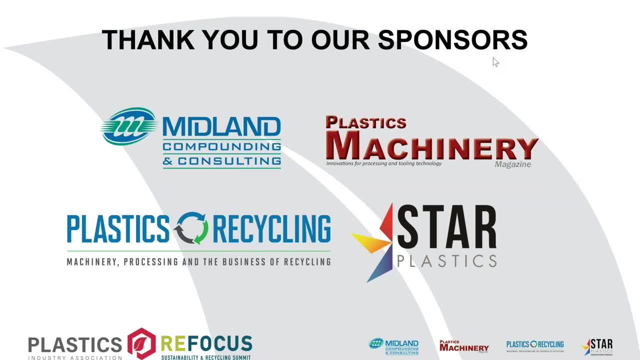 So I want to thank them again. I want to also thank our sponsors again for bringing this content Again: Midland Compounding and Consulting, Plastics Machinery Magazine, Plastics Recycling Magazine and Star Plastics um. we are able to do this because of them. we hold ourselves to the highest standard and we try to. 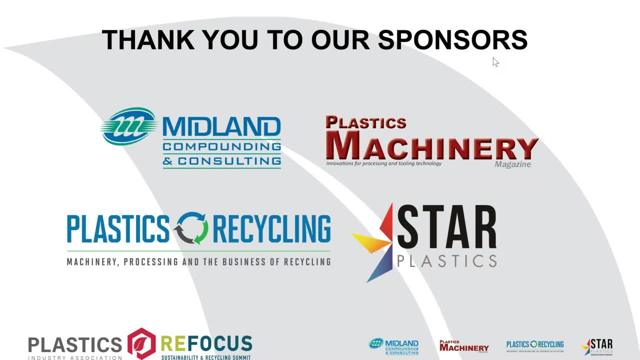 bring you the same exact high level of content through these virtual webinars that we would have brought you um to, you know, to cincinnati, had we been able to meet in person. so, um, thanks for everybody for joining us. i apologize, i did not get to all the questions. you guys had a lot of great. 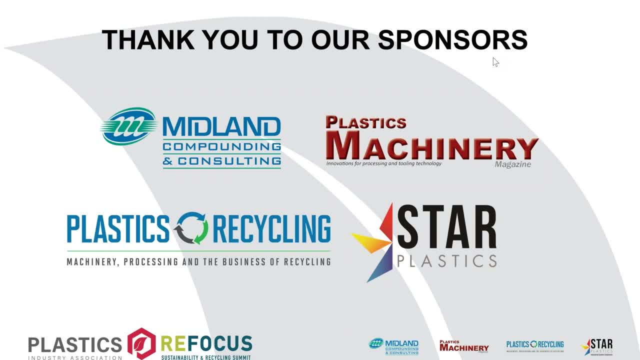 questions today. um. so please know that i will pull that list of questions at the end of this session and i will make sure that our speakers get a copy of that um so they can reach out to you with those answers directly if they wish, or vice versa, if you don't have their contact information. 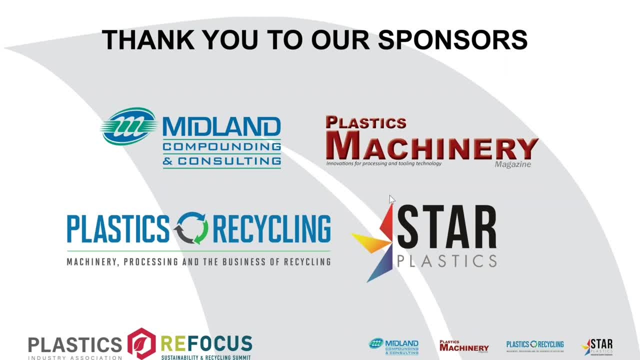 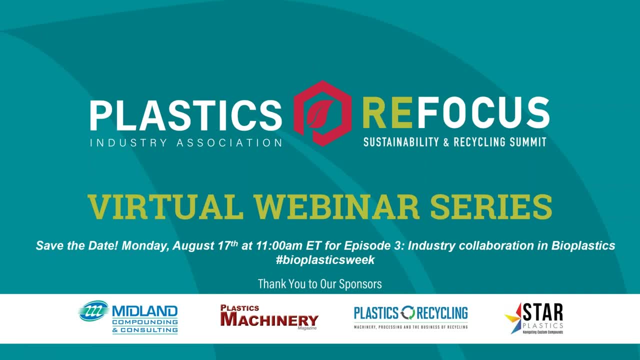 and would like to be put in touch with them. please let me know and i'm happy to to help make that happen and just as we wrap up. um, you know i said this monthly. this webinar is going to be a little bit longer than what we had planned for the webinar, but i want to. 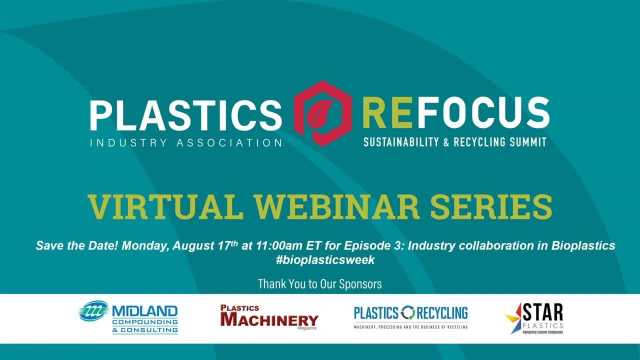 make sure that everybody knows that this webinar series was going to be monthly, but everybody needs a little summer break, right? so, um, we are going to offer a july- uh- break from the refocus webinar series. um, and we will be back in august, so we already have our date where we will resume with. 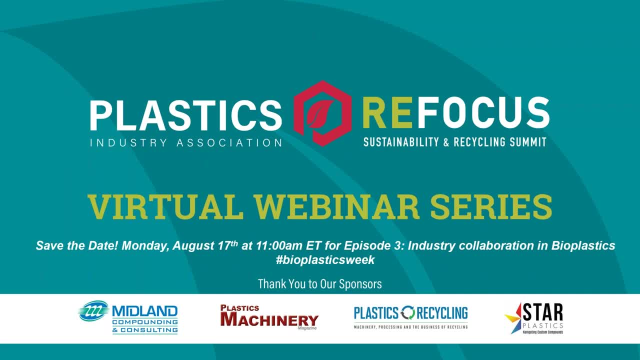 episode three on monday, august 17th, with an episode titled industry collaboration in bioplastics. and this is especially placed on a monday um in that time slot because it's kicking off bioplastics week, so that's a plastics industry association um event. that is a celebration and 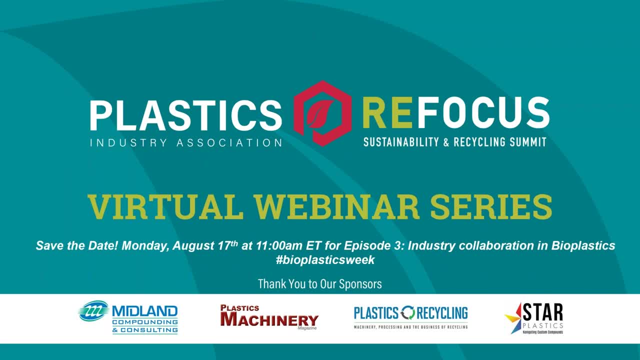 week-long education on bioplastics and largely um that takes place on social media, so, using the hashtag bioplastics week um, follow along with what's going on there. there'll be various ways to engage, but it starts with the webinar on monday, where you can learn more about bioplastics. we'll 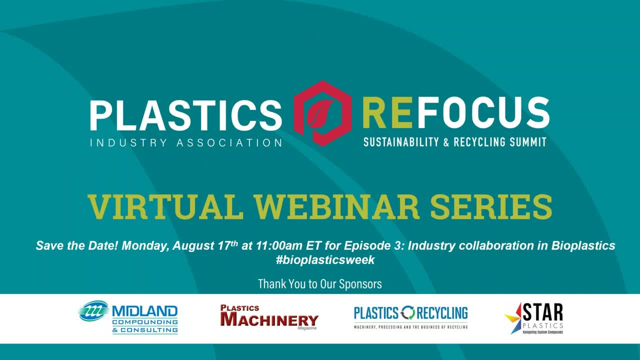 start with our bioplastics division directories, and then we'll be back in august and we'll be talking about what's going on in the field for bioplastics in the future as well, and then we'll be talking about bioplastics 101, and then peace, and peace is going to be ourselves, and we'll be.